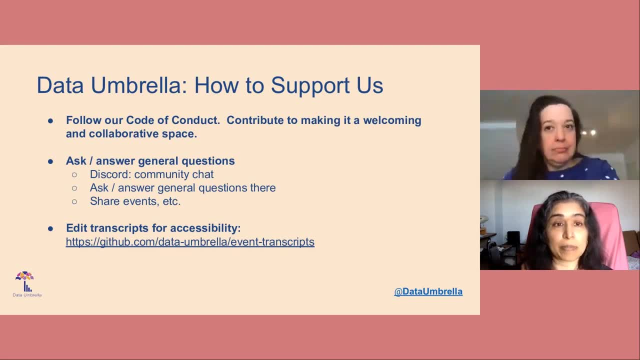 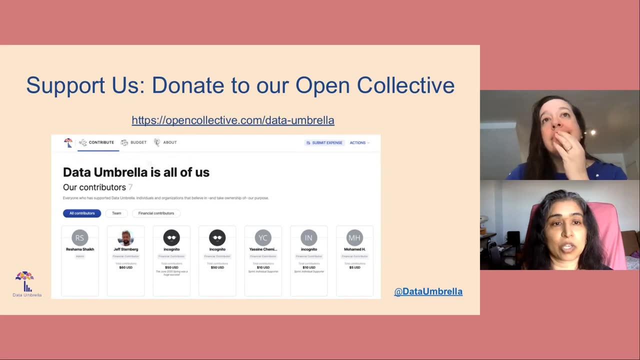 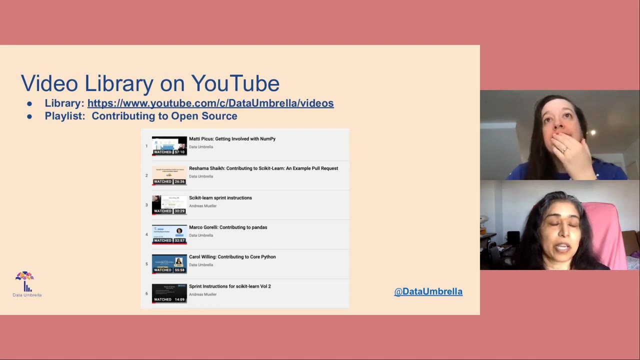 The link to the Discord is on our website. Next, we have an open collective if you want to donate something to support us operationally. This is being recorded and the video will be placed on YouTube, and all of our webinars are on YouTube. 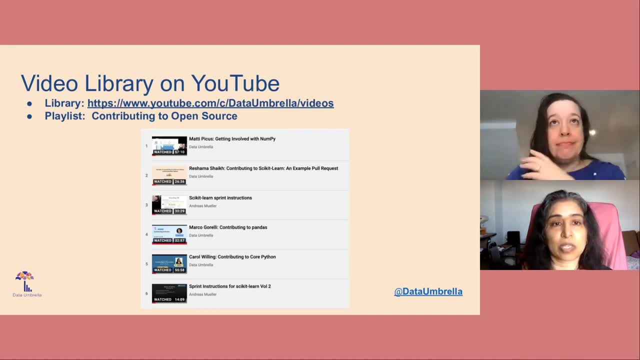 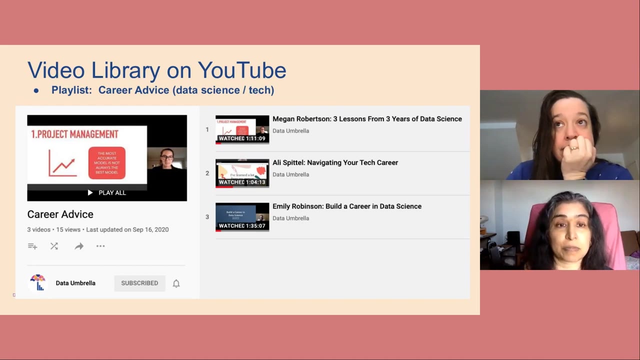 We have a few playlists. The first is contributing to open source, And so, if you're interested in contributing, there's some great videos that have been just done pretty much in the last six months. If you're looking for career advice in data science or tech, we've had three great speakers. 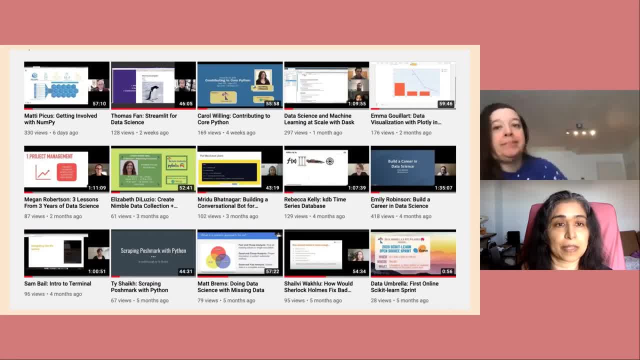 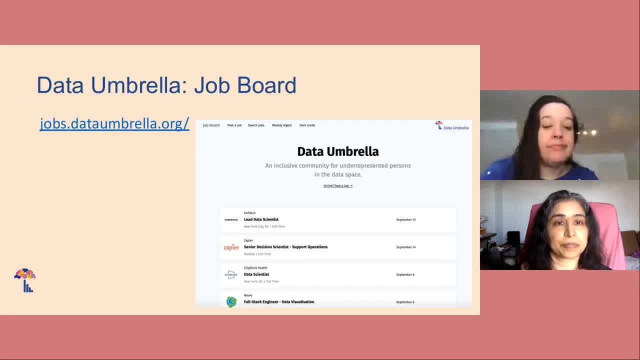 on that, And so we have a playlist as well, And this is just a sampling of some of the webinars that we have done in the past year. We also have a job board, So if your company is hiring, feel free to share job postings. 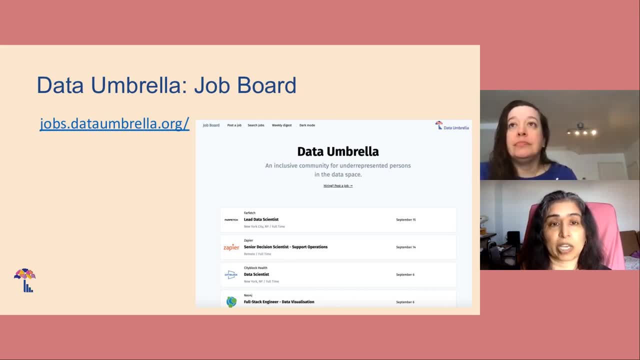 And if you're looking for jobs, check out our job board. Our website has a lot of information. So if you're interested in contributing to open source, there's a link in the description. So if you're interested in contributing to open source, there's a link in the description. 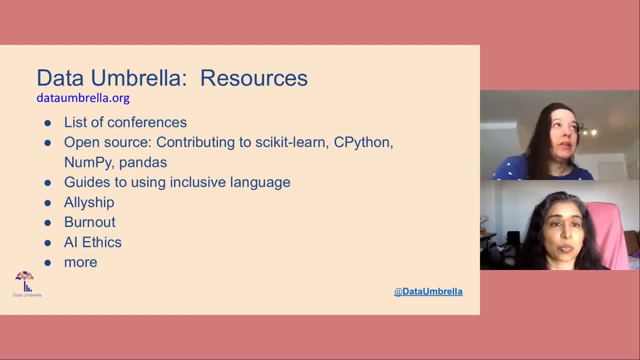 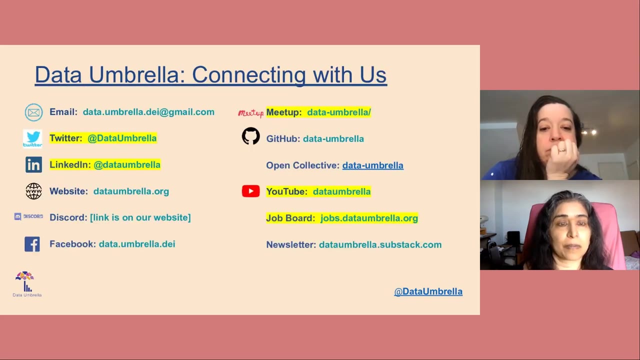 We also have a lot of resources. We have a list of conferences, We have guides to using inclusive language and how to appropriately collect demographic information, tips and articles about allyship burnout, AI ethics- So feel free to check that out. 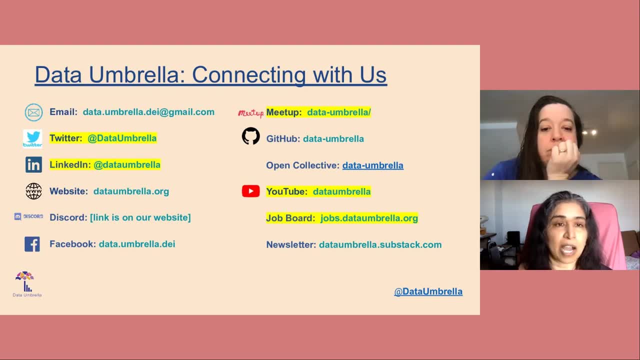 We're on all social media platforms. there's Data Umbrella. The ones I've highlighted are the ones that, if you can pick, the one that everybody has their preference for what they prefer to use is the place where all of our events are shared, so that's probably one place to join. 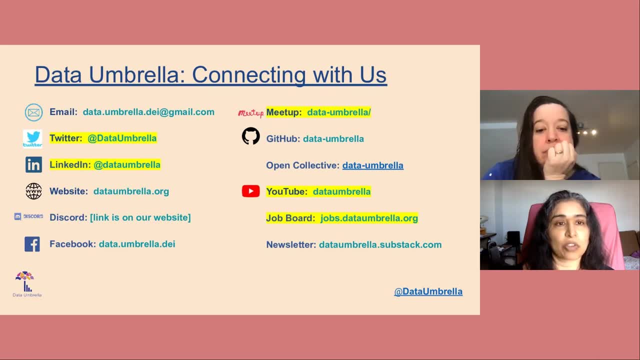 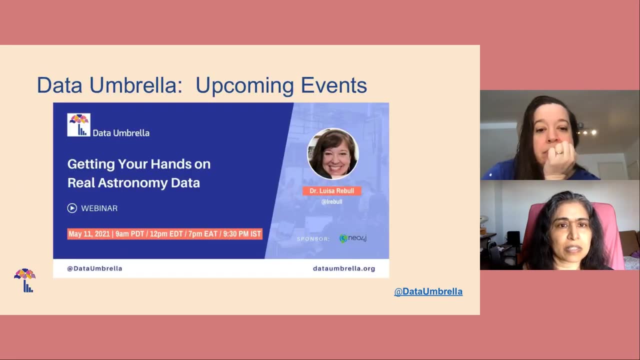 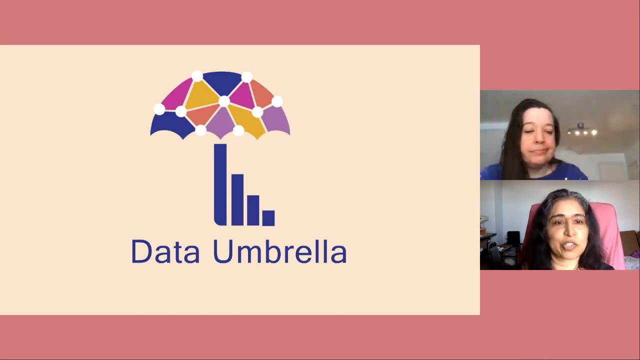 Our videos are uploaded on YouTube and we are also pretty active on Twitter and LinkedIn. Oops, did it not change? Okay, it went to the wrong thing. It didn't upload the right thing. I'm just going to go to my other thing. Today's speaker is Louisa Riebel. Louisa is 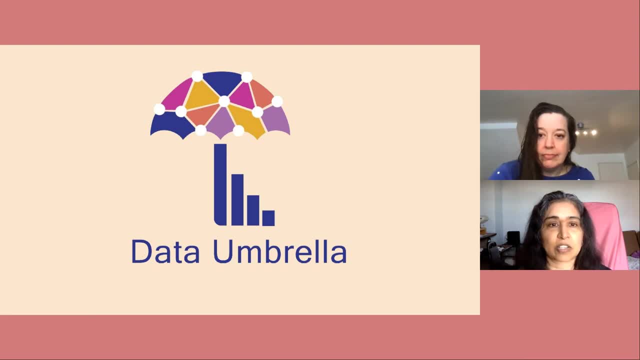 a research astronomer at NASA IPAC Infrared Science Archive at Caltech. Louisa has always wanted to be an astronomer, ever since she was very little. She got her undergraduate degree in physics from the College of William and Mary in Virginia and her graduate degrees 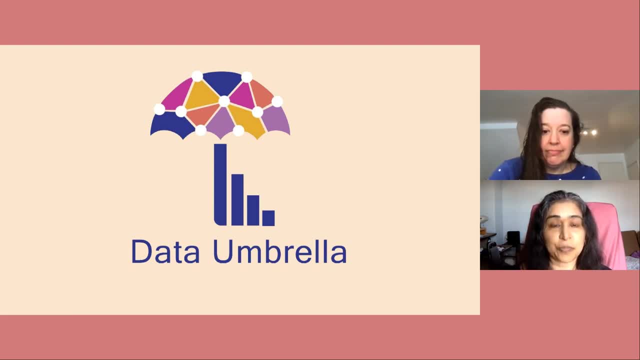 in astronomy and astrophysics from the University of Chicago. She's been on the science staff at IPAC since 2002, and her research focuses on the formation of young low-mass stars all over our galaxy: stars 1,, 2,, 3,, 4,, 5,, 6,, 7,, 8,, 9,, 10,, 11,, 12,, 13,, 14,, 14,, 15,, 16,, 17,, 18,. 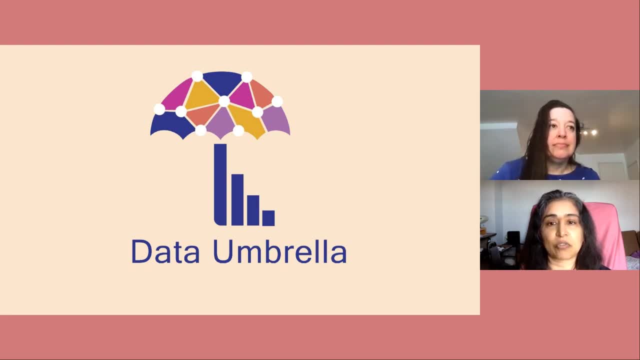 and 19, 20 years old Now. she has two grand �сти. She's 80-plus, I imagine she's already one to 50 million years old. Lisa is on Twitter as l-re-b-u-l-o. With that, I'm going to put myself on mute and I will hand it over. 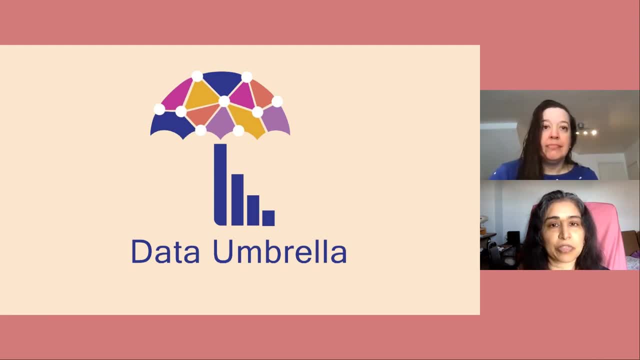 to Louisa. If you have any questions, feel free to post them either on chat or Q&A, and when there's a good time to sort of interrupt, we'll get those questions answered, Louisa. thank you so much. You're welcome, Rachael. 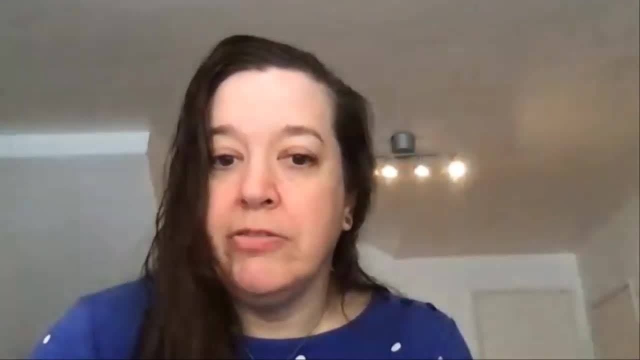 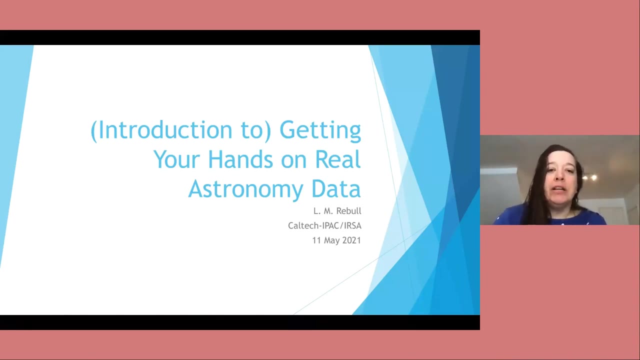 Okay, excellent. Well, thank you very much for inviting me to talk to you guys today, to all of y'all from all over the world, which is so exciting. My internet has been a little squidgy, So if things are getting weird, please let me know. I can turn off the camera and see if that speeds things up. 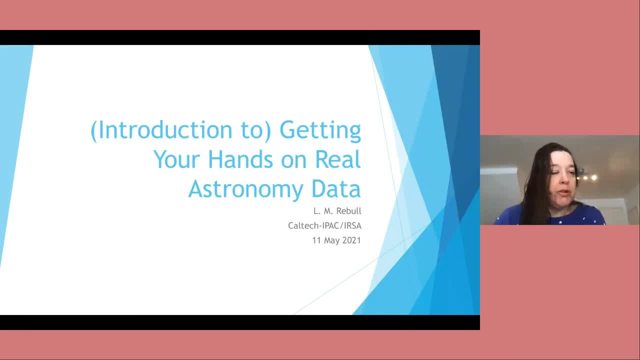 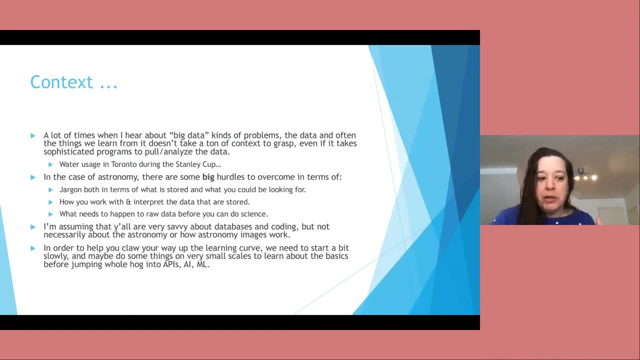 But hopefully it will all be fine because I rebooted the router this morning. Okay, so just in terms of the context of where I'm coming from. So a lot of the times when big data problems make it into the media, the data and the things that we learn from it, you don't need to have a lot of background knowledge or context to grasp. 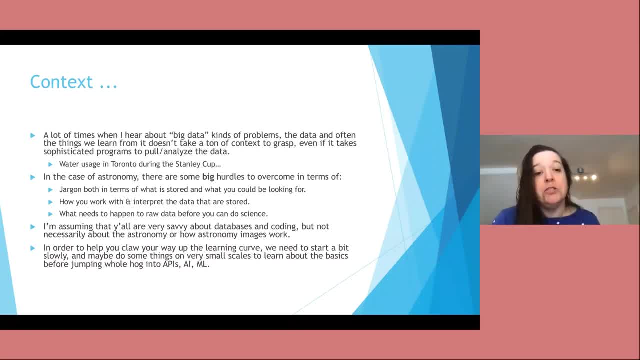 So the example that I have there is water usage in Toronto during the Stanley Cup. Now, probably that's enough information for you to start putting together what's happened there, right? So they studied the rate at which people were flushing toilets in Toronto during a big hockey game. Okay, And since in Toronto there's so many fans of hockey, you can see the water usage spike when there were lulls in the game. 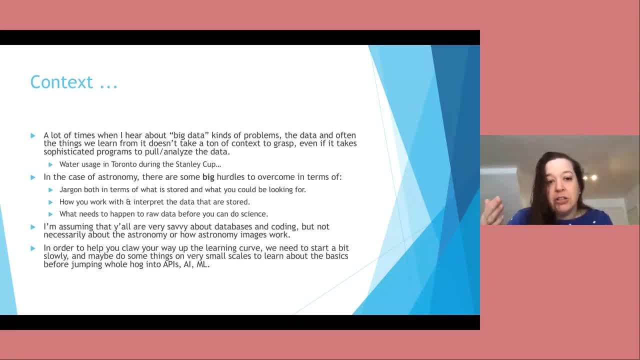 So you know you don't need a lot of context, or even you know deep understanding of the units that they were working, because it was probably gallons per second or liters per second, something along those lines. And so, even if the programs that were used to analyze those data are sophisticated, 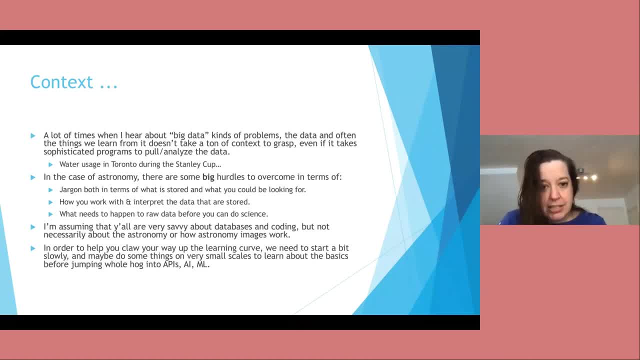 Both the problem and the context is easily understood without a lot of background information, But astronomy is very, very different than that. There's some really big hurdles that you know the average person on the street needs to overcome- In terms of jargon, you know, in terms of the astronomy concepts, but also in terms of what data are stored and what you could be looking for in those data and how you work with those data and how to interpret those data that are stored. 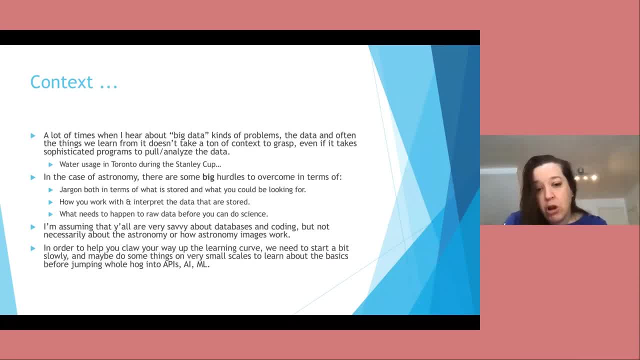 That's also not as interesting. Okay, and, as you were saying, other questions. However, the first question I want to ask you about astronomy- and I want to take a couple minutes to get through it- is whyudi not trivial and what needs to happen to raw data before you can do science. so i'm assuming that 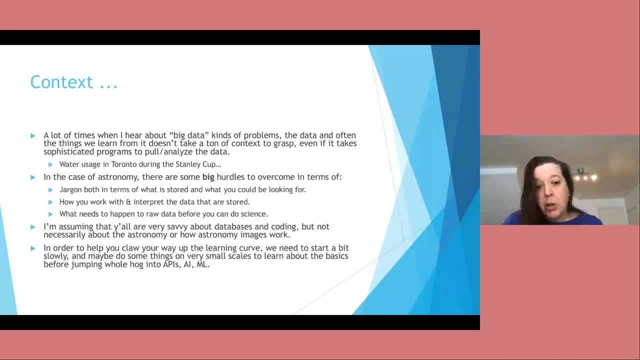 y'all are pretty savvy about the databases and the coding, but i'm going to start at the beginning. when it comes to the astronomy and astronomy images and in order to help get you there, we're going to have to start a bit slow and i recommend that you don't start jumping whole hog into python. 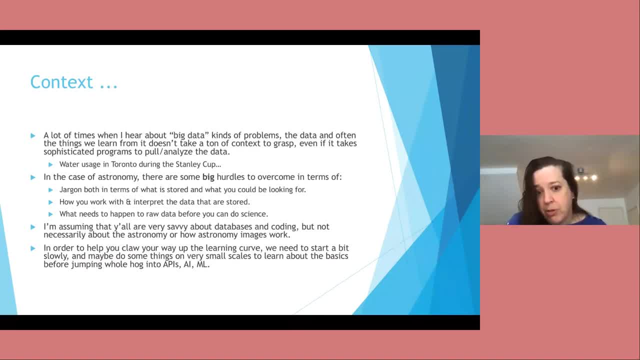 apis, or artificial intelligence and machine learning. i mean i'll be referencing those um throughout the talk, but i would recommend that you start slowly so that you learn about the basics of these data before you jump into the deep end. i am totally serious about this because even professional astronomers misuse these data all the time, and i've got specific examples. 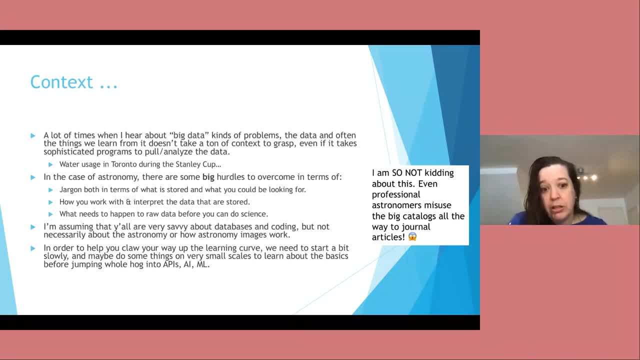 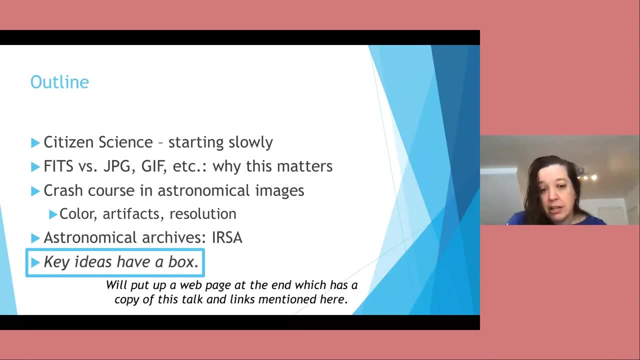 of it later in the talk. so i'm totally not kidding that you need to start small and don't start by pulling tens of thousands of sources and expecting that the science is just going to fall out. so i'm going to talk a little bit about citizen science and how to start. 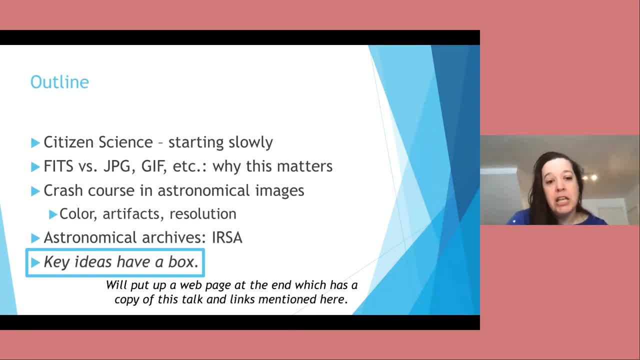 that you know, just to learn the basics, and then i'll have a whole bunch of concepts on things you need to know before you can work with astronomy data. so we'll talk about different file formats and why it matters and what things you need to worry about when dealing with astronomical images. 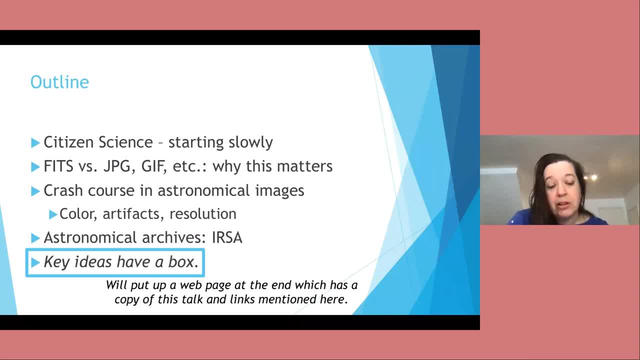 and then i'll give- i'll have some actual examples of ursa, the infrared astronomy- sorry, the infrared science archive, which is where i work. um, i'll give you lots of examples of that and then the really important ideas. i've put a box around and i made. there's lots of references. 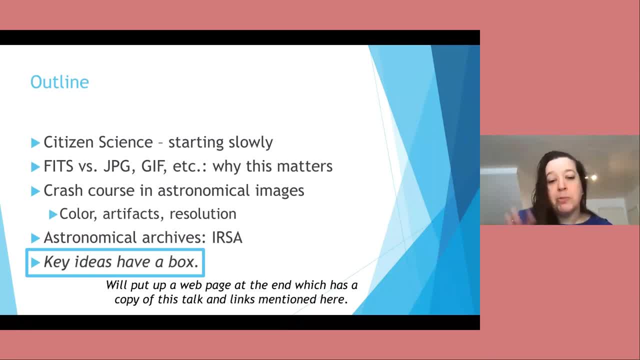 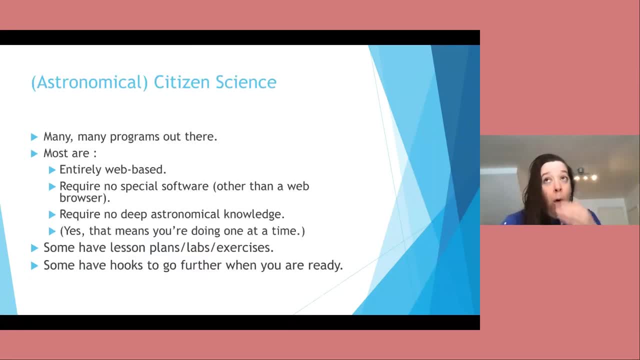 in this talk uh to other websites and other resources, and so i'll put up a web page at the end which collects not just a pdf copy of these slides but also all the links that i'm going to mention here. so there's lots of astronomy, citizen science programs. 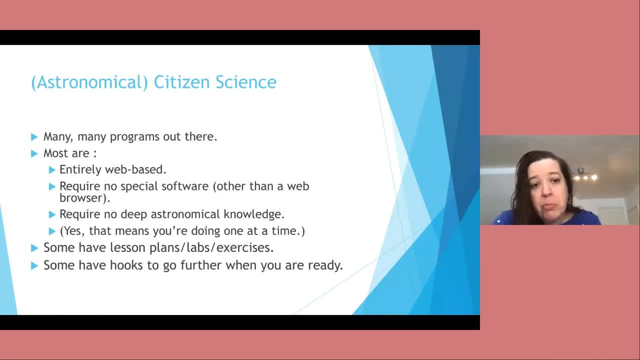 in fact, some of the very first citizen science programs were astronomy. so there are many, many out there, and most of them are entirely web-based. you don't need any special software, you just need the web browser and an internet connection, and you don't need any deep astronomical knowledge. 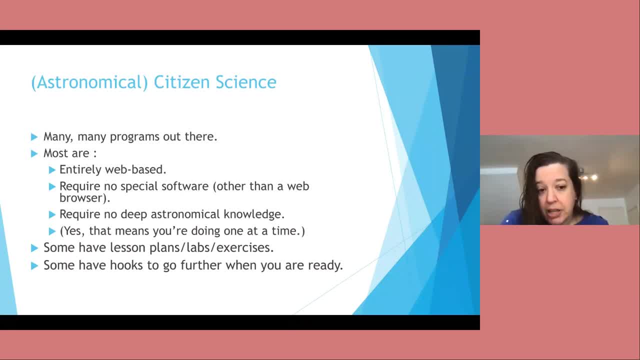 but yeah, that does mean you're doing one object at a time and i realize that that seems slow for those of you who are used to pulling, you know, huge amounts of data at once, but that at least starts to give you a sense of what they're looking for. uh, some have lesson plans or labs or exercises. 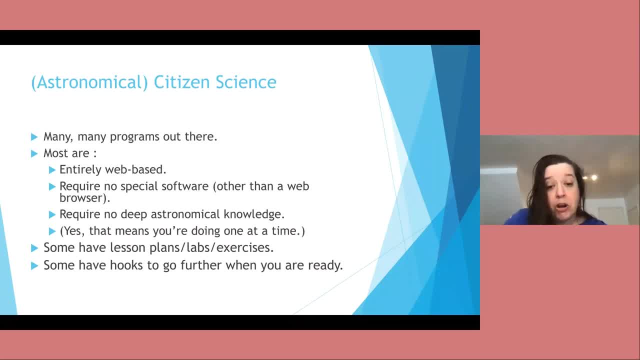 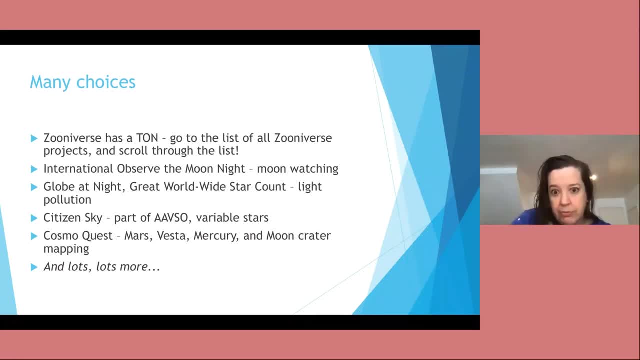 that you can do, and some have hooks to go further, when you are ready to start pulling tens of those together on the internet. so that's really important as well. so i'll let you go through the slides and then i'll give you a few more of my own personal thoughts on the moon and the moon. 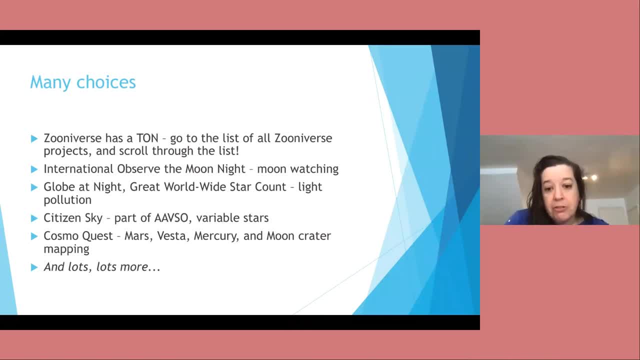 in general. good evening everyone. thank you so much for joining me today. this is a special session of the zooniverse and i'm going to be discussing some of the most important questions, or the most important questions that are asked by our listeners today. one of the things that i wanted to talk about today is the impact of the moon and the sun. 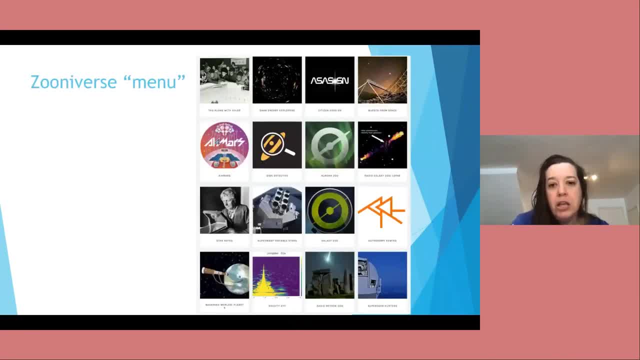 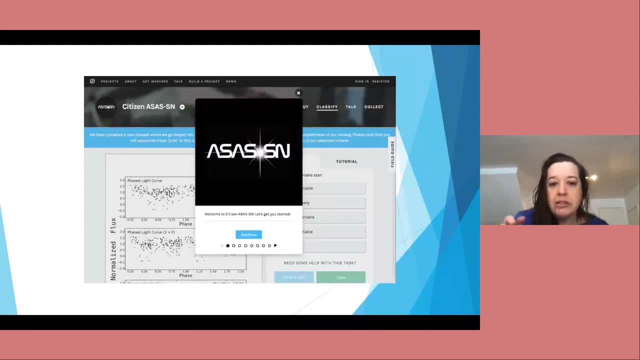 in our solar system. the moon is completely interconnected from the earth and the sun is just there's a ton more so this is just like the astronomy's universe menu, and you know there's there's so many projects. it's really amazing, and whenever you start one of them, it always starts. 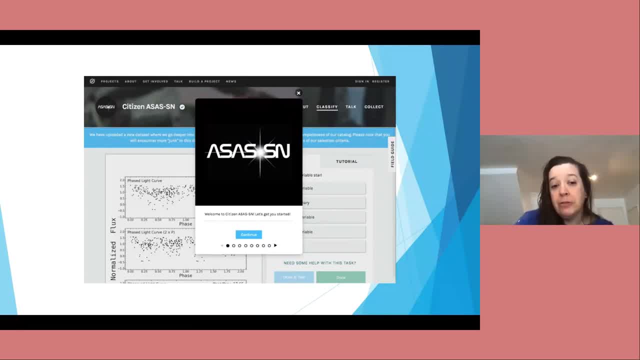 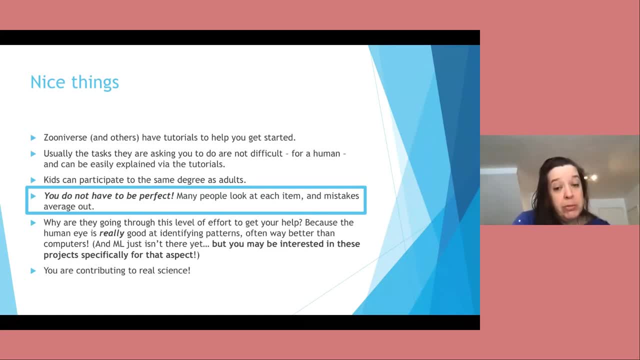 with the tutorial to show you this is what we're looking for and this is how to get started on this project. so the tasks they're asking to you to do are not difficult for a human, but may be very difficult for a computer, and so the tutorials are designed to explain specifically what they're. 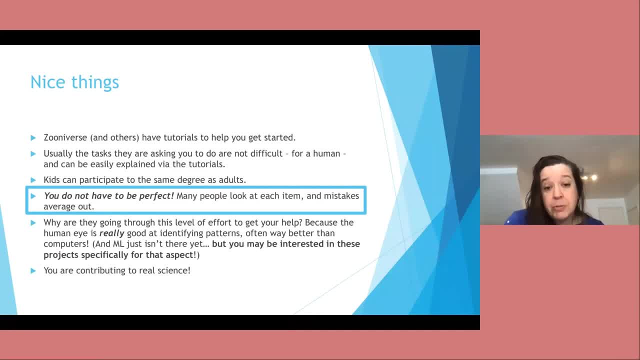 looking for. the nice thing about these projects is that kids can participate to the same degree as adults. you don't need lots of programming experience, you just need the web browser, and the whole reason it works is that you know you don't have to be perfect. many people look at. 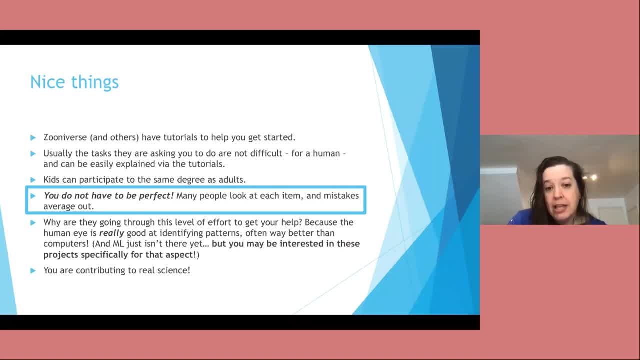 each item, and so the mistakes average out. now that's important for all of you guys who are thinking in terms of, you know, big projects and pulling tens of thousands of sources. the reason that this, the, that these kinds of citizen science projects work is that everyone is acting as a check on each other, and so that's. 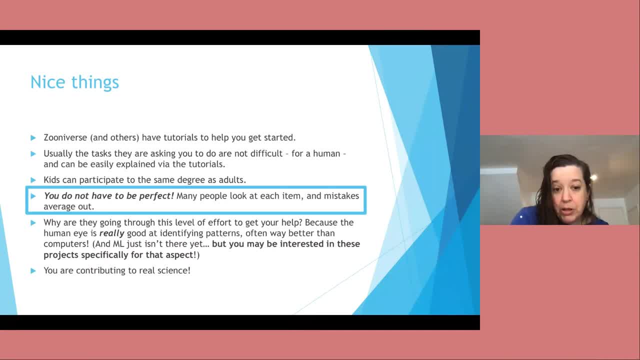 how you get rid of the mistakes. but why are these projects going through this level of effort to get help from citizen scientists? because the human eye is really good at identifying patterns and machine learning just isn't there yet. but especially if you're an expert on machine, 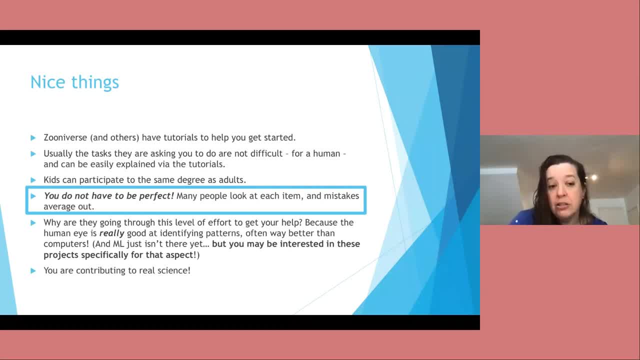 learning. i would. i would say, go and look at these projects, maybe not because you're interested in what kind of problems they're trying to solve, what kinds of problems that they need human eyes to do, because that is also, then, the horizon that you should be aiming for with machine learning stuff. 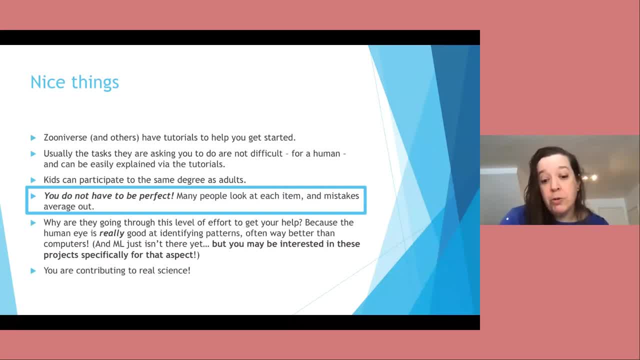 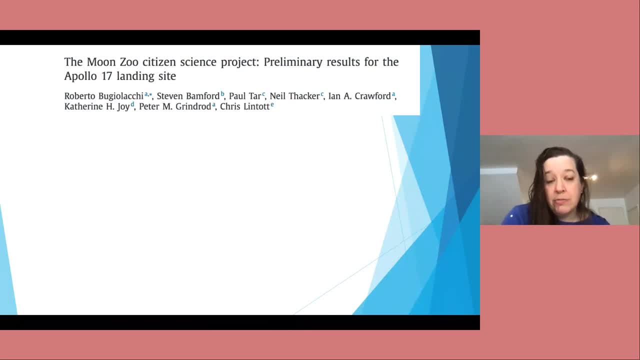 and for these projects you are really contributing to real science. there's, um, you know, lots of journal articles that have come out. this one has to do with looking at uh stuff on the moon. this one is looking for uh planets from some kepler data and this one is looking for 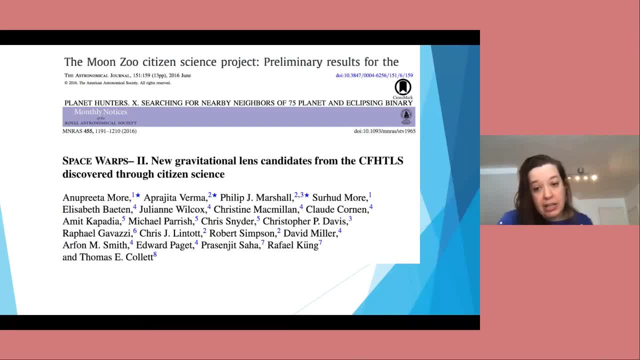 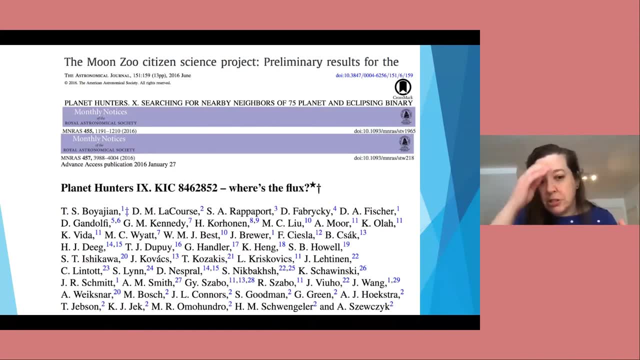 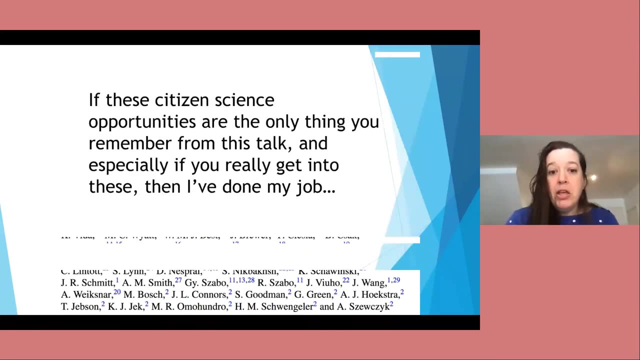 gravitational lens candidates, basically looking for galaxies, um, and this one has a- is a very interesting star that was discovered by citizen scientists. it's a very confusing star, where it's not at all obvious what's going on with this star. so, if you, if the only thing you remember from this, 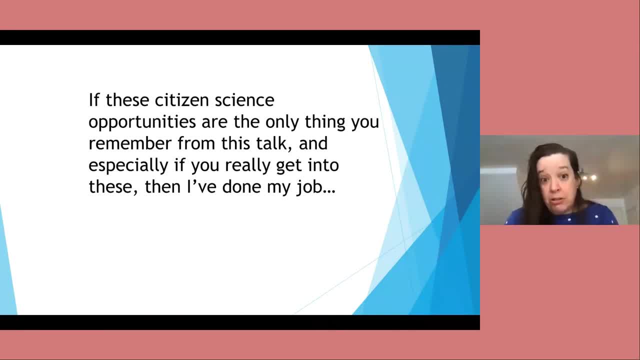 talk is that there are these citizen science projects, and especially if you really get into at least one of them, then i think that i've done my job. it's all good, but maybe that's a little bit more complicated than what you're saying, but i think that's a little bit more. 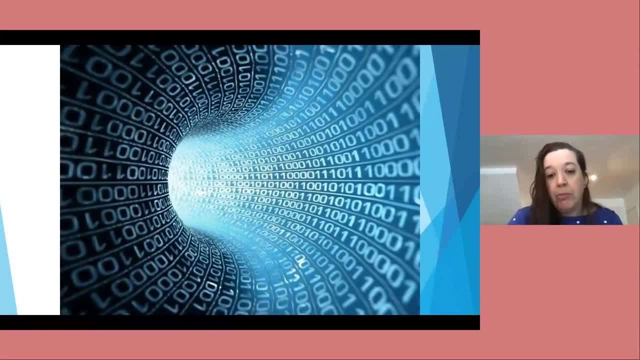 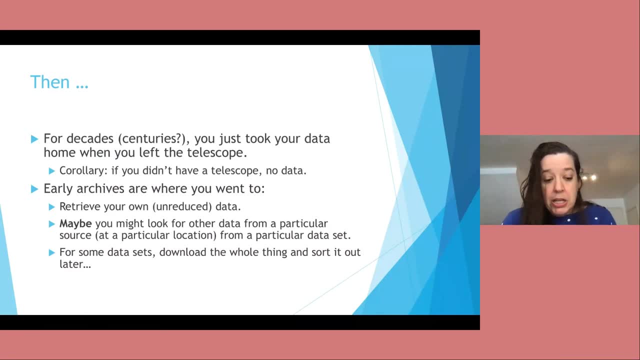 difficult than what you're saying, but maybe that's a little bit more complicated than what you're saying. but you know, you just went in and when you left the telescope it was just a pretty big spot, and so you're just gonna have to do that. so that's just the tip of the iceberg, and so now, 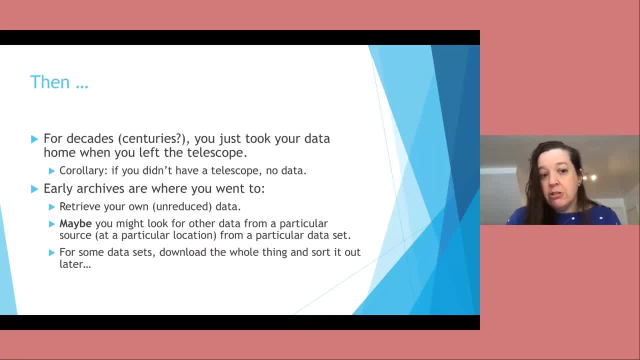 we're going to go down the digital rabbit hole and start, you know, poking around in these things more deeply. so for decades at least, if not centuries, you just took your data home when you left the telescope, and the ramifications of that is, if you are, if your institution, if your school, if 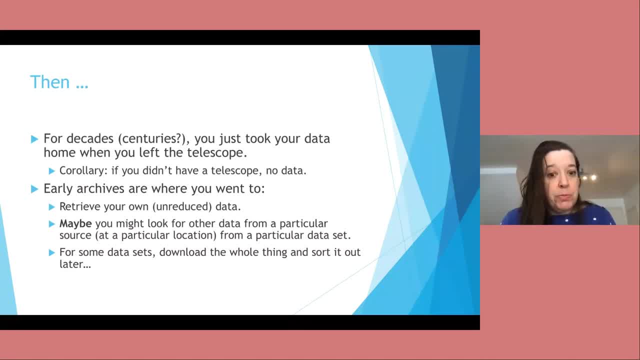 your state, if your country didn't have a telescope, you don't have any data, so early archives that was probably not ready to use right now. That's what I mean by unreduced. They're raw data and they still need to be processed before you can do science. 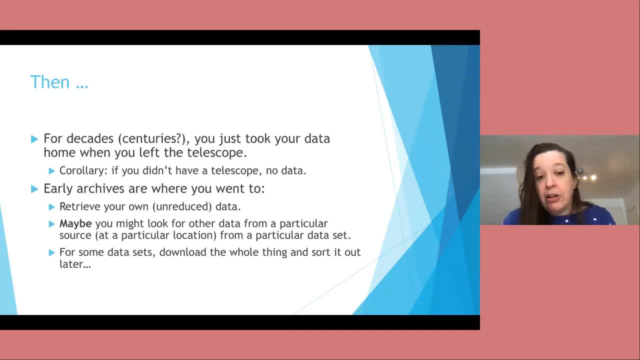 Maybe in those early archives you might look for other data from a certain source or from a certain data set, And for some data sets to be sure, you would just download the whole thing and analyze the data on your own computer when you downloaded the whole thing. 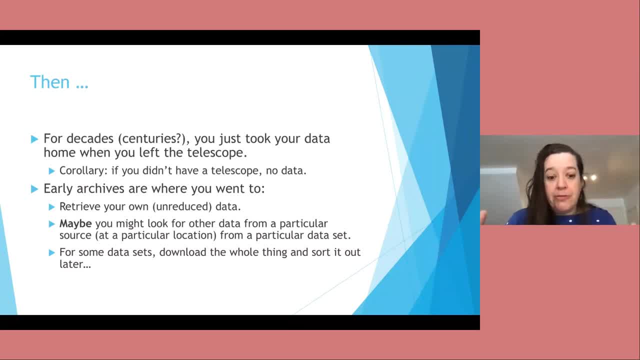 So 30 years ago, in the late 1980s, there was the very first infrared all-sky survey. It was called IRAS And IRAS was generating a catalog of all the infrared sources in the sky that it could see, And at the time it was an unprecedentedly large catalog. 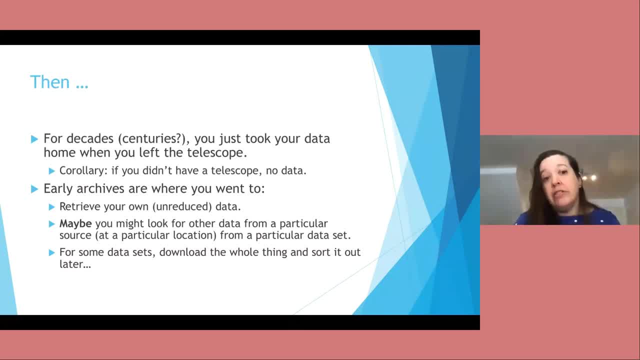 It was described as delivering an encyclopedia of knowledge every day, And there's interviews with the scientists from then who were like, oh, there's just so much data, Their big catalog. in the end you could email. It's only 200 megabytes and you could fit it on an iPhone. 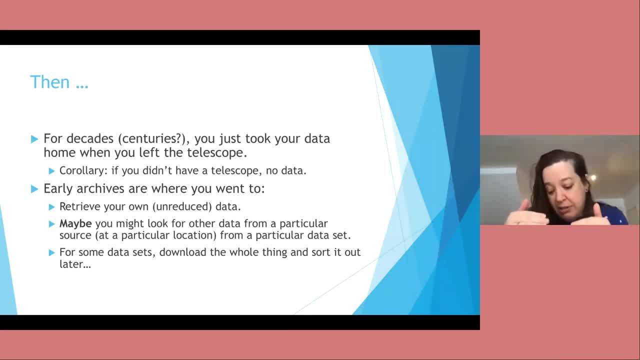 and you probably wouldn't even notice. But so that sort of set astronomers expectations for being able to download the whole catalog. And so more recently there's a survey called WISE, which is basically IRAS's successor. right, It's doing an all-sky infrared survey. 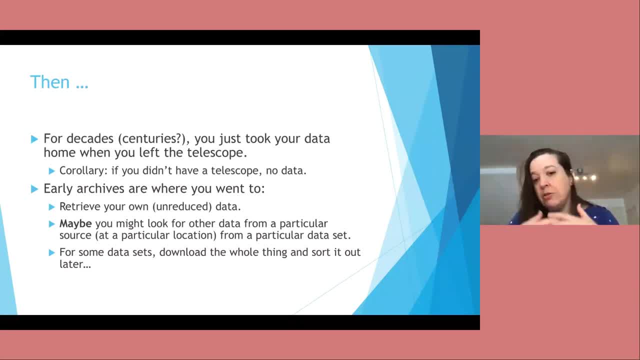 but it's much more sensitive than IRAS was. So there's millions more sources, And so when the WISE data first was made available, we had people who came and said, oh, can I download the whole data? And our reaction was: OK, ship us the disks. 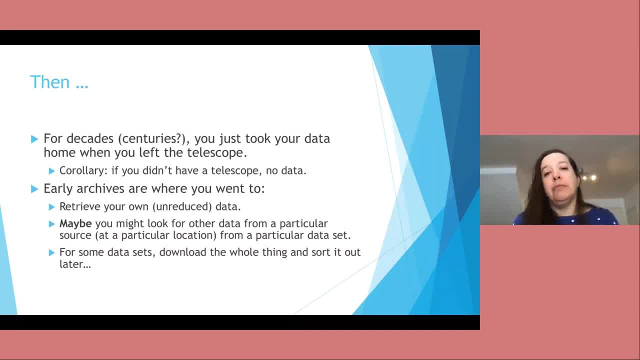 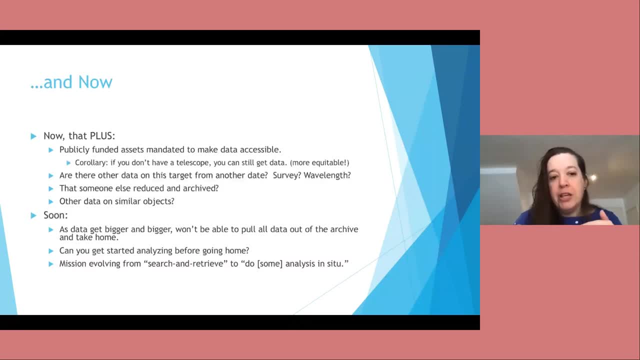 and then we'll fill up the disks and ship them back to you. And they were like what? Because it's a dramatic shift in how people think about archives. So now, any publicly funded assets, if you have a telescope that's funded by tax dollars. 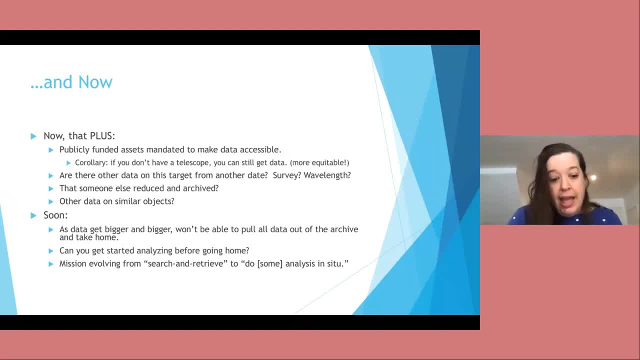 you have a mandate to make that data accessible. And the question is, how do you do that? And the corollary to that is, even if your school, your state, your country doesn't have a telescope, you can still get data. 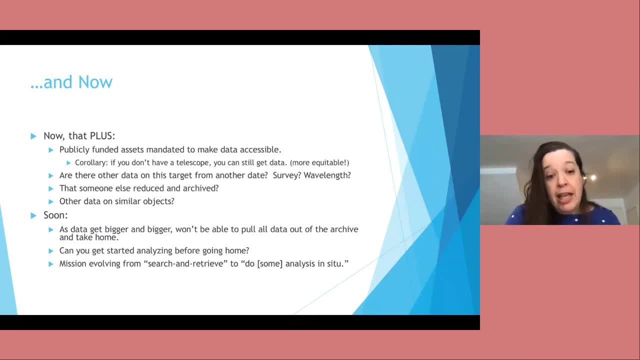 And that's very much a more equitable approach, And you can then use these archives to look for other data on the target that you care about, from another date or another telescope or another wavelength, or that someone else has already done most of the grunt work. 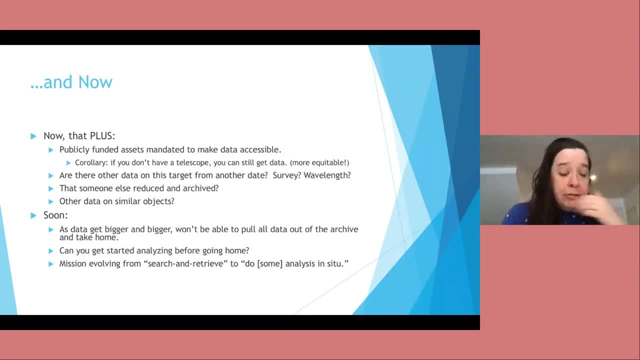 So you can just pick it up and do science. There are certainly people who are looking for other data on similar objects. There are other locations in the archive And soon, because the data are getting bigger and bigger and bigger all the time. it's not. 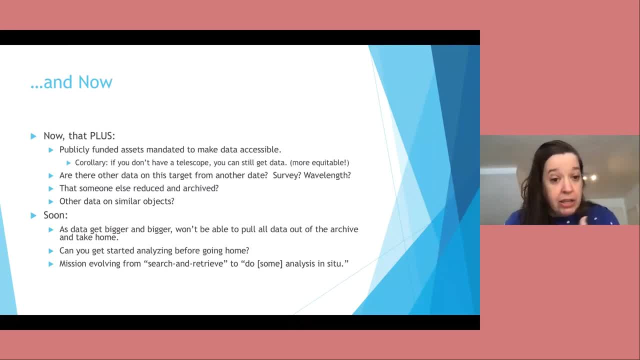 going to be possible to pull all the data out of the archive and take it home to work. So we're moving towards a model where you can start doing some analysis at the location of the archive before taking just a subset of the data home. So our mission is actively evolving right now. 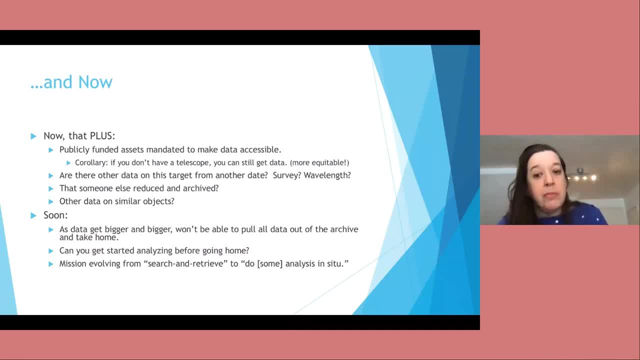 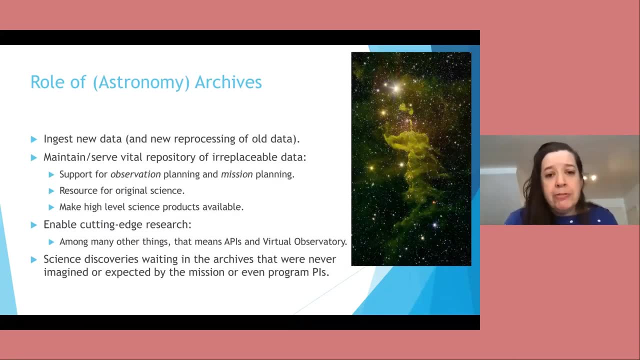 from a search and retrieve model to a model in which you do at least some analysis in situ at the archive and then take home And you can see that this is an amazing piece of data that's been made And the main thing that we are working on. 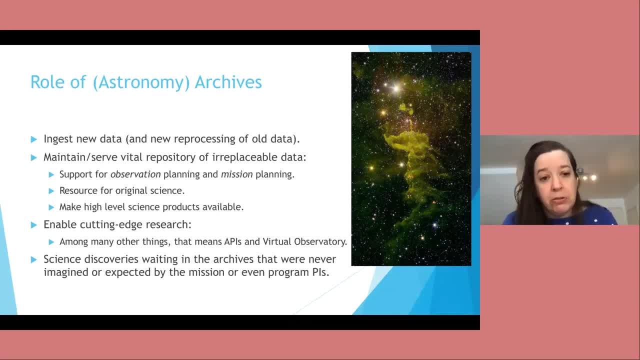 is actually trying to get the data out of the archives to work with. So the primary role of astronomy archives is to ingest new data, but also new reprocessing of older data, And we've built all these telescopes and accomplished all of these observations and kept track of all this data. 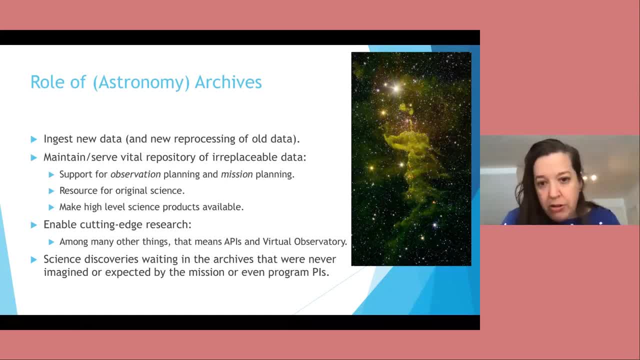 We don't want to lose it. There's a lot of blood, sweat and tears that have gone into these data, And so we don't want to lose them, And so that's the primary purpose is to maintain and serve all of this irreplaceable data In the context of NASA archives. we want to keep the data out of the archives. 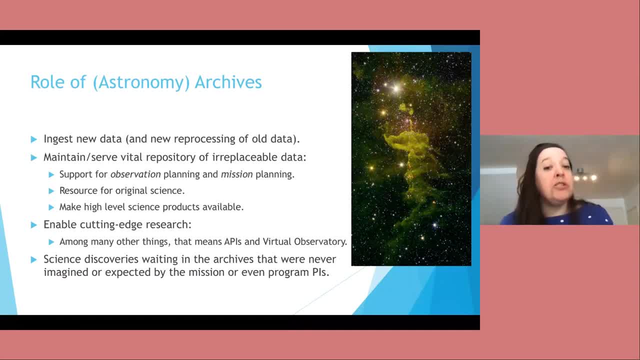 So we're working on the data for the future. in particular, we're not only supporting observation planning, but we're also supporting mission planning and of course, there's, you know, lots of original science as possible in the archives, and the archives can make them high-level science products available so that you can grab it. and 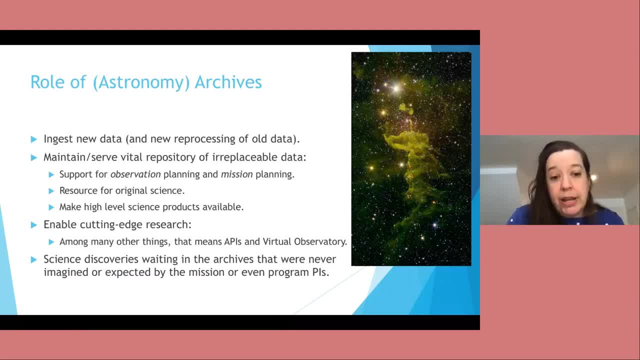 start doing science right away, and in order to enable that cutting-edge research, among many other things, that means that we have to have ways in which you can interact with the archive by program, using apis, using something called the virtual observatory, which is supposed to connect observatories worldwide with the same protocol so that you can download data from all of these. 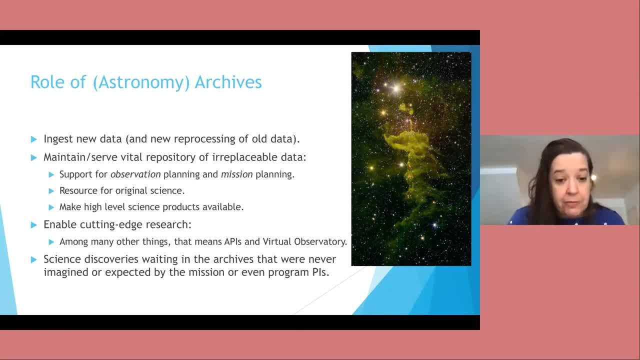 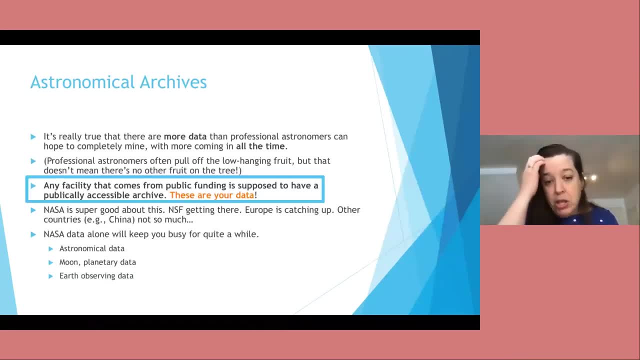 different locations, and so, to be sure, there are tons of science discoveries that are waiting in the archives that were never imagined by the people that originally built the mission or planned the data acquisition. so there are more data coming in than we can hope to completely mine, and there 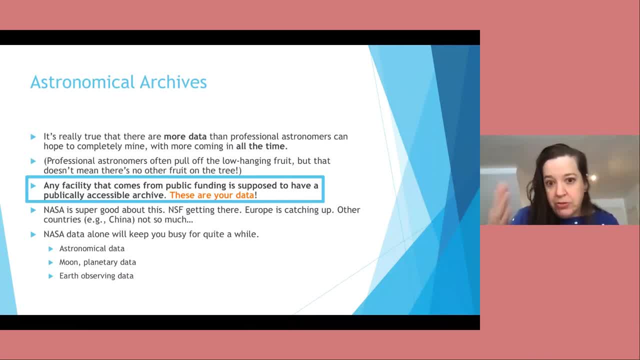 are more data coming in all the time and there is going to be more and more facilities coming on. in the relatively near future that's going to even, you know, even exceed that current glut of data. so the professional astronomer are all are going to pull off the really popular stuff or the easy stuff. but that doesn't mean 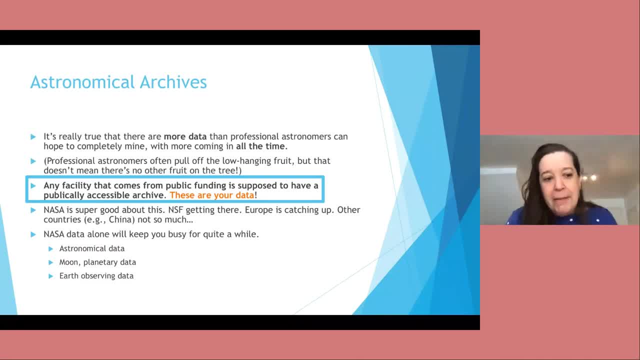 that there's not any more stuff in that data to find. and, just to remind you, any facility that comes from public funding is supposed to have a publicly accessible archive. these are your data too. nasa is really, really good about making the data accessible. nsf is getting there. europe is. 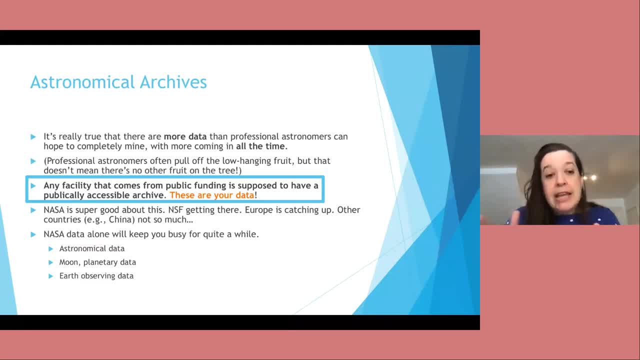 catching up. there are other countries that are a little bit more uneven, but the nasa data alone will keep you busy for quite a while, and nasa has lots of data in astronomy, in terms of things outside our solar system, so they'll probably provide you with the quick search links for our solar system. 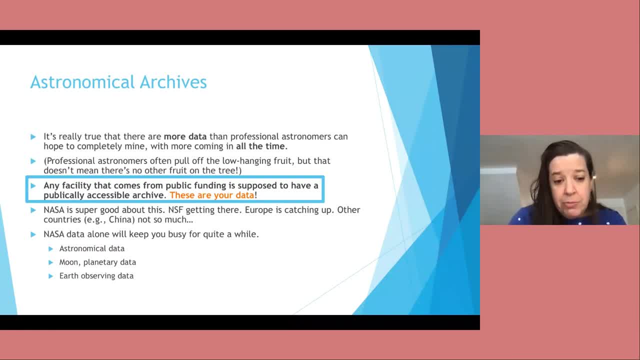 and they'll also be designed to easily access things from the moon and other planets in our solar system, but also earth observing data. i know the least about earth observing data and i am an astronomer, so i'm going to, as opposed to a planetary scientist, so i'm going to focus the 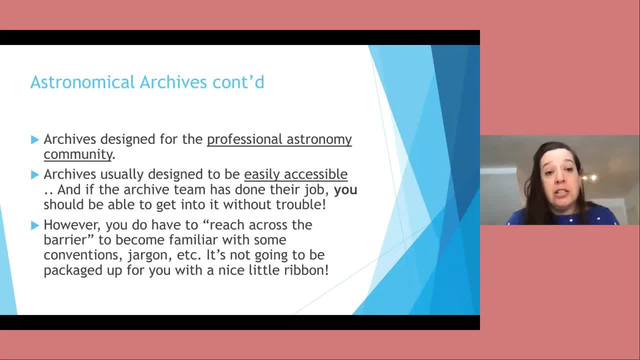 rest of this talk on the astronomical data, but i'll mention some of the planetary data when we get into this a little bit. so the archives are designed for the professional astronomy community and that means that they have to be easily accessible to everyone in the professional astronomy community, everybody from. 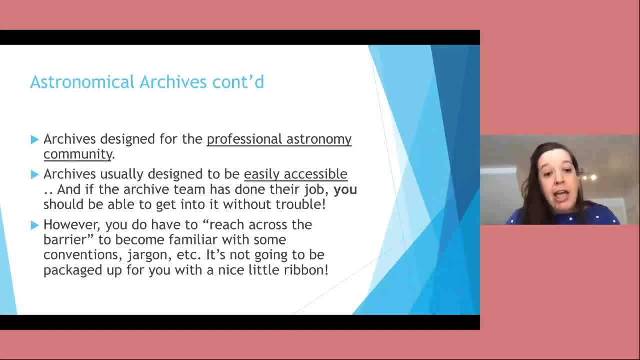 way down to a summer student starting her very first research project ever and in order to reach all of those people. that means you should be able to get into it without trouble, but you do need to become familiar with the conventions and the jargon, and the data are not going to be packaged up for. 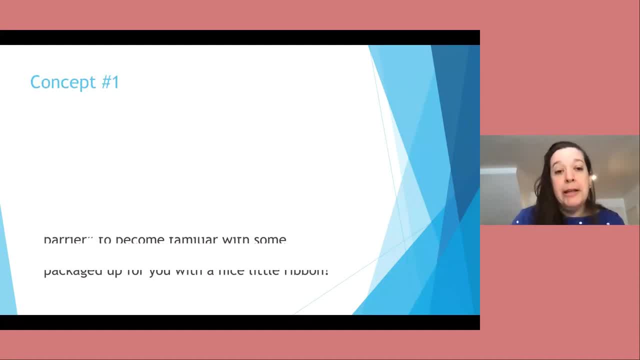 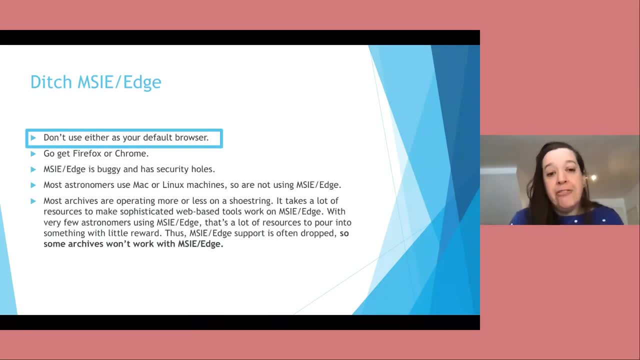 you with a nice little ribbon. it's going to take work to get into it. so the first big concept on how to do this is: don't use internet explorer, just don't do it. you should be using firefox or chrome. uh, internet explorer in particular, but also edge, has issues and most astronomers, it turns out, use. 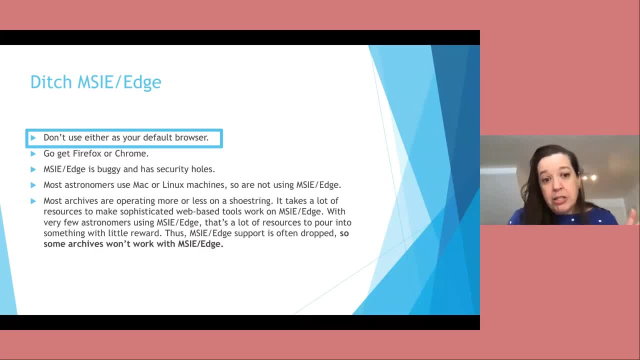 mac or linux machines. very few of them use windows machines, and so, since most of these astronomy archives are operating on a shoe string, it takes a lot of work to make some of these web-based tools work for these microsoft products, but because there are so few astronomers using those microsoft, 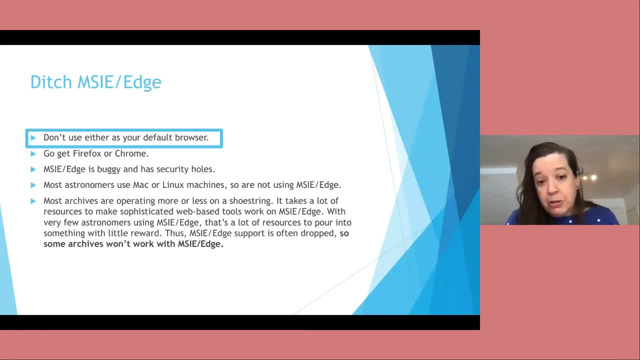 browsers. that's a lot of resources for the archives to pour into something with very little payoff, and so some archives won't even work. if you try to find a way to do that, you're going to have to do a lot of research and you're going to have to. 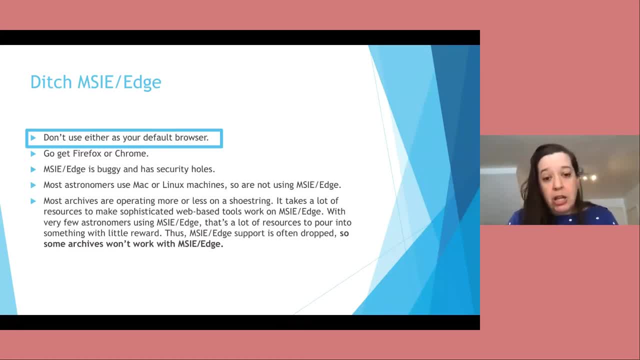 do a lot of research, and you're going to have to do a lot of research and you're going to have to try to access them with internet explorer or edge. um, like, literally like, the main home page for ursa wasn't working on microsoft products for at least six months and nobody noticed. okay, so just get rid. 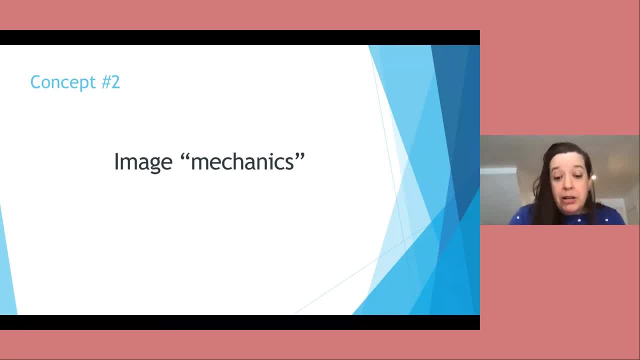 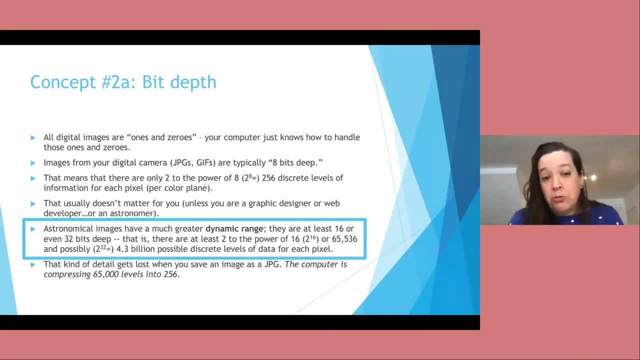 of it. use firefox or chrome. now the other. the next big concept is the mechanics of how to deal with the images. so all digital images are ones and zeros. it's just that your computer knows how to show those ones and zeros as an image. so the images that you take from your digital camera or your phone, 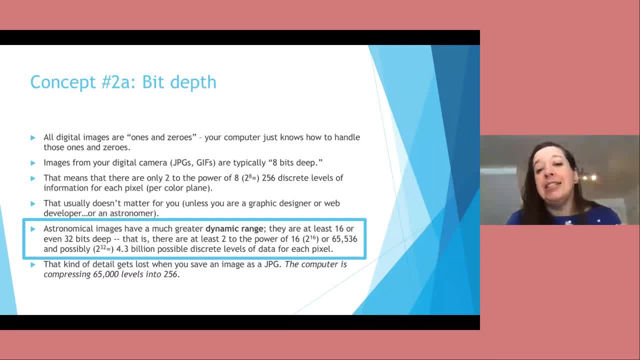 are typically jpegs or gifs, and those are typically 8 bits deep. what that means is each pixel has only two to the power of eight or 256 discrete levels of information in each pixel. that usually doesn't matter to you, unless you're a graphic designer or a web developer or an astronomer, and 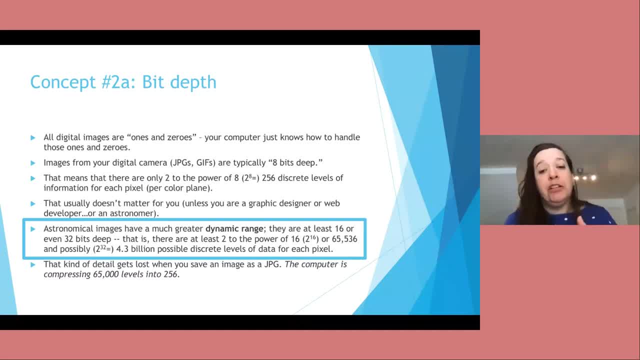 astronomer. astronomy images have a much greater dynamic range. they're either 16 or 32 bits deep. that means that there's two to the power of eight or 256 discrete levels of information. those are power of 16 or 2 to the power of 32 possible levels of data in each pixel. so 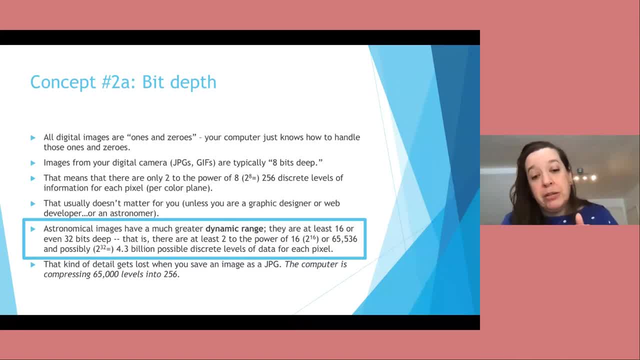 if you take one of those 16-bit or 32-bit images and save it as a JPEG, that you're gonna lose a ton of detail because you're asking the computer to compress 65,000 levels into only 256 levels, and so you lose a ton of. 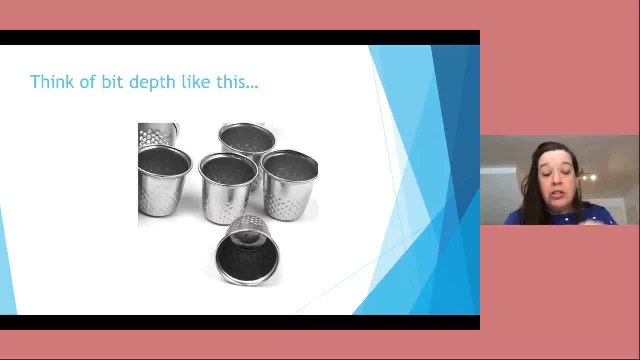 information when you save an image as a JPEG. so the way to think of bit depth is like this. so if you have a thimble doesn't hold very much water, it holds like a dribble of water. so if I have an array of thimbles I can't get much more. 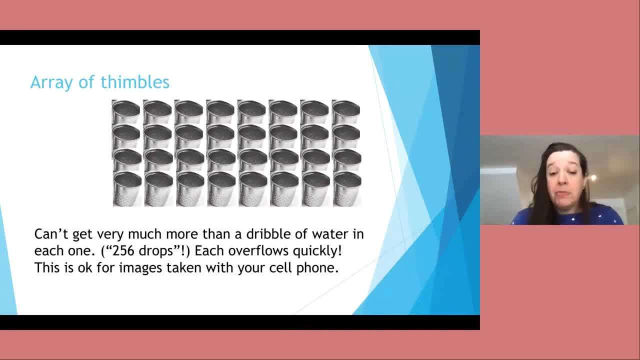 than a dribble of water in each one, let's say, 256 drops, and so each one of those little thimbles is going to overflow quickly, and that's totally fine. for images that you take with your cell phone, that's totally fine. so I'm trying. 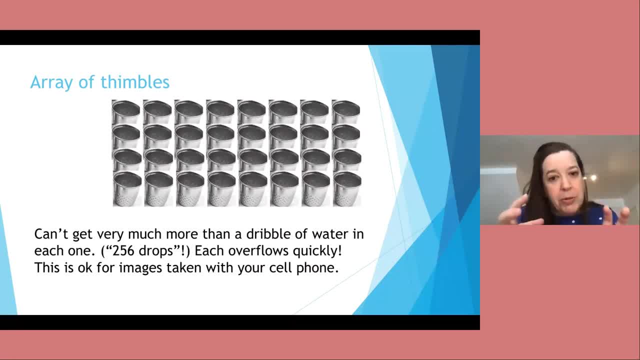 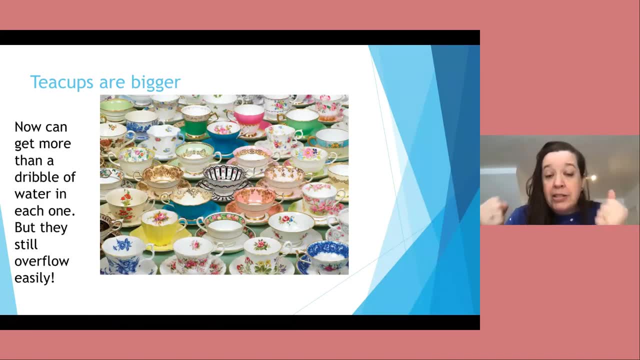 to figure out what I can use to explain bit depth, right. so thimbles are really tiny. what's bigger than a thimble teacups? you can get in a more than a dribble of water in each one, but the teacups still overflow easily, so trash. 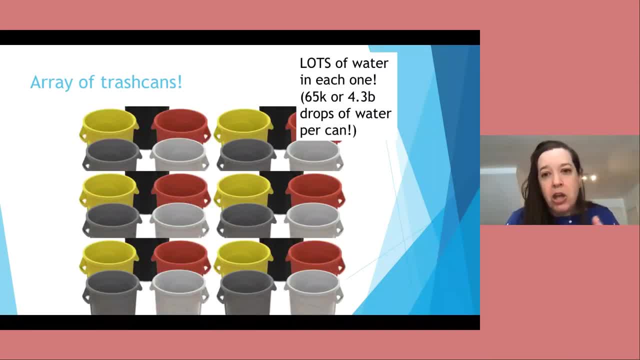 cans. trash cans are good, so think of it as an array of trash cans where there's lots of water that you can hold in each trash can. 65,000 or four point that, four point three billion drops of water in each can. so the the main, the main thing. 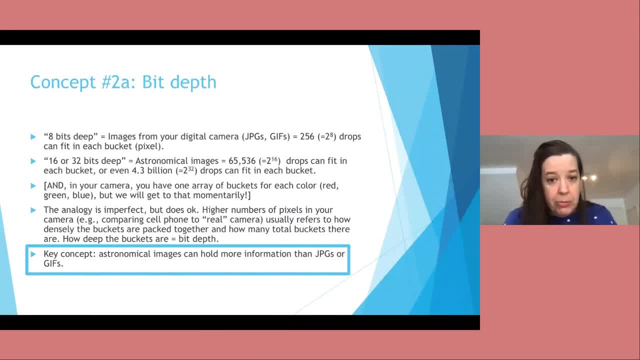 to take away from this is that images from your digital camera, like JPEGs or GIFs, are only 256 drops of water, so only two to the eight. eight bits meaning 256 levels, assuming 256 levels of information can fit in each bucket, but if you have 16 or 32 bits, which are 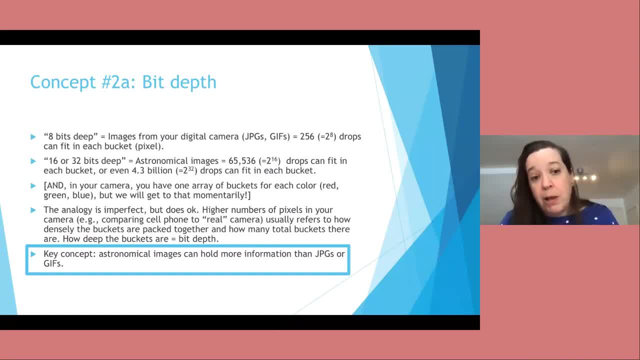 astronomical images. you can fit a lot more drops in each bucket. you can fit a lot of water in each bucket and it turns out in your camera. you have an array of buckets for each color, but we'll get to that in a second. so the analogy of 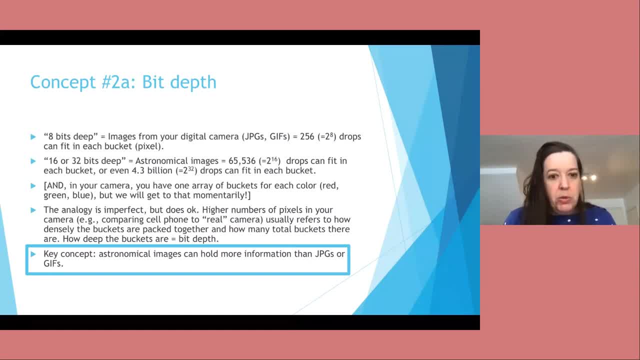 collecting water is imperfect, but it does okay. companies are trying to sell you digital cameras. they usually talk about how densely the buckets are packed together and how many there are, but I'm talking about something different. I'm talking about how deep the buckets are and that's bit depth. so the key concept here is it: astronomical images hold way. 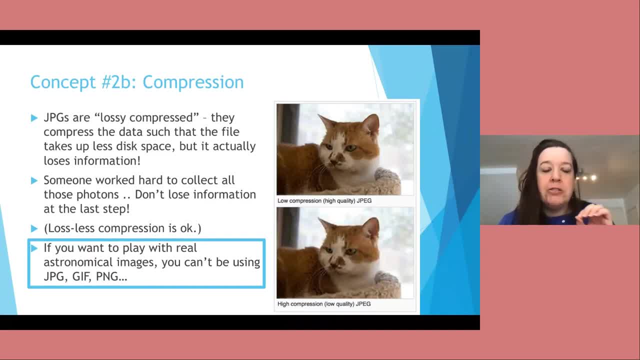 more information than JPEGs or GIFs and, moreover, JPEGs are something called lossy compressed. they compress the data so that the file takes up less disk space, but you lose information. I don't know if you can see on your screen, but the cat on the left is a cat and the cat on the right is a cat and the cat on the left is a cat and the cat on the left is a cat and the cat on the left is a cat and the cat on the right is a cat and the cat on the right is a cat. 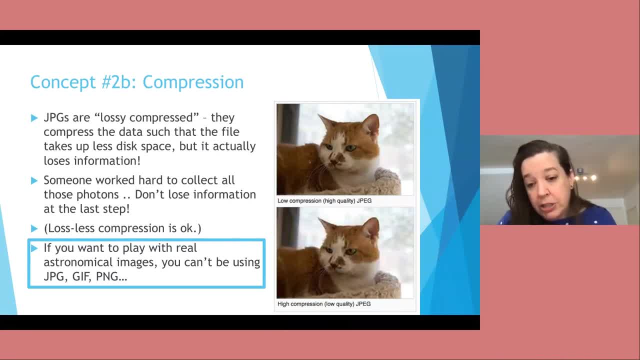 on the top is low compression, So it's a high quality JPEG and the cat on the bottom is the same image, but with high compression or low quality, And you can see that there's blockiness in the background. You can see the edges of the cat's head, sort of ring. 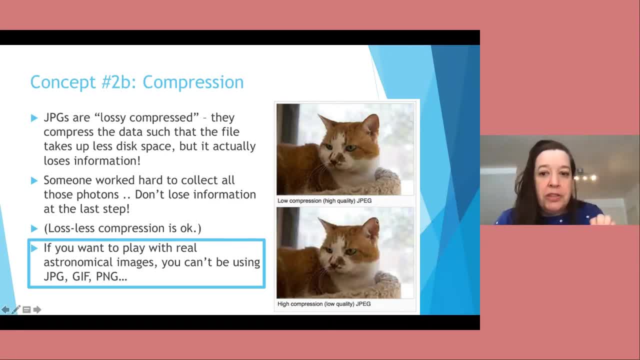 You get sort of an echo of the cat's head. So that's what I mean by lossy, compressed, It's losing information, And especially in the context of astronomy images. somebody worked really hard to collect all those photons. Do not lose information at the very last step. 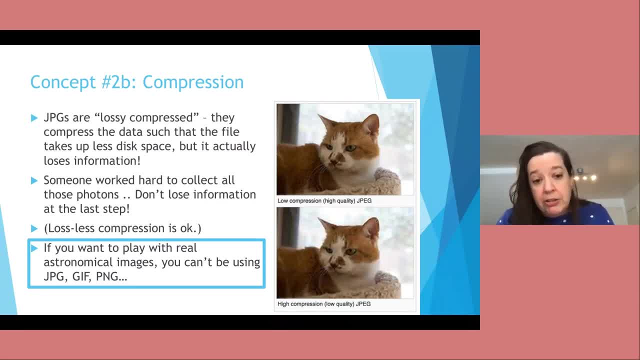 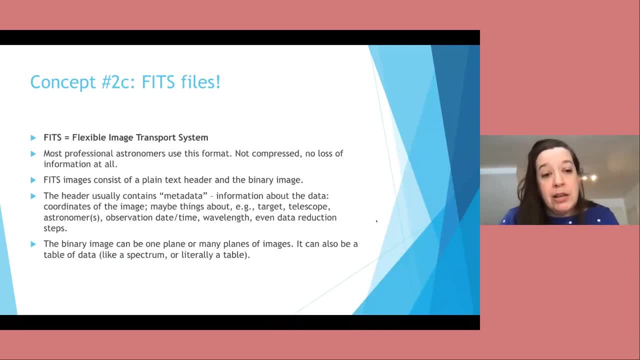 Of course, loss less compression is okay, But the punchline here is that if you wanna play with real astronomical images, you cannot be using JPEGs or GIFs. You need something else, And that something else. the most commonly used format in astronomy is called FITS. 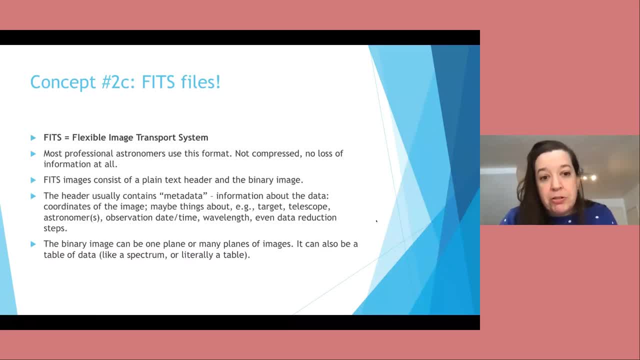 which stands for Flexible Image Transport System. Most professional astronomers use this format. It's not compressed, There's no loss of information And it's basically a plain text header and the binary image. The plain text header is metadata, So information about the data coordinates of the image. 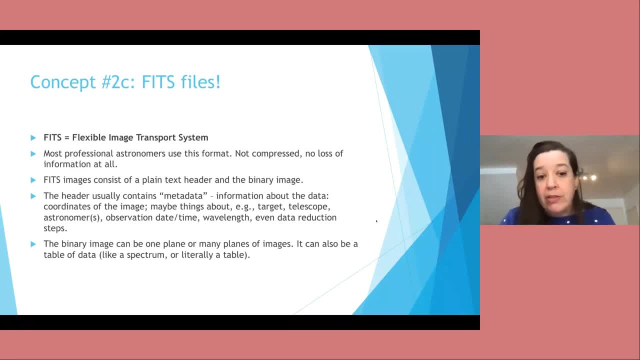 where it was looking, when it was looking, what telescope, what wavelength, what astronomer, what observation date and time it was taken And, depending on the provenance of the FITS file, it might even tell you a list of all the data reduction steps. 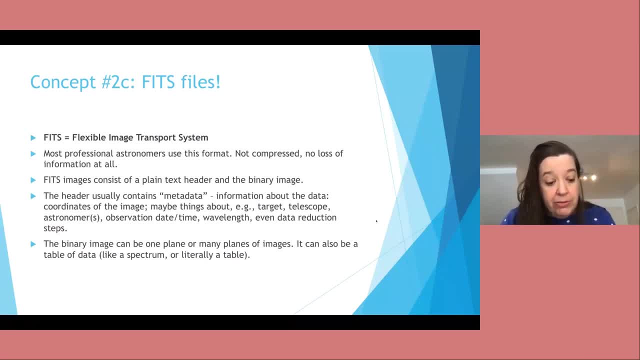 that have been applied to that image. So a minimal FITS header is just the position. Is this the position on the sky? But you can have a header that's really long talking about everything that's happened to that image. The binary image can be just one image. 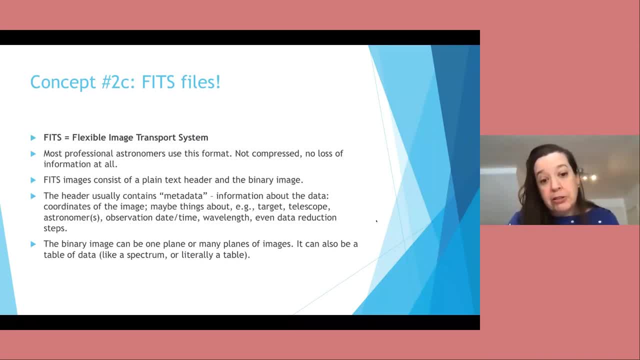 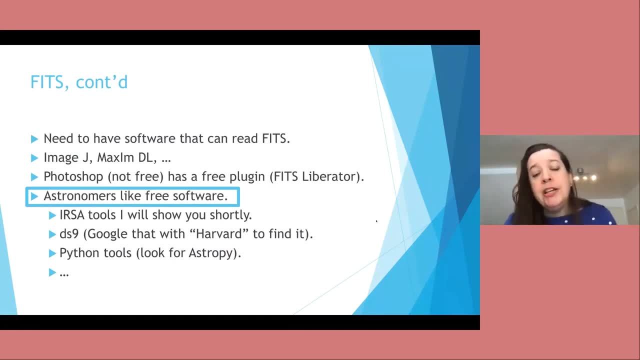 It can be just one plane, or it can be many planes of images And also can literally be a table, either like a brightness as a function of wavelength, like a spectrum, or literally a table of data. So you need to have software that can read FITS. 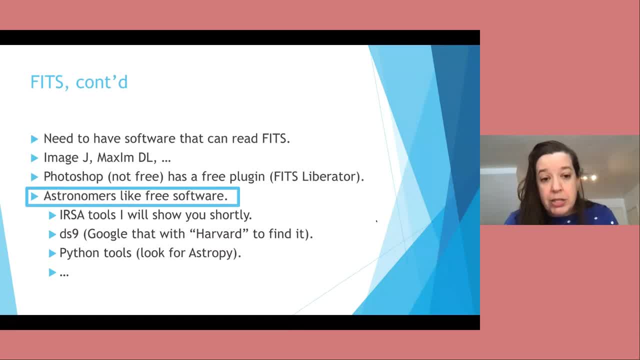 Amateur astronomers tend to use something called ImageJ or MaximDL. Photoshop, which is of course not free, has a free plugin to deal with FITS. It's called FITS Liberator, But in the end astronomers really like free software. 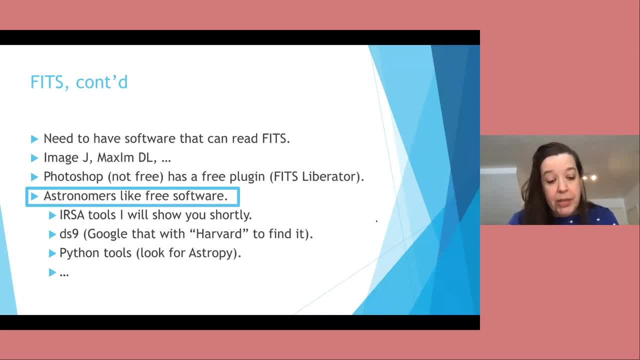 So I'm gonna show you the URSA tools in a little bit that are totally free. There's a tool called DS9, which you'll have to Google with Harvard to find, because, I mean, the reason it's named DS9 is not independent of the fact. 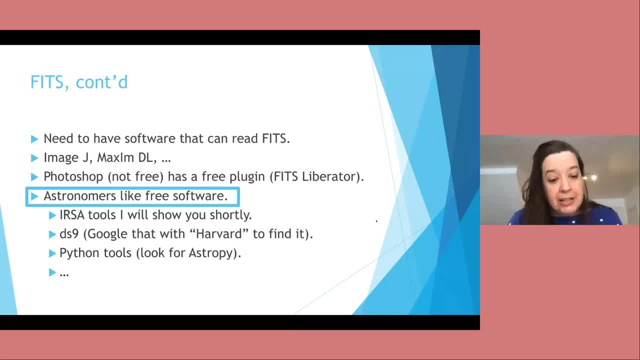 that there's a Star Trek series called DS9. But if you Google DS9, it's gonna take you to the Star Trek series. So you have to Google DS9- Harvard to find the program I'm talking about. And of course, there's a ton of Python tools as well. 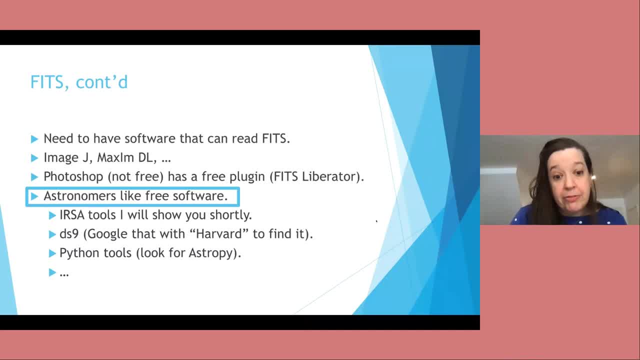 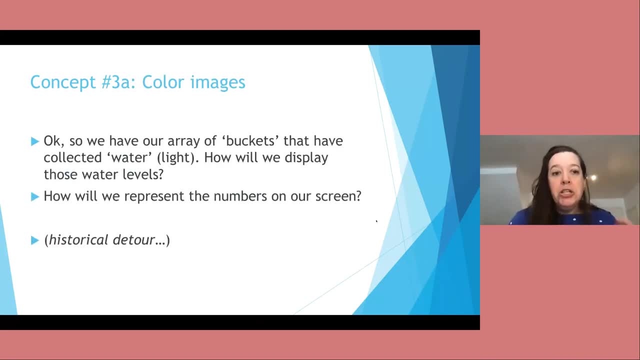 You wanna look for a package called AstroPy in order to find all of those tools. So to deal next, the next big concept is color in images. So we have our array of buckets that have collected water, So how are we gonna display those water levels? 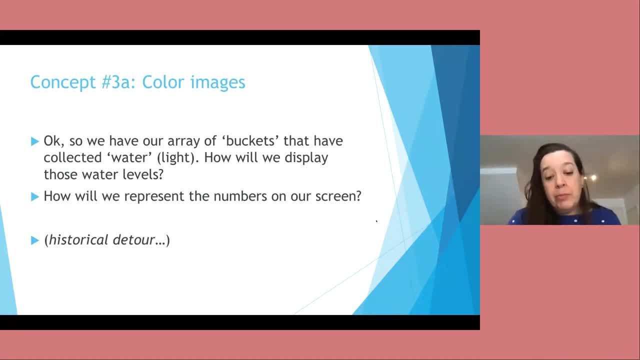 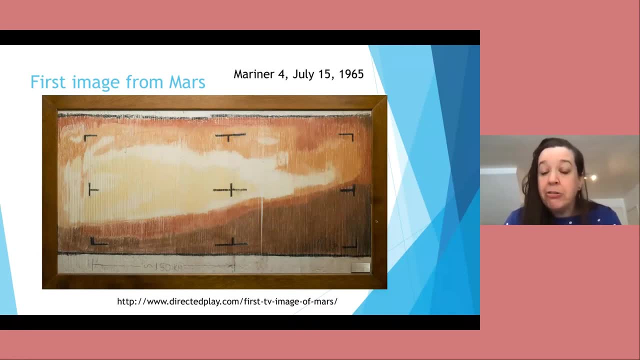 How are we gonna represent those numbers on the screen? So, in order to explain that, I'm gonna take a brief historical detour. This is the very first image ever taken from Mars. It was from a spacecraft called Mariner 4. And the image was taken in July 1965. 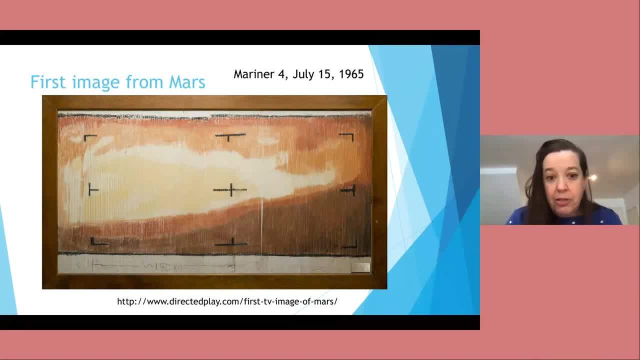 And the scientists and engineers that were dealing with the Mariner data were very impatient. They did not want to wait for the computer to chew and chew and chew on those numbers and turn them into an image. It was gonna take many hours for the computer to do that. 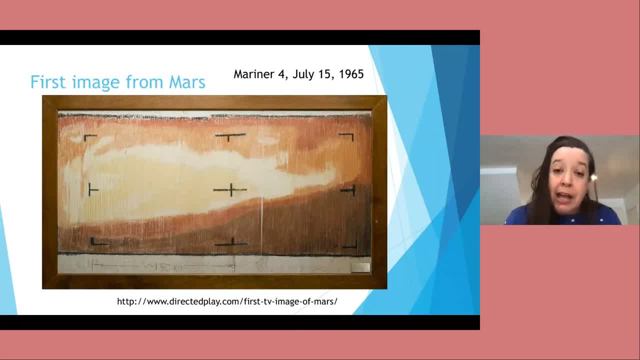 And they were too impatient for that, So they printed it out. They printed out the numbers on good old dot matrix paper, cut them up and taped them, stapled them into a bulletin board and then colored the numbers because that you know. they wanted to see what the image was. 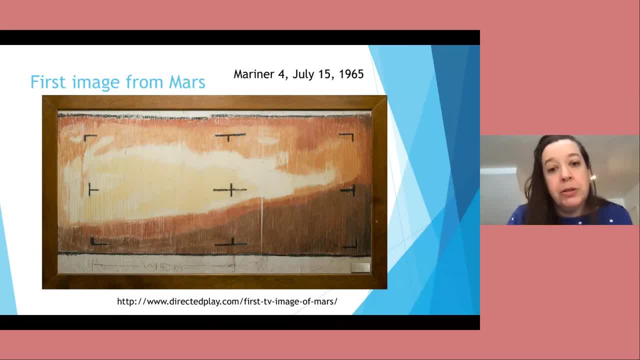 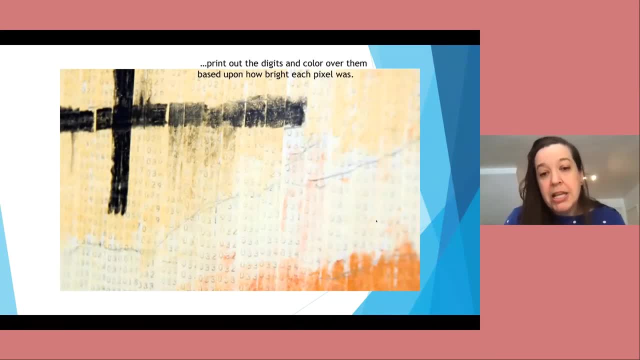 They wanted to see what the image was And they were going to be faster than the computer could generate the image. You think I'm making this up. I did not They are. they printed out the numbers on dot matrix printer paper, cut them up and colored them in. 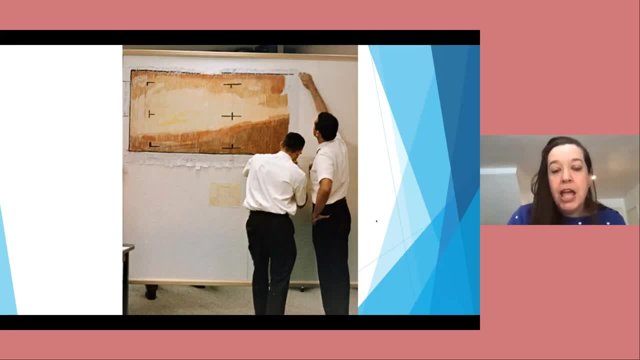 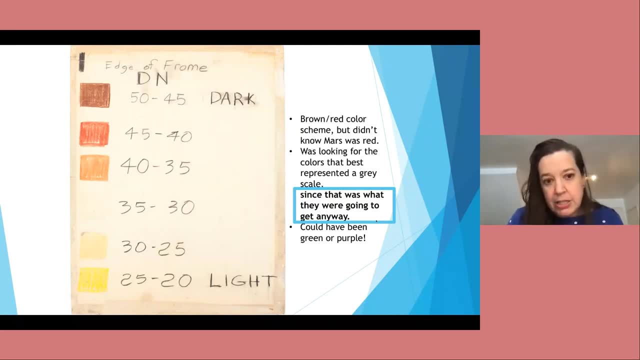 I am totally dead serious. That is exactly what they did, And they were trying to get shades of gray. They went to an art supply store and they were looking. they wanted to have at least six levels and they were seven. yes, six levels. 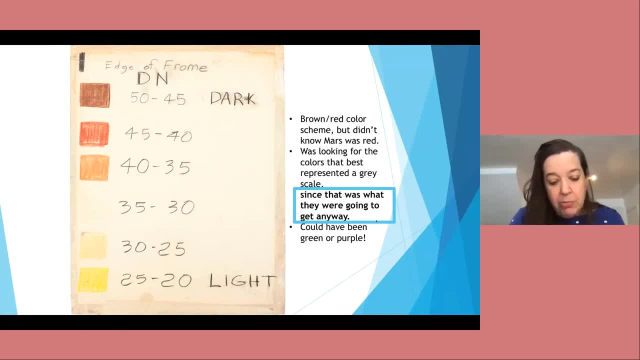 And they were trying to find. they were trying to find shades of gray- pastel box with that many shades of gray and they couldn't find one. And so at the time- remember this is the first image from Mars, So they didn't know that the sky on Mars was going to be red. 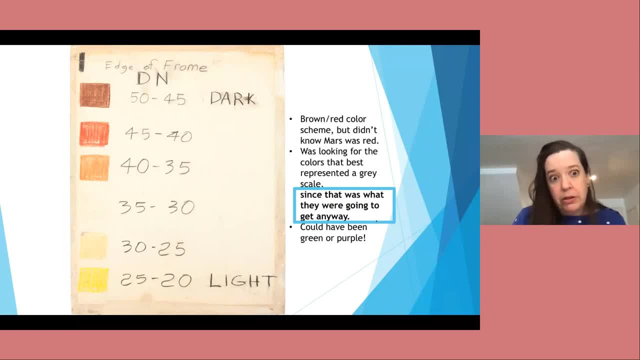 They didn't know. I mean, they knew Mars looked red when you go out at night, but that was all they knew. So they were like, okay, well, we need something that has like six different levels of color. So we're going to use sort of this red and brown. 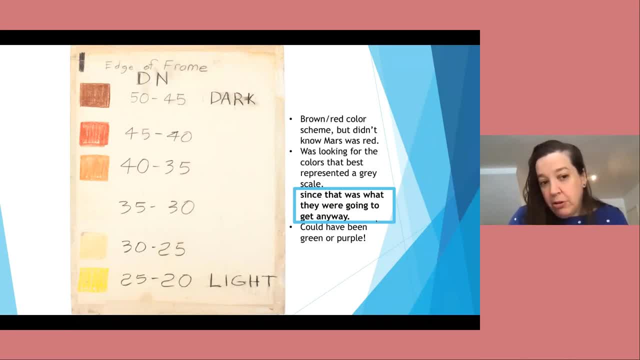 and yellow scheme, but because we can't find the grays, So they were going to, they're going to work with those. but they could have picked like six shades of green or six shades of purple, but they picked six shades and sort of the red color scheme. 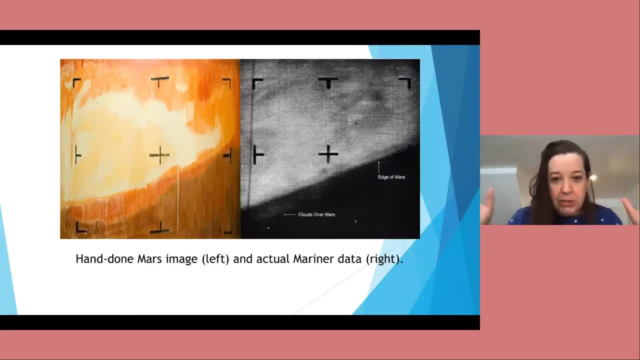 So there on the left they had- I've adjusted the aspect ratio, but there on the left is their original hand on Mars image And there on the right is the image that eventually was spat out by the computer from the Mariner data. 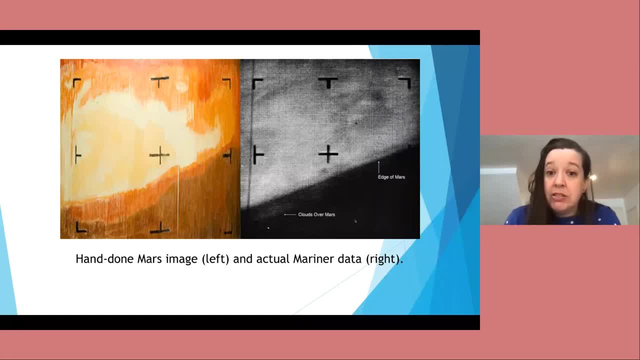 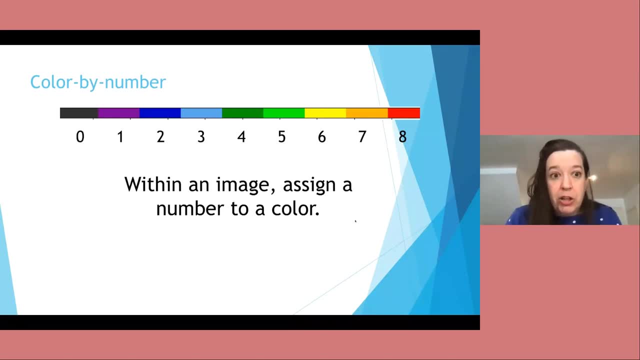 And they didn't do a half bad job. It actually there's definitely things that are similar between these two images, So that is literally so. you think of it as color by number, but that's literally how your computer is handling those images. 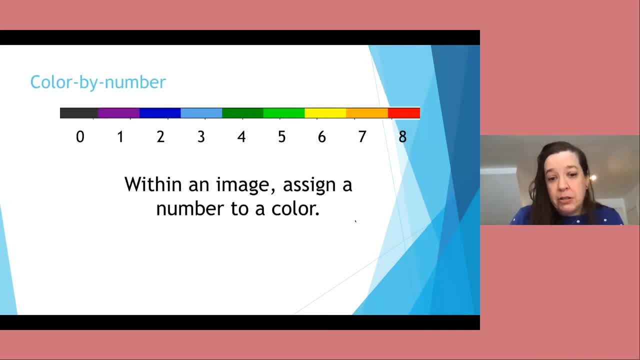 So within the image the number is assigned to a color. So I've got here a rainbow and I've assigned the numbers between zero and eight. but what if you have values more than eight, So you can start bundling them up, saying okay. 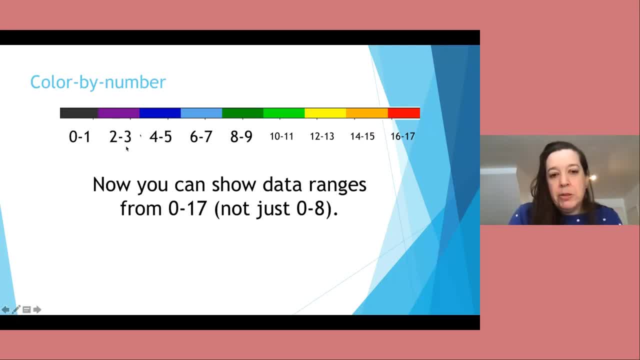 black is going to be zeros and ones, purple is going to be twos and threes, dark blue is fours and fives, and so on. So now I can show data ranges from zero to 17, not just zero to eight. but what color should i make? 7.9, i mean 7.9. 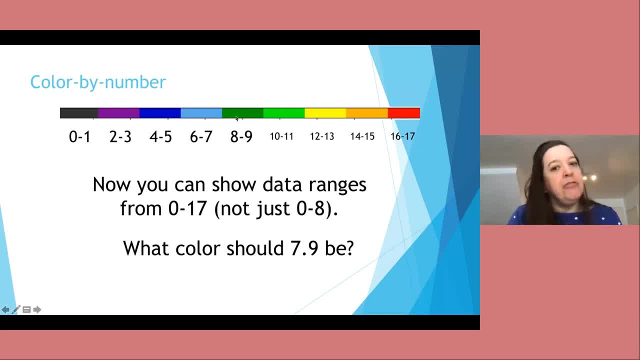 according to this color scheme should be light blue, but it's awful close to eight, which is this dark green. so, okay, let's make a more continuous spectrum of colors to represent the data ranges that we have. but we've been talking about dip bit depth. what if you have numbers that are much? 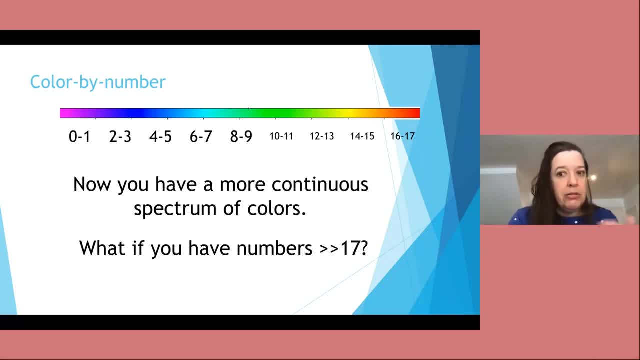 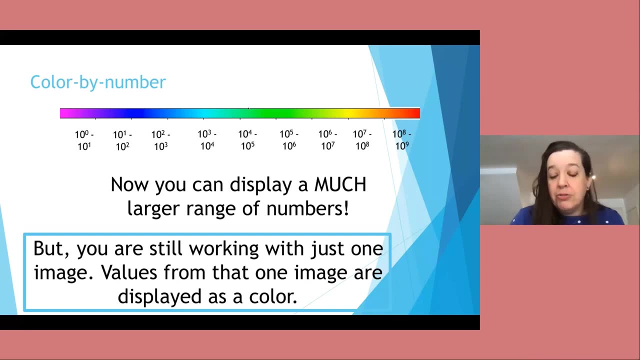 greater than 17. well, you can change that color to number correspondence and say, okay, i'm going to display now numbers between one and a billion using this color scheme. so for all of this, you're still working with just one image. it's just the values from that one image are displayed as a 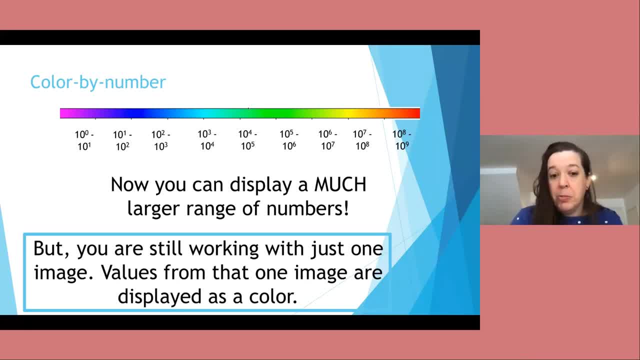 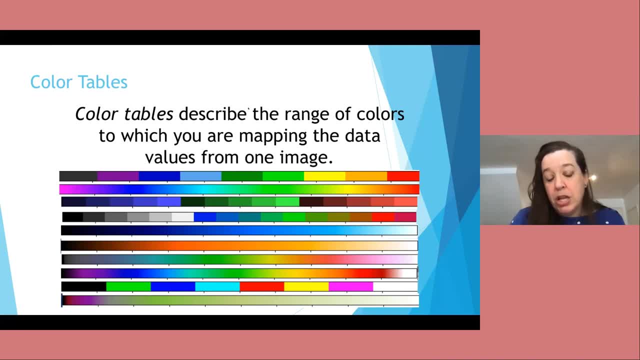 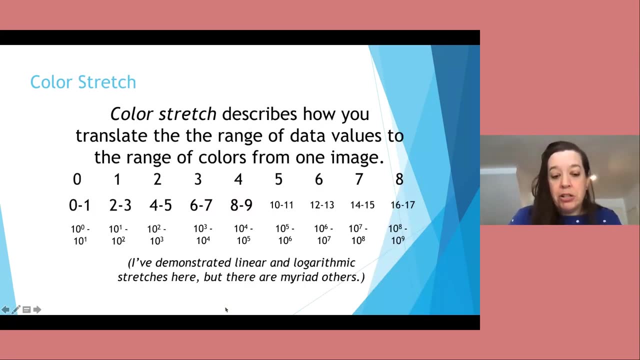 color and you get to pick how the colors and numbers correspond. so the the term color table describes the range of colors that you're mapping the data values from one image, and there's lots of them to choose from. these are some of the most popular. but the other term is color stretch color. 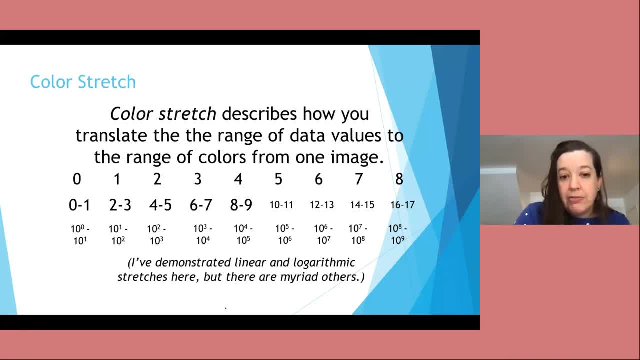 stretch is the color of the image and the color of the image is the color of the image, and the color stretch describes how you translate the range of data values to the range of colors in just one image, and so in these examples here i've demonstrated a linear stretch and a logarithmic 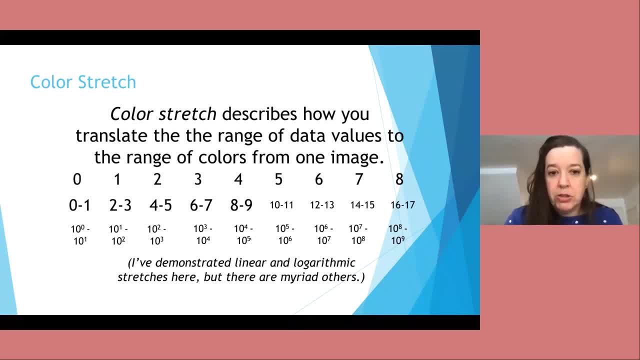 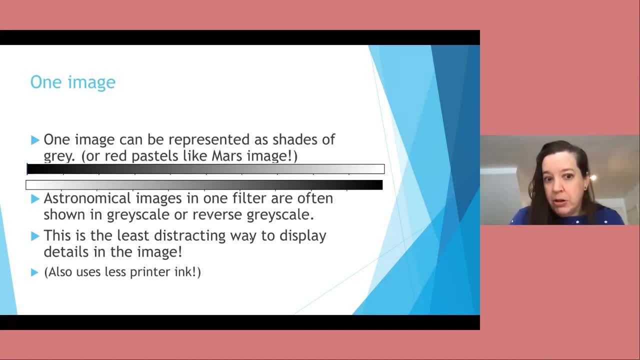 stretch, but there's many, many others that are used in astronomy in particular. so one image is can be represented as shades of gray or shades of red, like in the mars image. but the astronomical images that are in one filter are often just shown not just in grayscale, but often reverse grayscale. 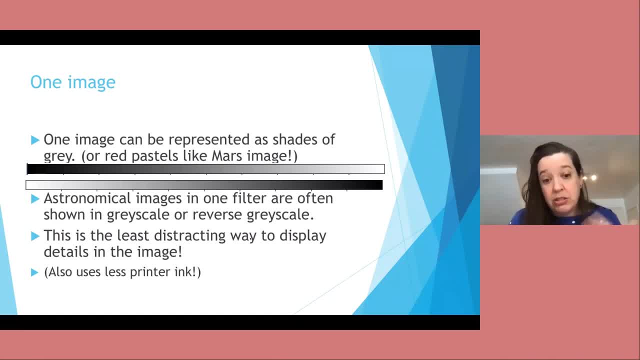 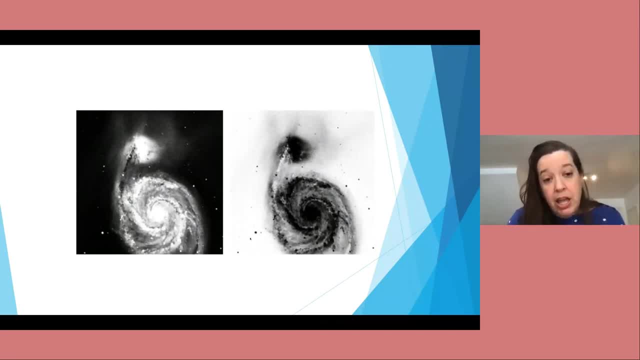 because it's the least distracting, and it's the least distracting and it's the least distracting way to display the details in the image and also, if you print it out, it uses less printer ink. so there's the same galaxy, but one is in grayscale and one is in reverse grayscale and you can see. 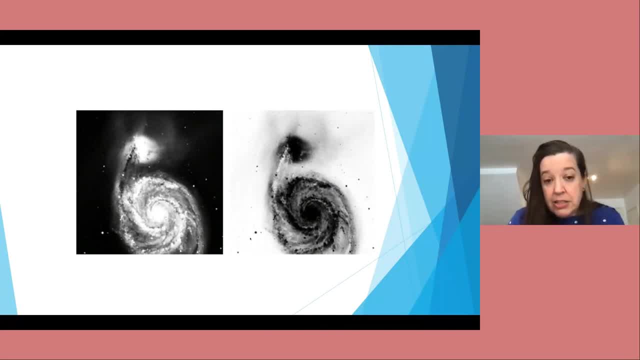 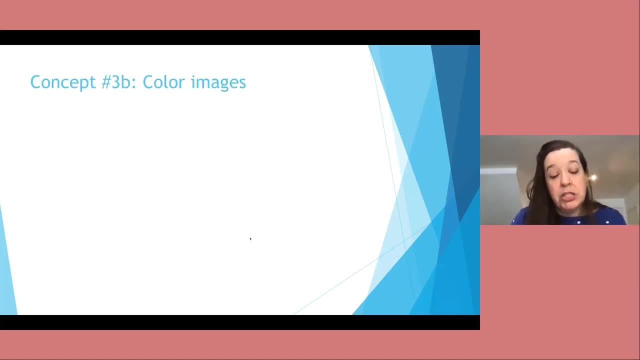 that your eye is drawn to different details in these images. it's the same color stretch, but it's just. the color table is different, and so you, you can pick your color table and, for that matter, your color stretch, to reveal what details you care the most about in your images. so the next big concept: 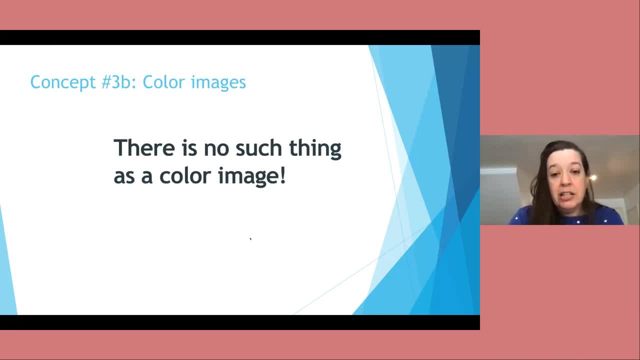 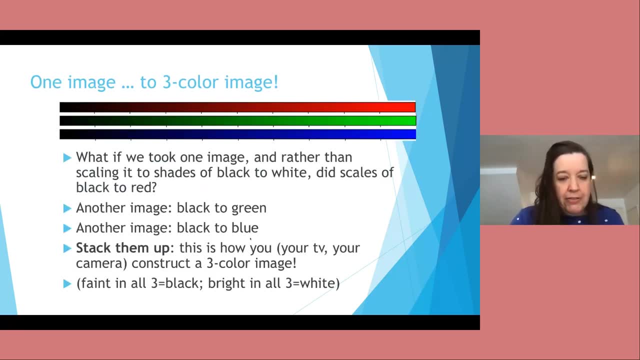 in color images is that there is no such thing as a color image, and i can hear you all the way from here. what i'm looking at: a color image, well, you're. you're kind of not if you take one image and, instead of scaling it to shades from black to red to white, do scales from black to red and then 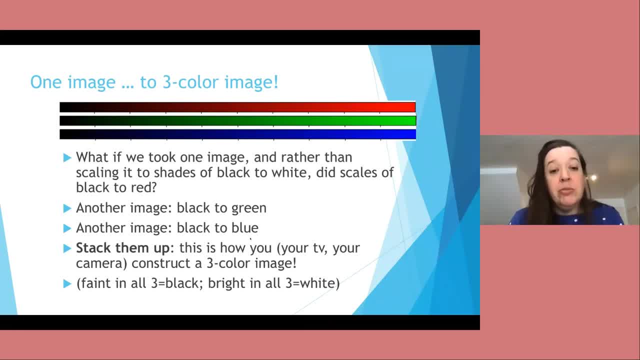 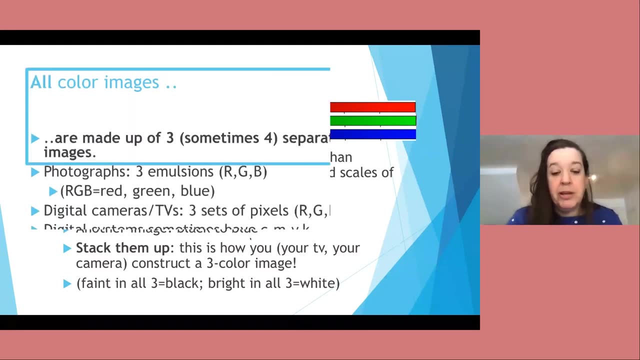 another image between black and green and another image between black and blue, and that is how you, or your tv or your camera, construct a three color image. something that's faint in all three is going to be black, something is going to be bright and all three is going to be right. so all color images are made up of three, sometimes four, separate images. 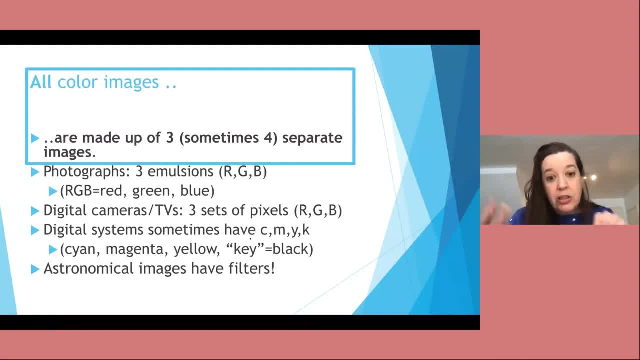 in old-fashioned color photographs, there's actually three emulsions in the film: one that's sensitive to red, one that's sensitive to green and one that's sensitive to blue. digital cameras or tvs have three sets of interwoven pixels. if you look at your screen. 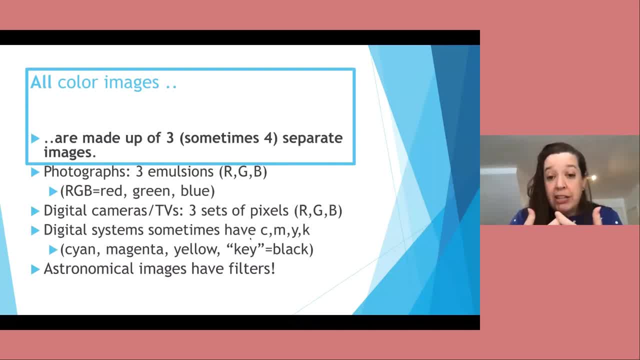 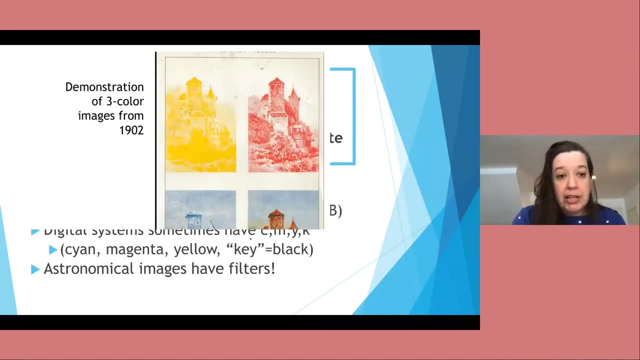 with a magnifying glass you can see those interlaced three sets of pixels. some digital systems have four sets of images: cmy and k, which stands for cyan, magenta, yellow and key, which is black. astronomical images have filters, which we'll talk more about in a second, but this 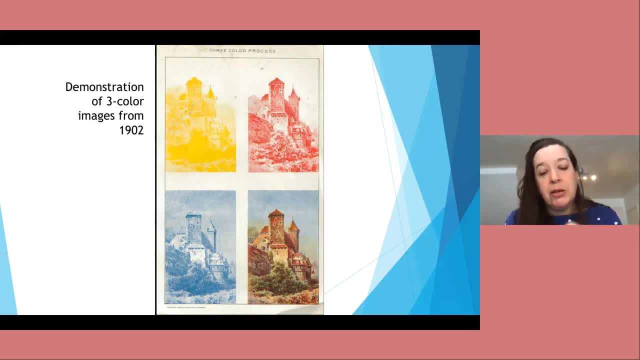 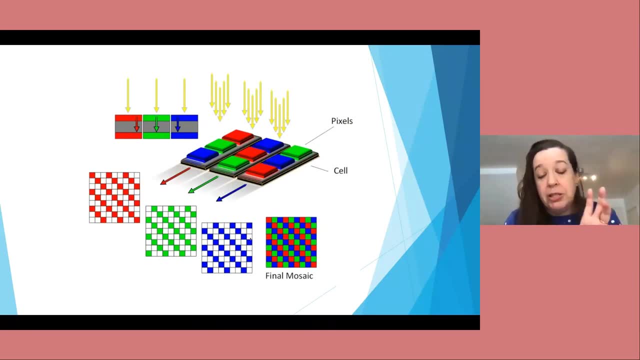 is a demonstration of three color image printing from 1902, where they're assembling a color image from red, yellow and blue, and this is, uh, actually something from a digital screens promotion materials, talking about the interwoven nature of their red, green and blue pixels in the final television product that they're selling. so in astronomy you take an image. 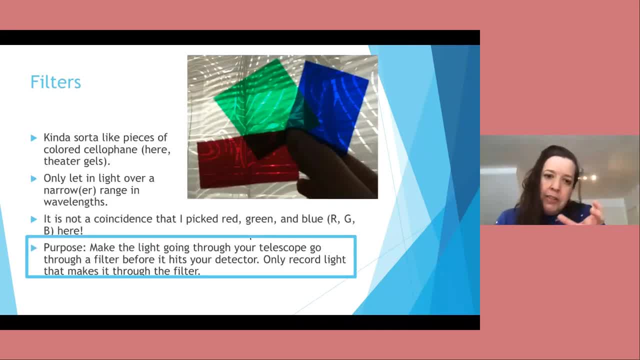 in one filter. but what do i mean by that filters? you can kind of think of them as like pieces of colored cellophane- here i'm using theater gels. so it's the. the blue filter only lets in blue light and the green filter only lets through green light and the red filter only lets through red light. so 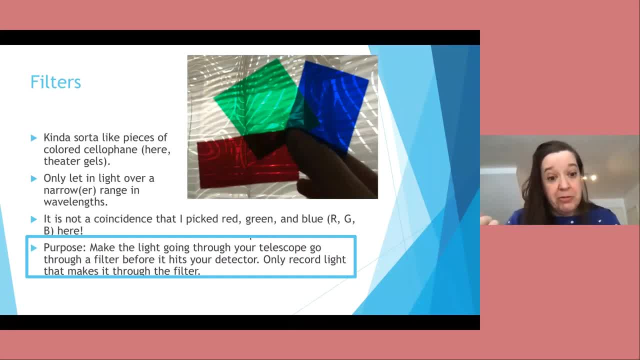 it's not a coincidence that i've picked red, green and blue filters for this example. the whole point is to limit the light that's going through your telescope so that you're only recording light that makes it through the filter. so in astronomy you take an image in one filter. you 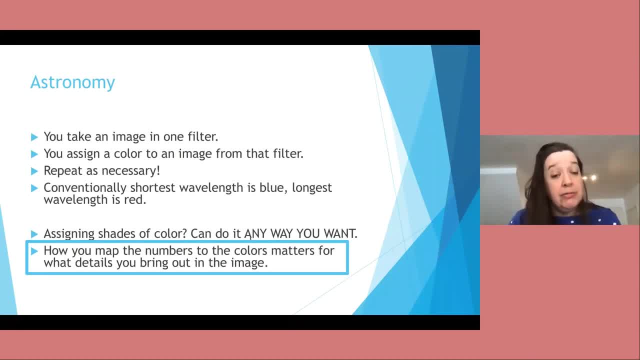 assign a color to an image from that filter and then you repeat. so conventionally you make the shortest wavelength blue and the longest wavelength red. but you can do whatever you want. you can assign shades of color any way you want, depending on what you want to bring out the image. if you're 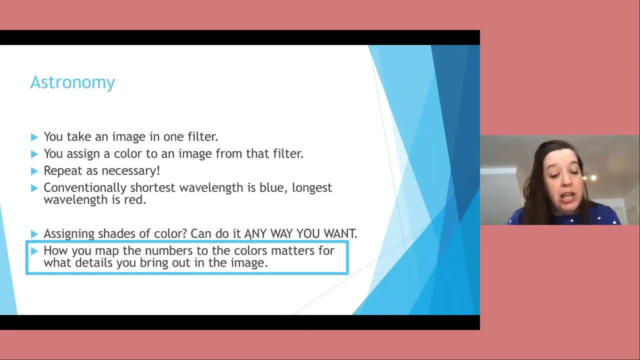 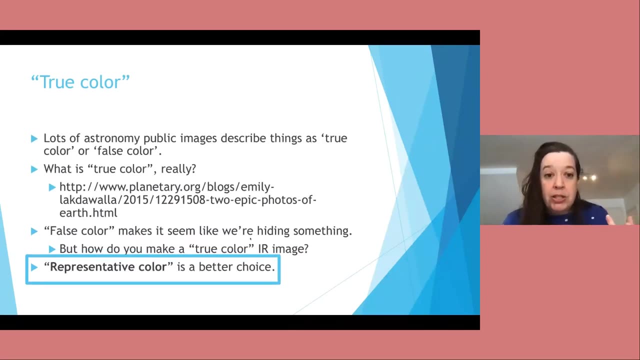 interested in the bright core of a galaxy, you're going to pick a different stretch than if you're interested in the fainter edges of the galaxy. how you decide to map the numbers to the colors you know is determined by what details you wish to bring out in the image. So lots of astronomy public image may mention things like true color. 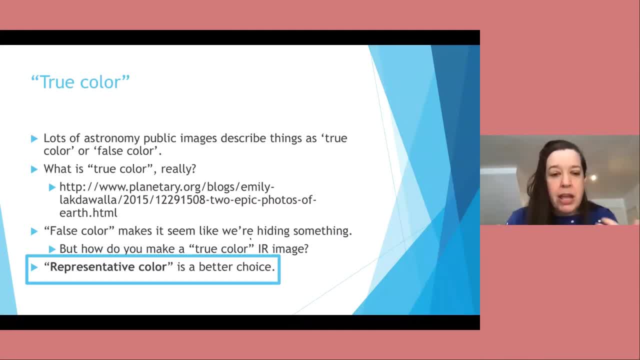 or false color, But that is really a confusing concept. Anyone who's done any interior design with any other human knows that no two people see color the same way, Because I myself have had conversations like that is not pink, How can you say that's pink? So people clearly look at. 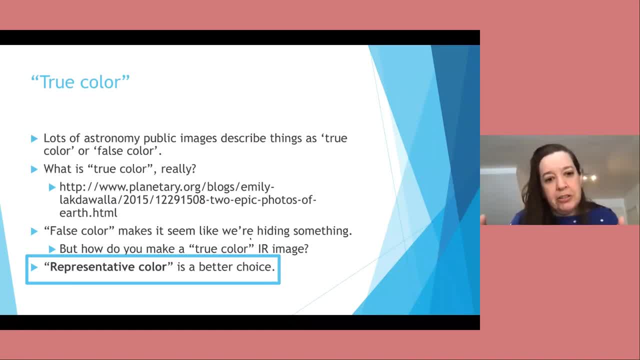 colors differently, And true color is really a difficult concept, And it turns out that in 2015,, there were two images that happened to be released on the same day from two different lunar spacecraft and they were taking pictures of Earth, And so there were two different pictures. 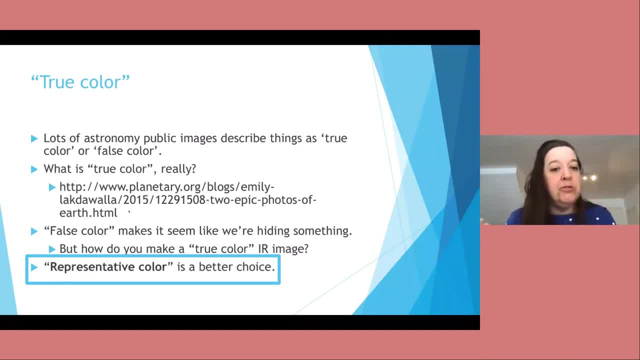 that were released by two different teams on the same day, both claiming to be true color, and they're totally different. So what does true color really mean? And the term false color I mean. let's be honest right now, in particular, language matters, And false color makes it seem. 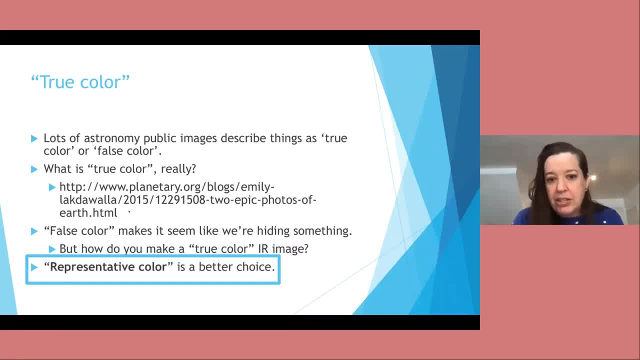 like we're hiding something, but we're not, Because if I'm taking an image in the infrared, a true color infrared image, is going to be black. it's going not going to be useful at all. So we have to translate those photons into light that we can see at the very minimum, very minimum. 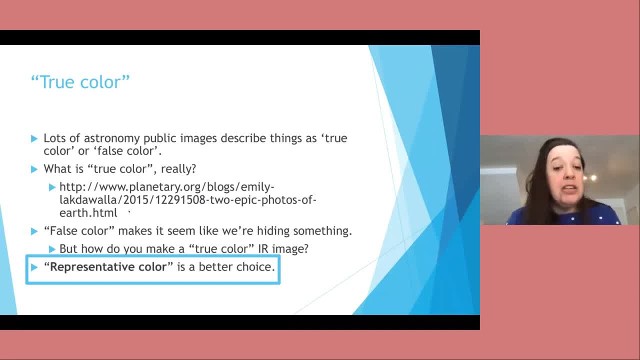 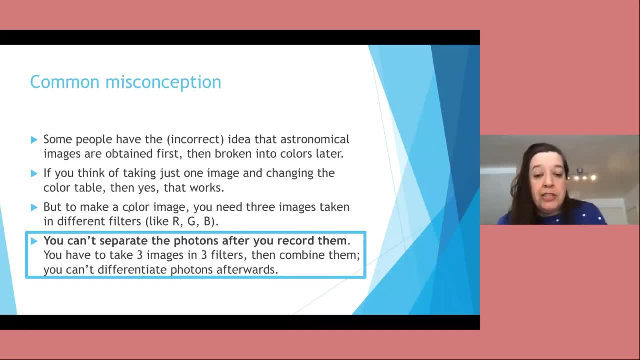 So instead of false color or true color, you should use the term representative color, because it's a better choice of terminology to explain what it is that you're doing. And some people have this incorrect idea that astronomical images. you take the image first. 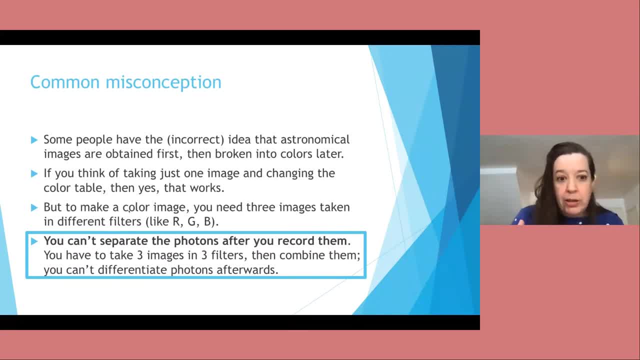 and then you break them into colors Later. certainly, if you take just one image and change the color table of the stretch, then, yes, that's the correct concept. But to really make a color image you need at least three images taken. 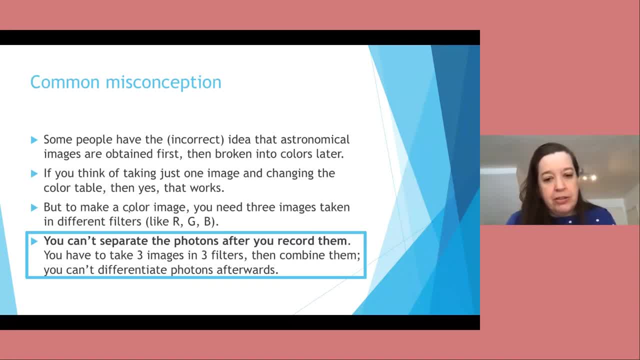 in three different filters And in general you can't separate the photons after you record them. you have to take three different images and three different filters and then combine them. you can't differentiate the photons after they've already hit the detector. in general, So astronomy- 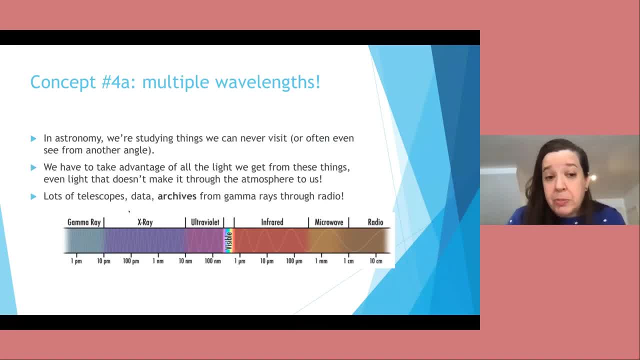 data, as I've already mentioned, comes from multiple wavelengths, because in astronomy we're studying things we can never visit Or even turn around and see from a different angle. So we have to take advantage of all the information that we get from these things, even the light that we can't see, even the light that doesn't make it. 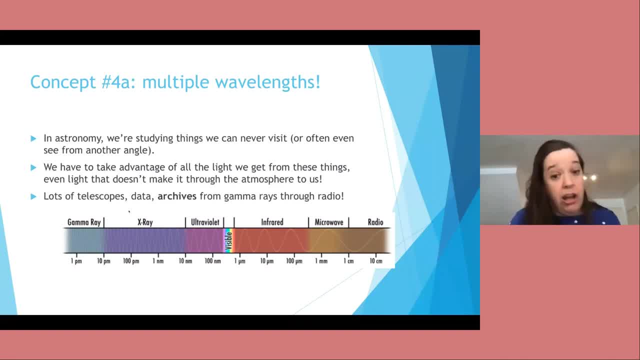 through the atmosphere to us, And so there's lots of telescopes, data and archives that house astronaut astronomical data, from gamma rays through radio, but their conventions can be very different, The units that they work in can be very, very different, And at IPAC, where I work at, 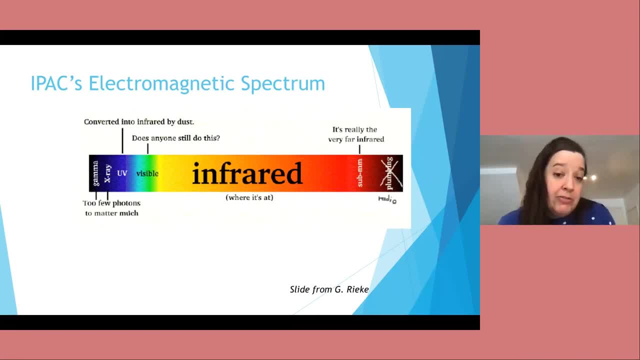 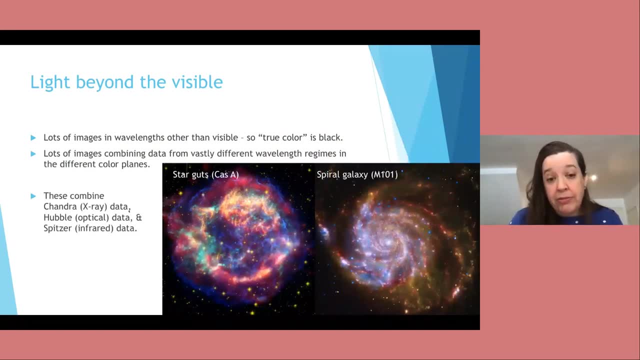 Caltech, we do a lot of infrared stuff, So we have a very biased view of the universe because most of what we do is infrared. So there's lots of images in wavelength other than the visible And of course, true color, for light beyond the visible is black, So that's not useful And so there's lots of 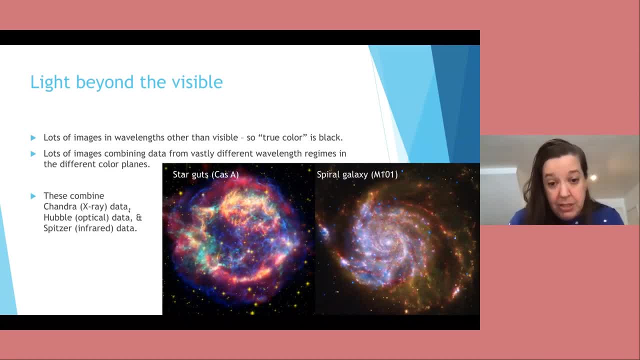 images combining data from hugely different wavelength regimes in the same image, So I've got two different images here. This one is an exploded star, So what you're seeing is all the star guts, And here's a spiral galaxy, And the three color planes in these images are combining x ray data. 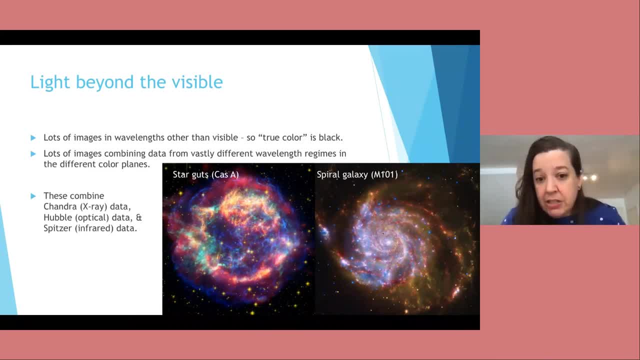 optical data and infrared data in one view, And so you can definitely see that there are things that are very, very bright in red or in blue that are not nearly as bright in the other band passes. So not. it also turns out that not every 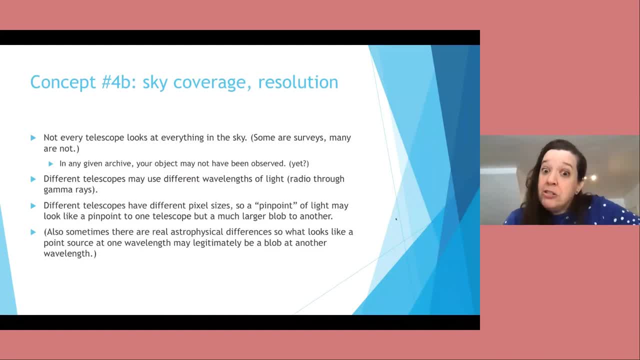 telescope looks at everything in the sky. there are some telescopes that are indeed surveys. they do look at the whole sky, or the whole sky that they can see from their ground base location, But many telescopes are not, And so if you were data mining in any given archive, 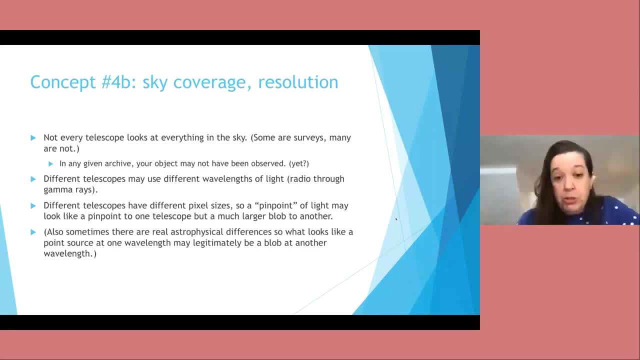 your object may not have been observed And that may be that because the telescope is too new, or it may be that that object is just not thought to be very interesting in that wavelength regime. So different telescopes are going to use many different wavelengths of light. 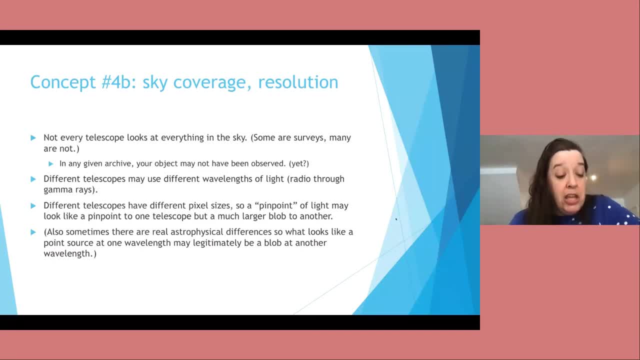 Different telescopes also, turns out, have vastly different pixel sizes. So something that is a pinpoint of light may look like a pinpoint to one telescope but a blob to another, And sometimes that's real astrophysics. Sometimes there's real astrophysical differences, So something that's a 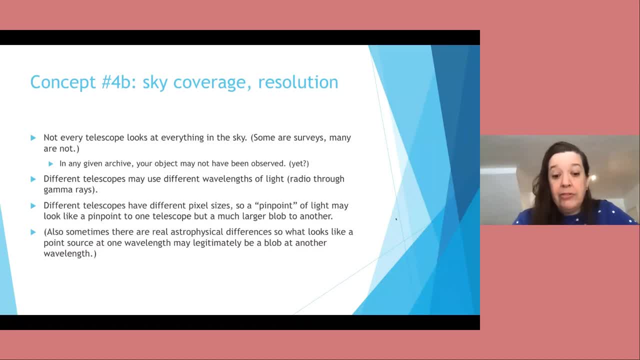 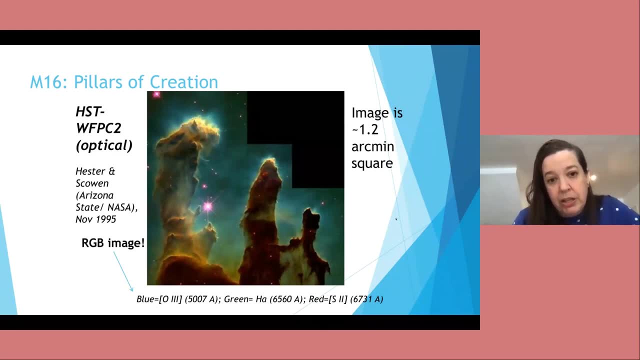 point: source at one wavelength is legitimately a blob at another wavelength. So here's some examples. The Hubble image, the most popular image downloaded from the Hubble website. it's called the pillars of creation And what's happening is there are some bright stars in this view, above the image. 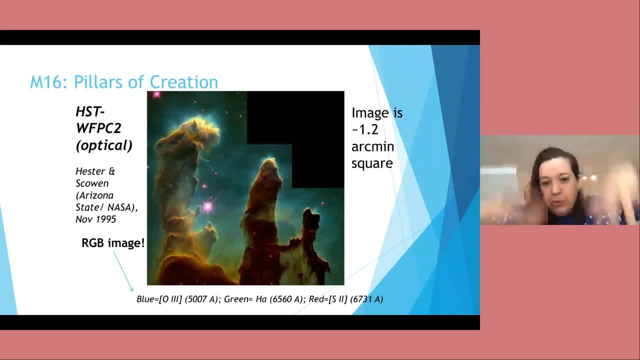 that we've got putting out so much radiation that it's pushing the gas and dust around, And so you end up with these fingers. These fingers, it's an M16- is the Eagle nebula, So these are the talons of the eagle in the Eagle nebula, And so this particular image is an RGB image where I've got 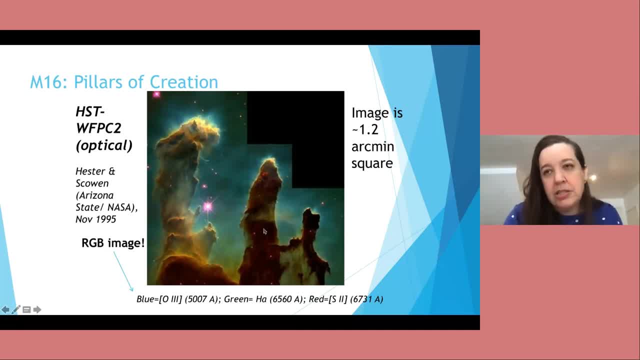 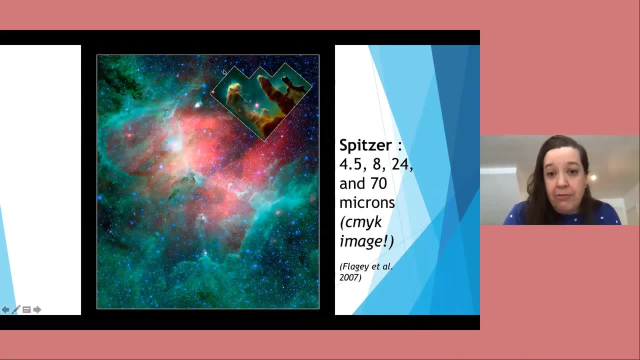 three optical bands So you can see the talons of the Eagle in the Eagle nebula And I'm going to contributing to this image. But this image, it turns out, is really tiny because Hubble's field of view is really tiny. This is the Spitzer view. Here's that funny footprint. There's the funny. 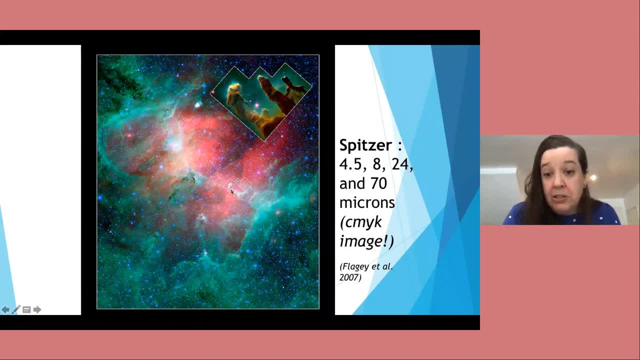 footprint on that Spitzer image And you can see it looks totally different. This particular Spitzer image is a CMYK image, So there's four channels And it's not optical at all, It's all infrared. So the shortest wavelength is 4.5 microns and longest wavelength is 70 microns here, So that 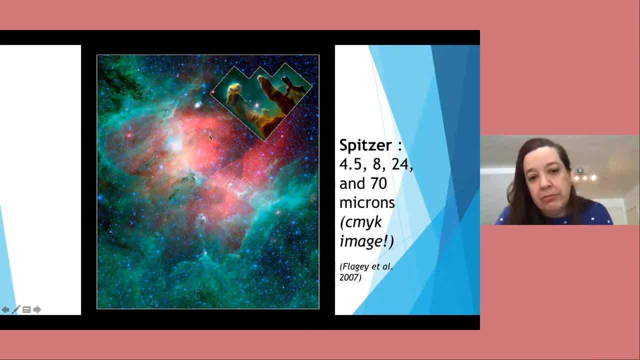 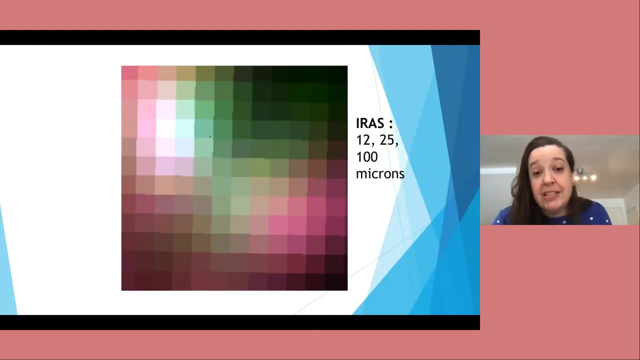 red there is 70 micron data. Now this image. I swear to you it's lined up. If I flip back and forth, you can see that there's definitely things in this image that are also there. But this is a much older mission. This is the first infrared all-sky survey taken with a 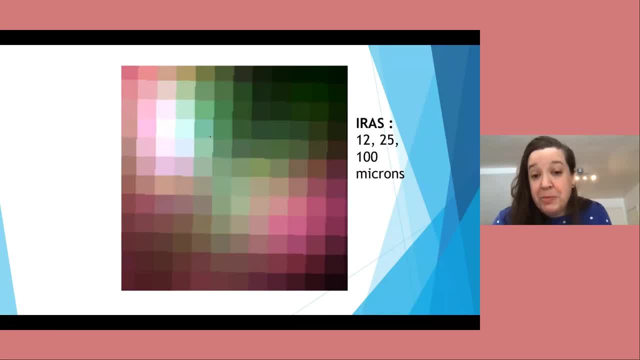 satellite called IRAS, And so the pixels were huge because the technology was new, And so in this case, it's the technology that's different. The technology here is the infrared all-sky survey, taken with a satellite called IRAS, And so the pixels were. 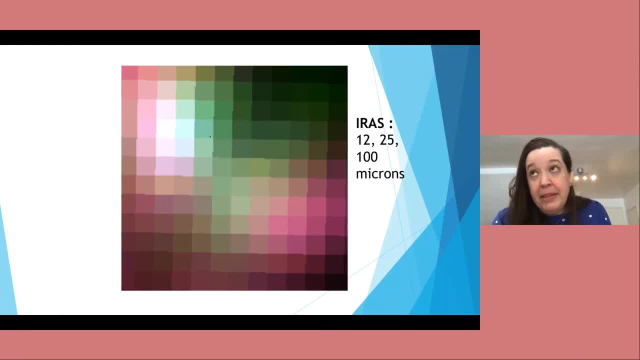 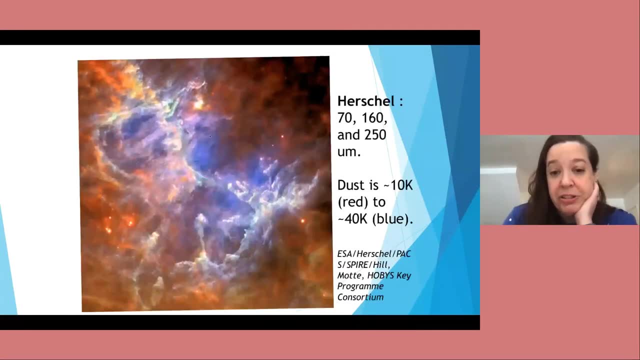 much more modern than the technology here. So here, going back to the Spitzer image, now I'm going to flip back and forth between Spitzer data and Herschel data. So for the Spitzer data there's 70 microns is red. For the Herschel data, 70 microns is blue, because it's the 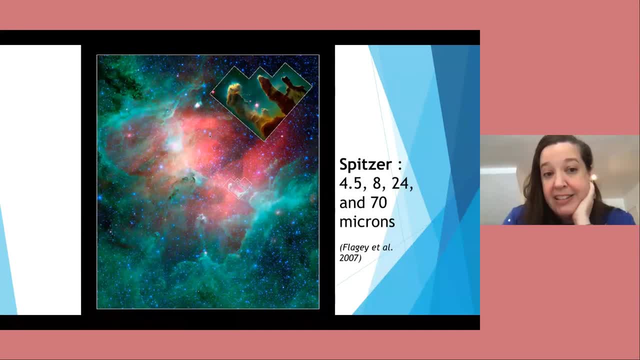 shortest wavelength shown In the Spitzer image, you see lots of blue dots. Those are all stars. Here there are very few stars, It's mostly dust that you're seeing. So it's very, very different. You're looking different astrophysically because you're looking at 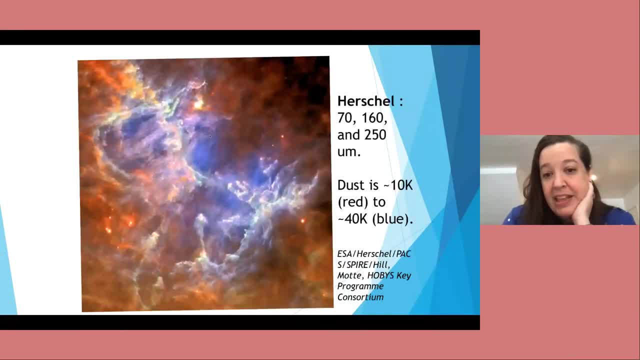 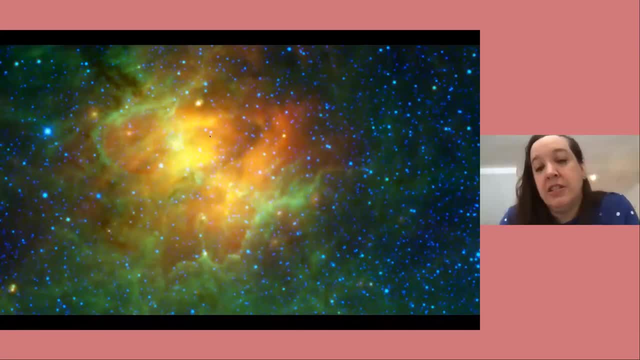 different things in this nebula, And then the Herschel data is lined up here with another image. So this image is from WISE, which is another all-sky infrared survey, And the resolution is not great. Here you can see lots of details. Here the resolution is a little bit poorer. 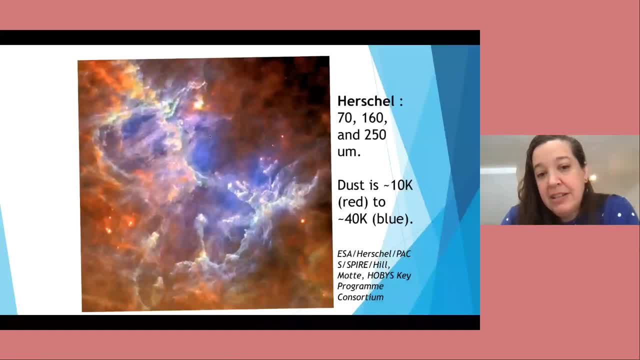 Here the resolution is much worse, But here that's pretty much all the Spitzer data there are for this region. It's pretty much all the Herschel data. So here you can see lots of details. Here the Herschel data there are for this region, But WISE is an all-sky survey So the data don't. 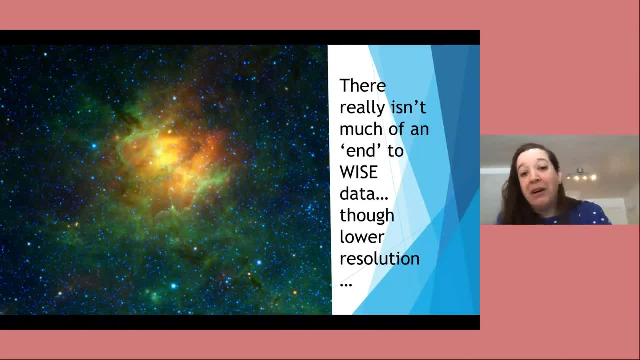 really end. There really isn't much of an end to WISE data, because it covers the whole sky. It's lower spatial resolution, but it covers the whole sky. So that's usually the trade-off And so you're going to see when you start poking around in these different data archives, there's 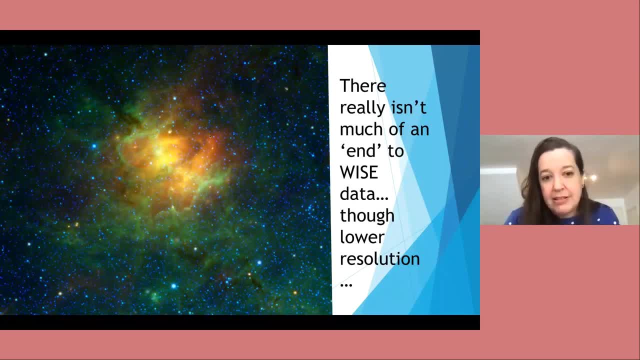 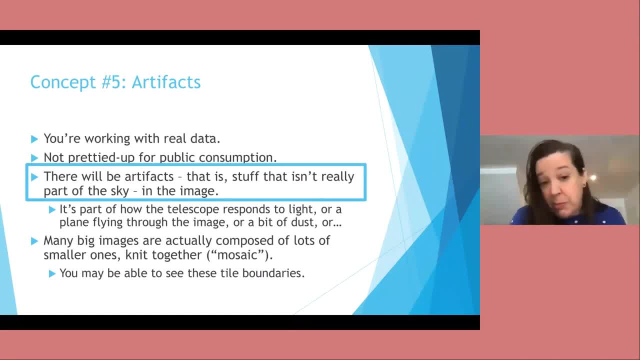 big concept is artifacts. So the last big concept is artifacts. So you're working with real data when you get into these archives. It is not going to be printed up for public consumption, So there's definitely going to be artifacts in those images. That is stuff that's not really part of the sky. 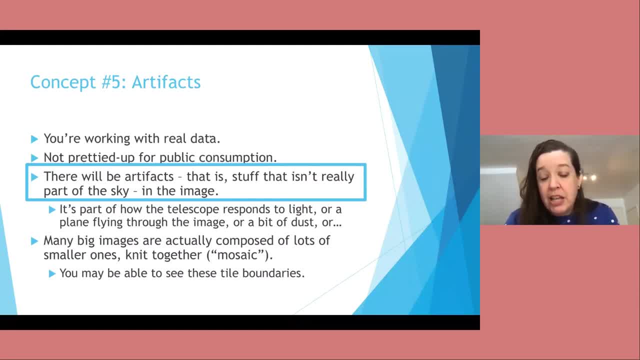 that you can see in the image And it's just how the telescope responds to light. Or if you're looking at ground-based data, maybe there's a plane flying through the image or a bit of dust on the telescope. You know, all of that could be the case, And when you have really large images, 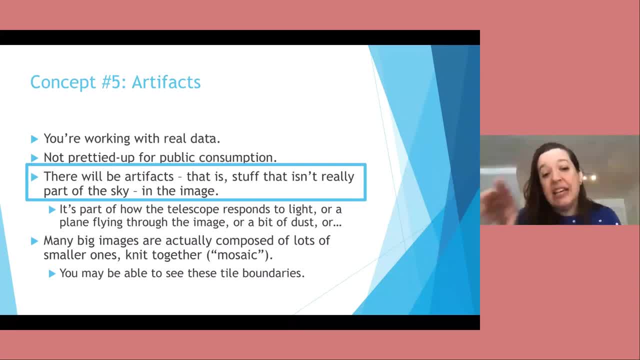 they're actually composed of smaller ones knit together or mosaicked together, And you may be able to see these tile boundaries. So when you have really large images, they're actually composed of smaller ones knit together or mosaicked together, And you may be able to see these tile boundaries. So 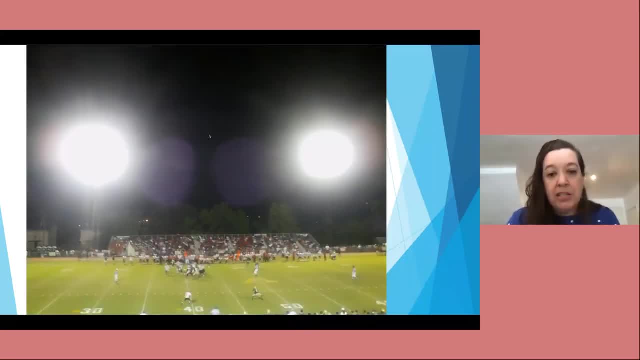 you already are familiar with this concept, even if you don't know it. So this image I don't know if you can see on your screen, but it's a high school football game, And the bright lights are these huge fuzzy blobs with these weird purple appendages coming off of both of these bright 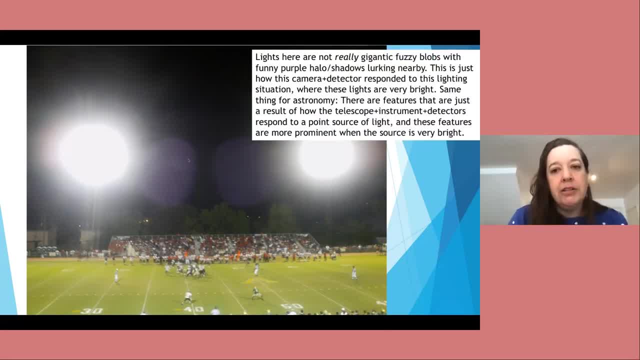 lights. You know intuitively that the lights here are not really gigantic fuzzy blobs with these funny purple halos lurking. That is just how this camera and the digital detector responded to this lighting situation, Because these lights are very bright And the person 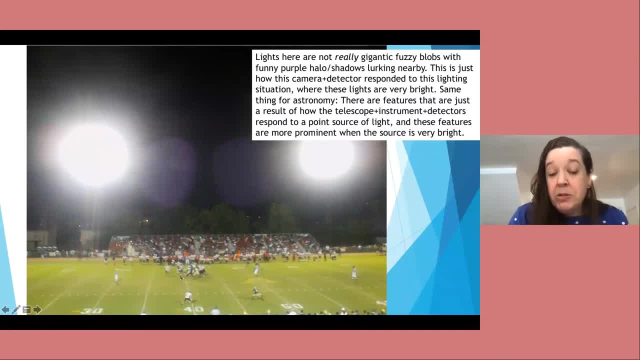 taking the picture was trying to take a picture of the football game, So it's just the way that this camera is responding to these bright lights, And so the same thing is true of astronomy: There are features that are going to be there just because it's a really bright source of light. 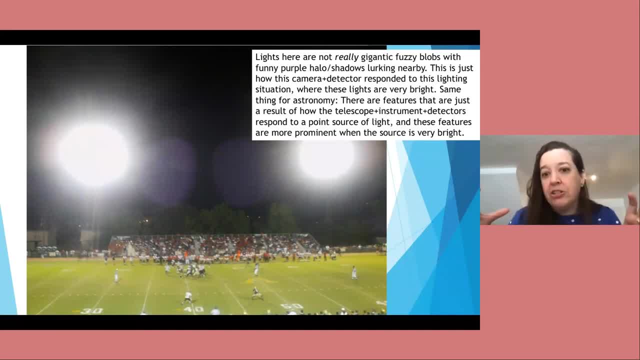 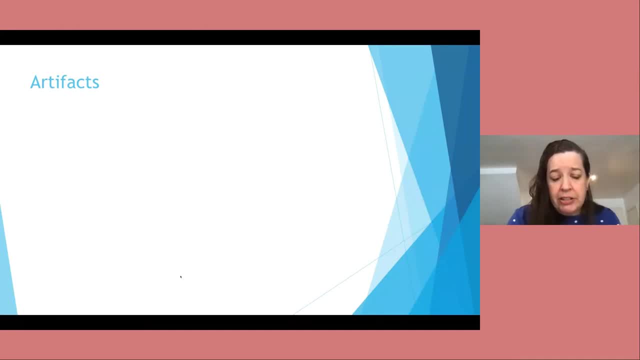 Or the feature. you know you end up with all of these artifacts showing up much more prominently when the source is very bright. So let me just point out there's a Neil deGrasse Tyson is on the Stephen Colbert show a lot, And Stephen Colbert 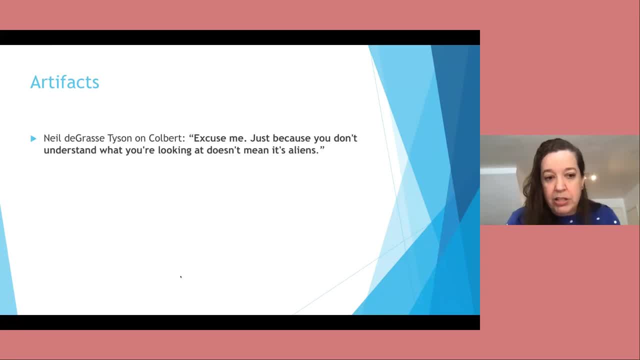 was very excited about some of these results And he wanted to push Neil deGrasse Tyson on what it meant And he cut him off short with excuse me, just because you don't understand what you're looking at doesn't mean it's aliens. So if you find something that looks weird in the data, 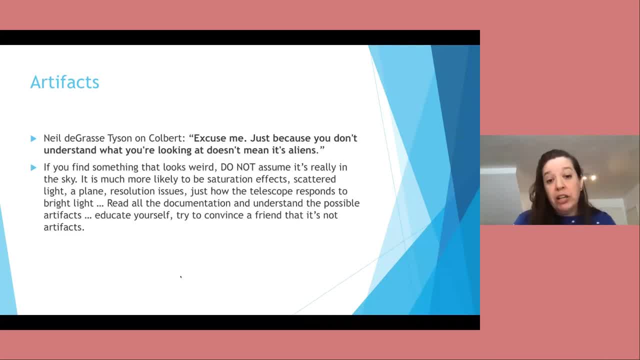 please do not assume it's really in the sky. It's much more likely to be saturation effects or scattered light or a plane or spatial resolution issues Or how the telescope responds to bright light there's. you're gonna need to get in and read the documentation. 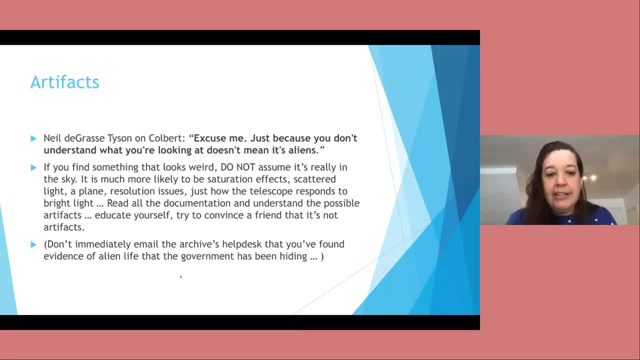 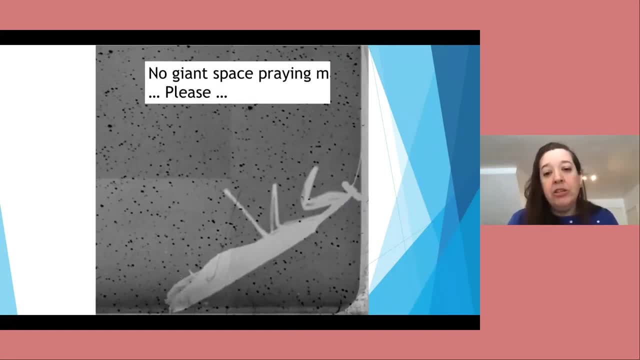 You know. please do not immediately email me and tell me that you found evidence of alien life, because that's not the case. There's gonna be lots of artifacts. please do not call me and tell me that you found giant space praying mantises. 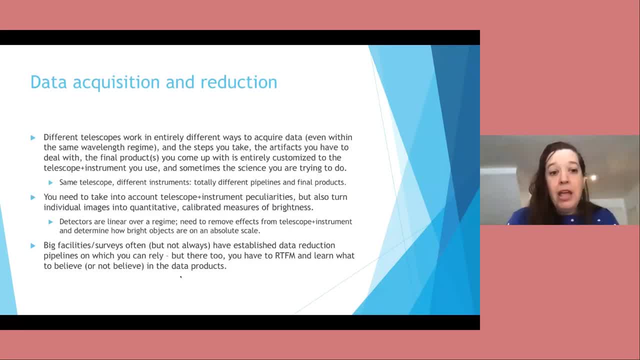 There's all sorts of interesting artifacts that will show up in the data, And so when you're, when you're acquiring the data in space, different telescopes work in entirely different ways to acquire data. even if you're working with the same wavelength regime, the telescopes are going to work. 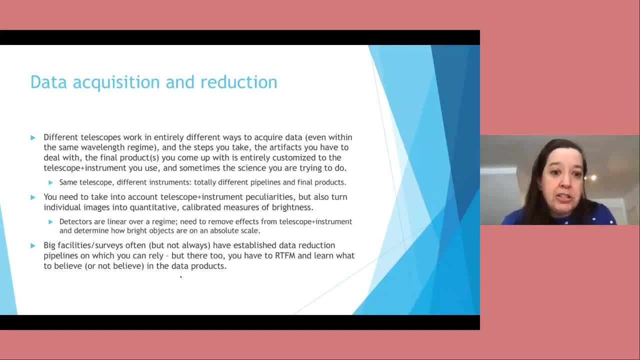 entirely different and the steps that you take, the artifacts that you encounter and the way that you get to that final product isn't going to be entirely customized to the telescope combination combined with the instrument, and sometimes it's going to be strongly influenced by the science that you're trying to do. so you can have the same telescope and different instruments and have 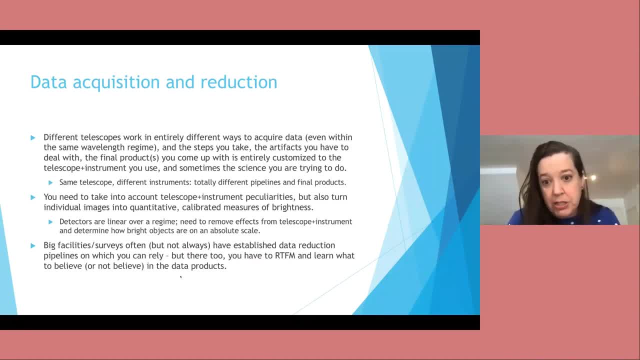 totally different pipelines, totally different software packages to reduce the data and turn it into a final product. so you need to take into account the you know the telescope and instrument peculiarities, but you also need to turn those images into a quantitative measure of the brightness. and that is not trivial with your camera: you can just take a picture and tra la la. 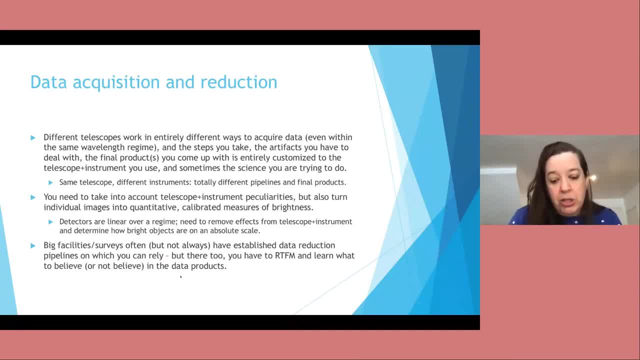 you've got a picture and you can move on your way. but in astronomy you need to be much more careful. you need to much more carefully understand how the detector is responding. what is effects from the telescope or the instruments? what is effects from the detector? and remove that and calibrate the data so that you know how bright. 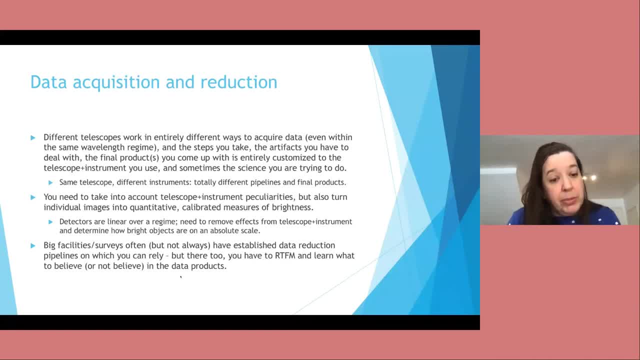 objects are on an absolute scale. so a lot of the really big facilities or surveys have an established pipeline that you can rely on. but you have to read the documentation that are provided and learn what you can believe or not believe in the data products. because all of these 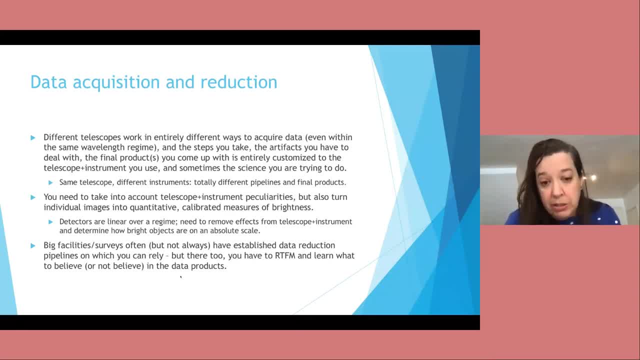 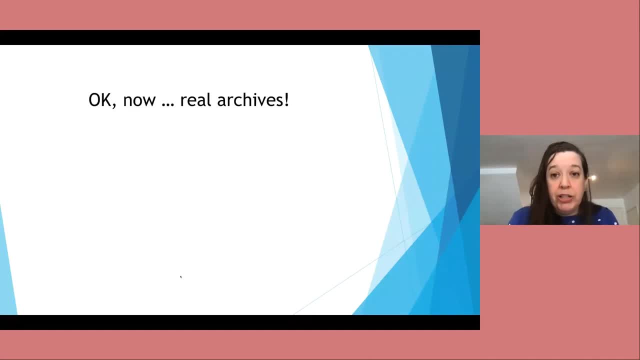 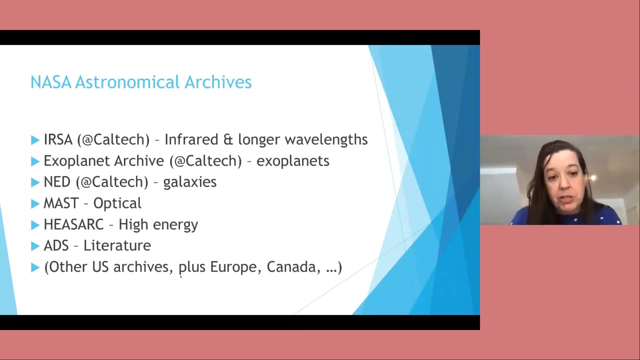 facilities and surveys are going to have documentation- copious documentation that goes with it. that explains what you can believe and not believe. so now i'm going to talk about some real archives and get into more of a demonstration. so nasa has many astrophysics archives. ursa, which is based at caltech, which is where i work, is nasa's home. 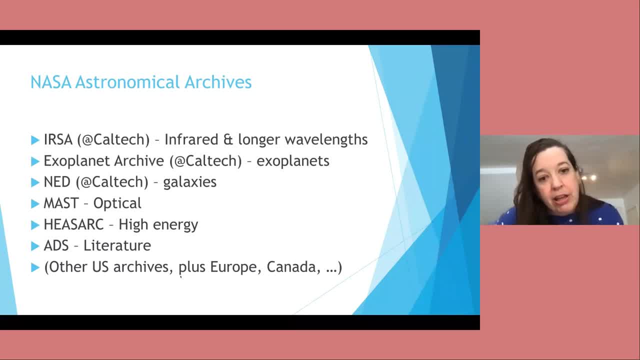 for infrared and longer wavelength data. we also have it at ipac at caltech, something called the exoplanet archive, which unsurprisingly focuses on exoplanets. ned is the nasa extragalactic database, which is also at caltech and that specializes in galaxies. mast, which is based at the space telescope. 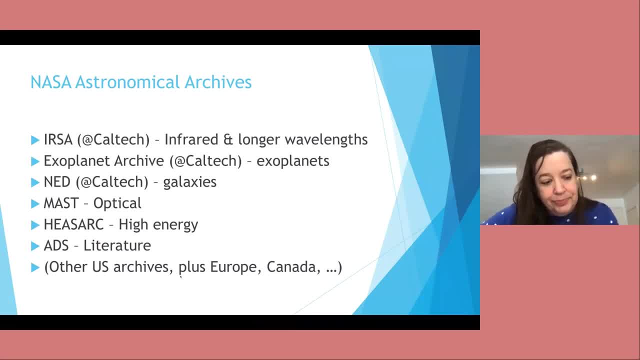 in baltimore. maryland is nasa's home for optical data. he is sarc, which is based at nasa's goddard space flight center in um greenbelt. maryland focuses on high energy astrophysics data. ads, the astrophysics data system is based at harvard in cambridge, massachusetts, and that 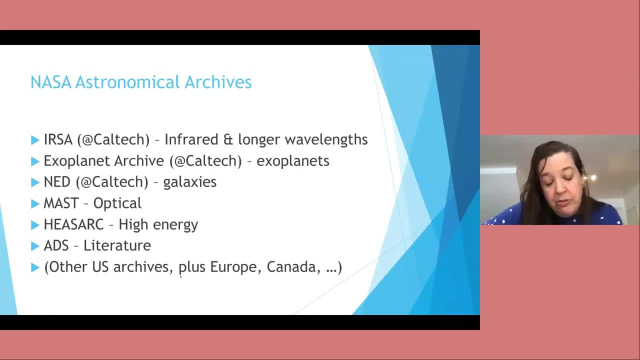 focuses on literature. that includes all of the astronomy literature from the 1800s through this morning, and it's all there and it's all freely available and you can dig into it at your leisure. there's other us archives um that, but those are. these are all the nasa archives and there's more. 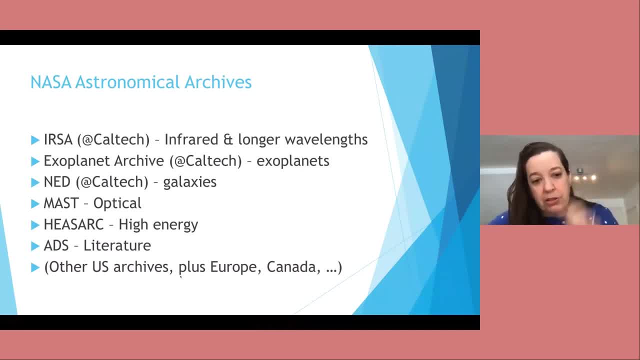 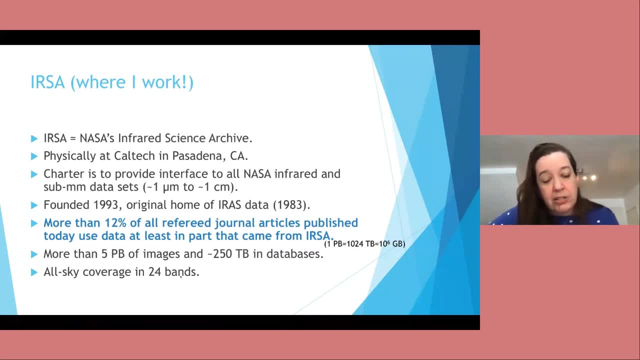 archives in europe and canada and elsewhere, but these are the the nasa astrophysics archives. ursa, where i work, is nasa's infrared science archive. that's what ursa stands for physically. i'm based at caltech in pasadena. our charter is to keep track of all of nasa's infrared and 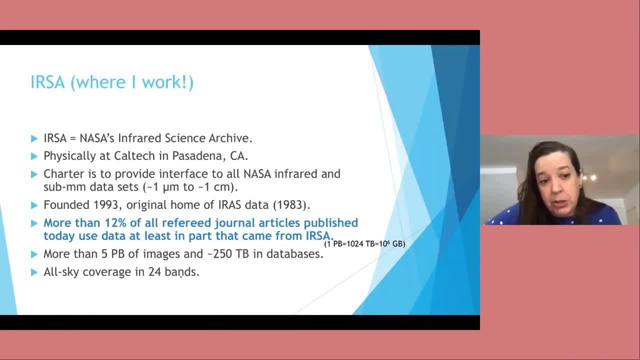 sub-millimeter data sets, so we're talking wavelengths between a micron and a centimeter. we were founded in 1993 originally to be the home of the iras data. the iras was that first all-sky infrared survey that was taken in the 80s. more than 12 percent of all referee journal articles that are published today. 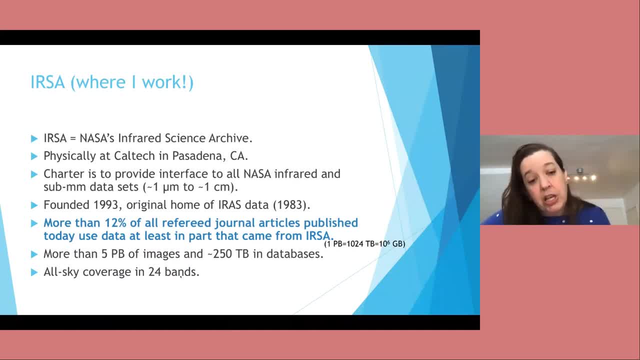 use data, at least in part. that came from ursa. we currently have more than five petabytes of images. remember that a petabyte is a thousand terabytes or a million gigabytes and there's 250 terabytes in databases and counting. we have an all-sky coverage and 24 different long wavelength. 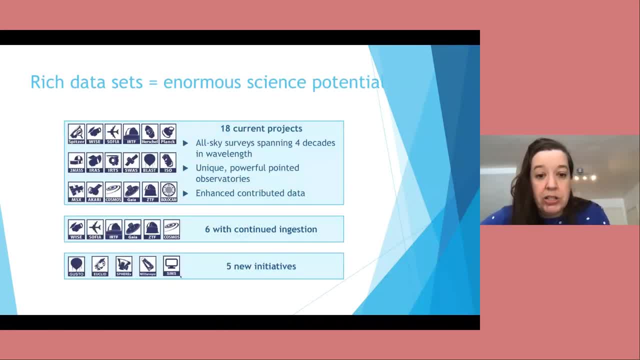 so we have huge amounts of data. we have 18 current projects that are either the data are already done and it may be reprocessed, or they're actively being added to. there's actively more telescope, more telescope usage, more data being collected. there are six projects that are ongoing continued data ingestion and there are five new initiatives. 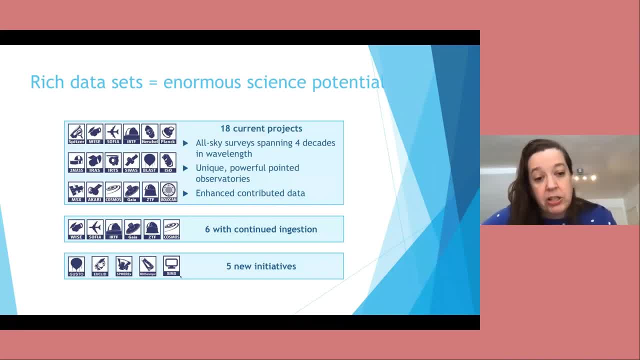 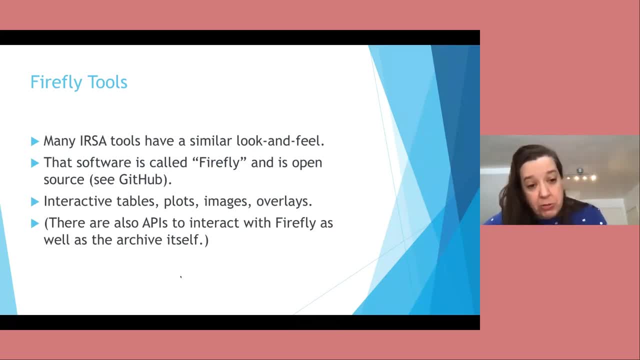 that we're planning for more spacecraft that are on their way to launching in the next few years. so many ursa tools have a very similar look and feel, and that software is called firefly. it is open source. if you look on github, you can find this um. it provides interactive tables and 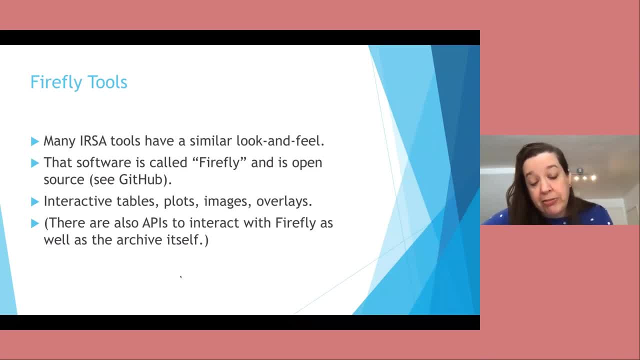 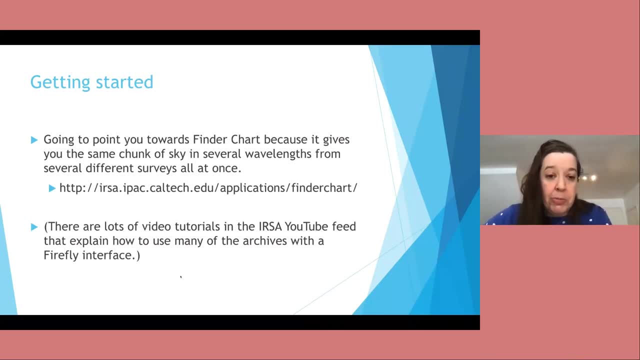 plots and images and overlays, and there are apis to interact with firefly, as well as all of the archives that we have itself. so i'm going to point you towards a tool called finder chart, because it gives you the same chunk of sky in several different wavelengths from several 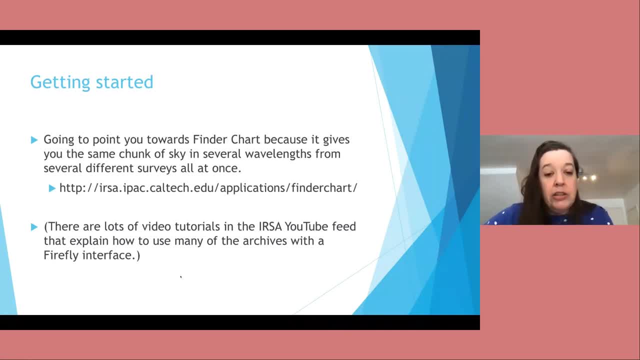 different surveys all at once. that's the link right there. there are lots of video tutorials in the ursa youtube feed that explain how to use the archives that have a firefly interface, so let me quit out of this. um, you can still see my browser right, it's on the ursa home. 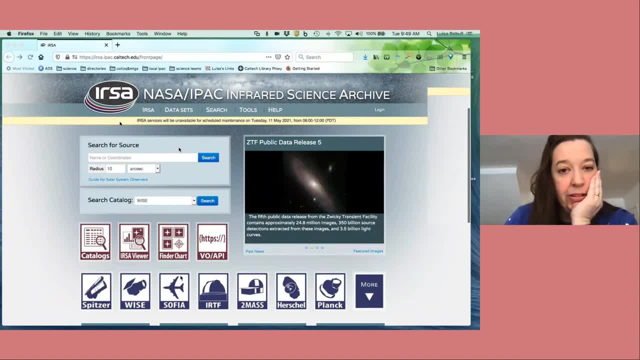 page. yes, hopefully you can see it okay. so, um, if you just put in a source name there, it'll give you a list of all of the data that ursa has. that overlaps that position, but it's um, it's maybe harder to understand that for a new person, so i'm going to recommend you go to finder chart. 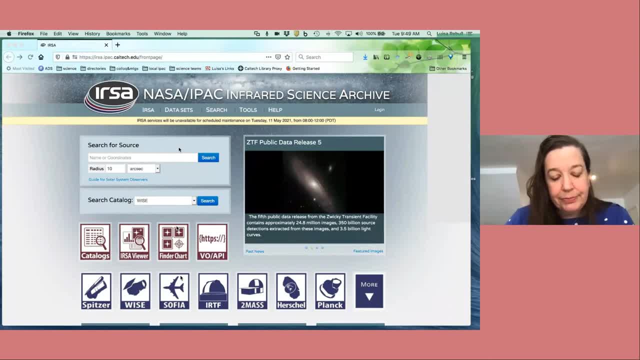 which is this one right here. so if you click on finder chart, it launches this tool and the very first thing you want to put in is the coordinates or the object name. i'm going to put in m16, which is the eagle nebula. now you can see that i've put in a name and it's turned it. 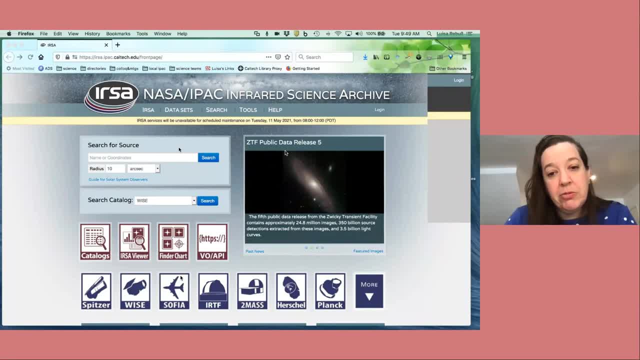 into coordinates. there's two different ways to do that. either one is fine for most purposes. then you want to put in the image size that you're asking for. you need to pick units of arc seconds, arc minutes or degrees. i'm on a laptop right now, so i'm going to leave it on. 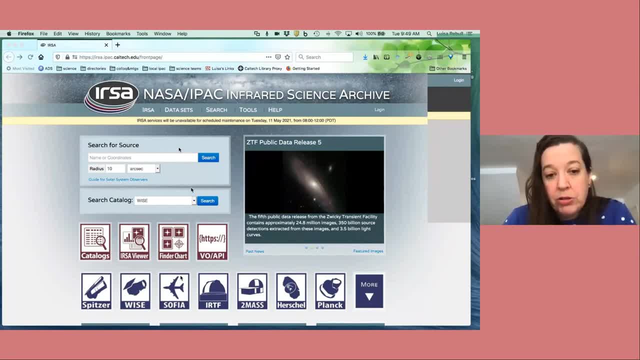 the medium display size. but you may if you have a big monitor, one large, or if you're on a really small laptop. you want might, want small. then the next thing is you want to select your images. there's many different archives that are here, so let me go back to one slide from the powerpoint. 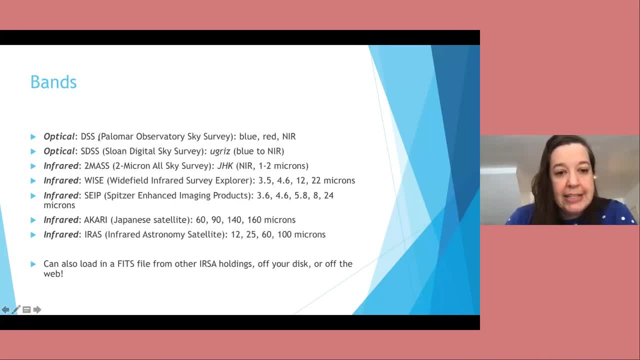 so there's several different bands. optical is the dss, the digital sky survey. it actually turns out that you can see that the dss is a digital sky survey. so if you take a look at the dss, this is the dss of the alamar observatory sky survey. so this is data that was taken. 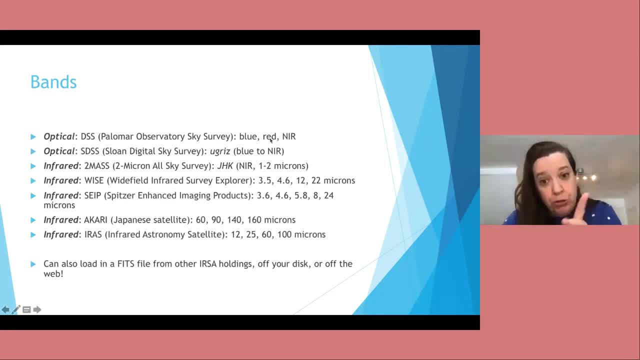 in the 50s on photographic plates and then scanned in, digitized later. and those bands. there's two blue lands, one, two blue, two blue bands, two red bands and one infrared, one near infrared band. you can also get to the optical sloan digital sky survey, or sdss, that is a ground-based telescope. so 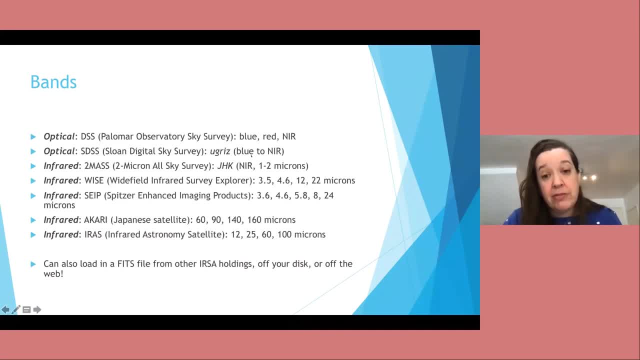 they can only do the northern hemisphere, they didn't do the whole sky even in the northern, from blue to the very near infrared. And then there's several different infrared surveys. The 2MASS is the two micron all sky survey. That's near infrared, so between one and two microns. 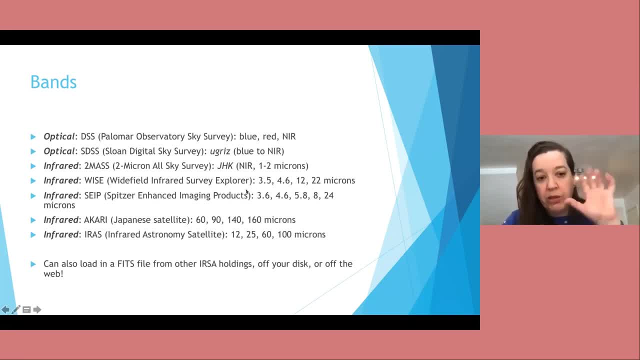 There's the WISE Wide Field Infrared Survey Explorer. That's one of the surveys that I'm talking about. that does the whole sky And that's between three and a half and 22 microns. There's also the SEIP. 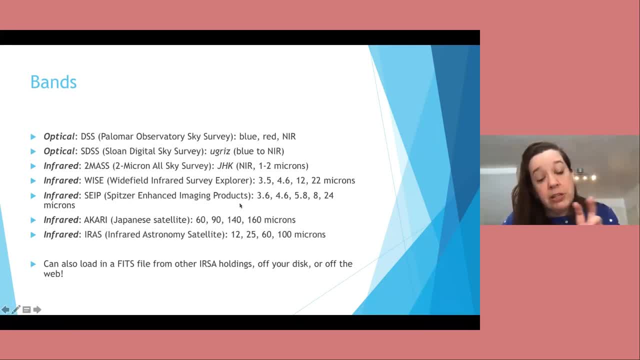 which is a Spitzer Enhanced Imaging Product. Spitzer was a pointed observatory and it observed in many different bands, but this particular processing covers three and a half to 24 microns And again, not the whole sky, but the most popular pieces of it are in there. 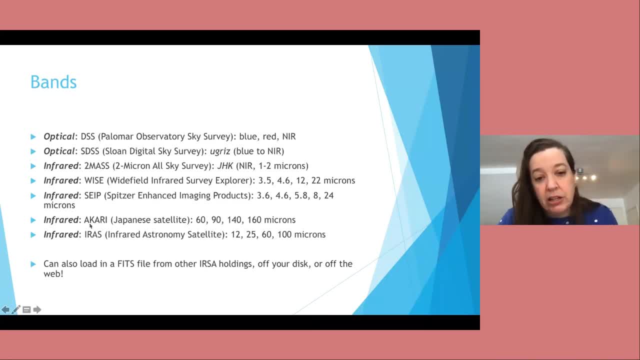 In the infrared also. there's a Japanese satellite called Akari, and it observed between 60 and 160 microns. And then there's good old IRAS, which was the first all sky infrared survey And that observed between 12 and 100 microns. 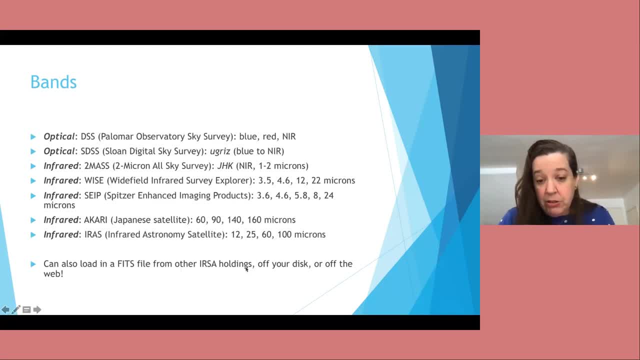 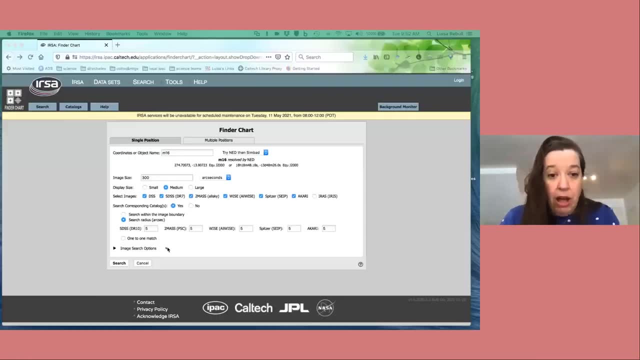 If you got a FITS file from someplace else, from other URSA holdings, from a telescope that you have access to, or an image that you found on the web, you can also load it in there. So I'm gonna go back here for M16.. 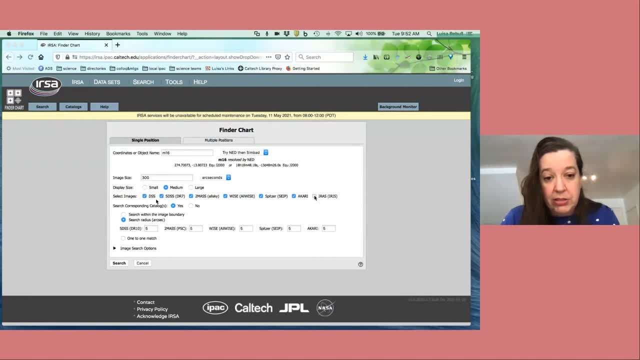 I'm gonna select all of the surveys, So optical is here, then infrared out to here, And for this point, when you're starting out, I strongly recommend turning off the catalogs because it can become very overwhelming, very, very, very quickly. 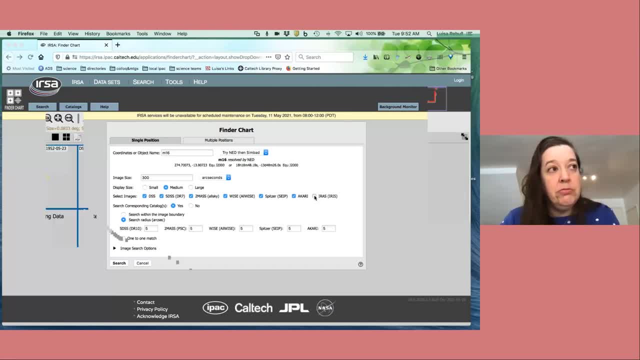 So then I'm gonna go ahead and hit search and it's gonna go do it. It's going to go pull the same chunk of sky from each one of these surveys And it's zooming around here as it's loading in the additional images. 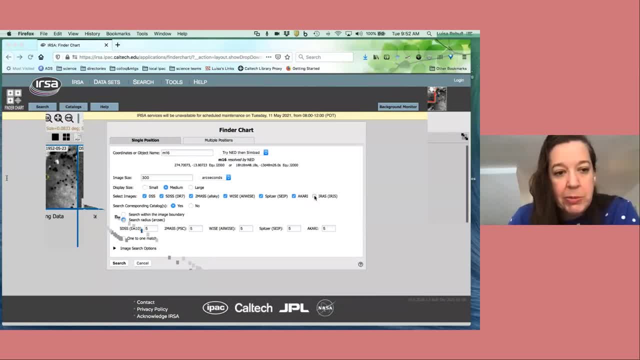 So here is a row of optical DSS. Remember that scanned photographic plates. So the date here- 1952, is this is when that photographic plate was taken And this photographic plate was taken. Then in 1984, they did some additional photographic plates. 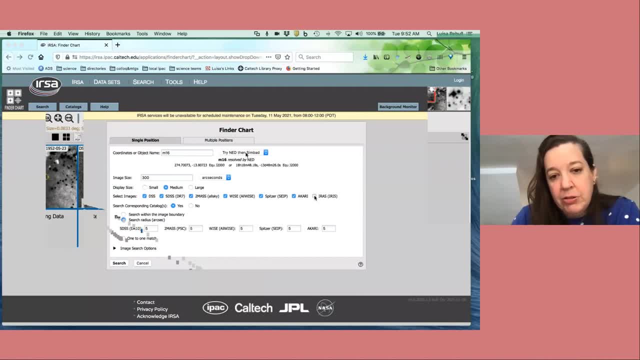 Photographic surveys, And in the near-infrared there's one from the 1980s, And so it was all digitized in the 90s and made available. So this is all in reverse gray scale. Let me keep going through the data. 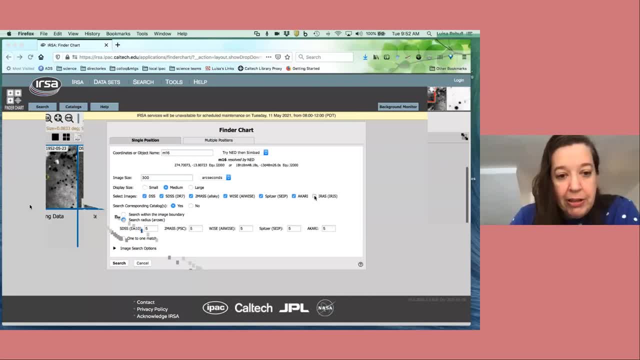 then I'll go back and do the gray scale. This is the near-infrared, this is 2MASS. There's WISE. So between WISE 1,, which is 3 1⁄2, to WISE 4,. 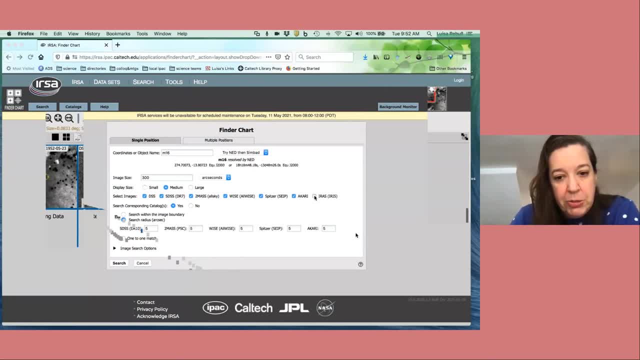 which is 22 microns, And then there's the Spitzer bands And you can see ACARI is not very high High spatial resolution And IRAS has giant honking pixels And Sloan didn't observe this region at all, So the default it's come up with is reverse gray scale. 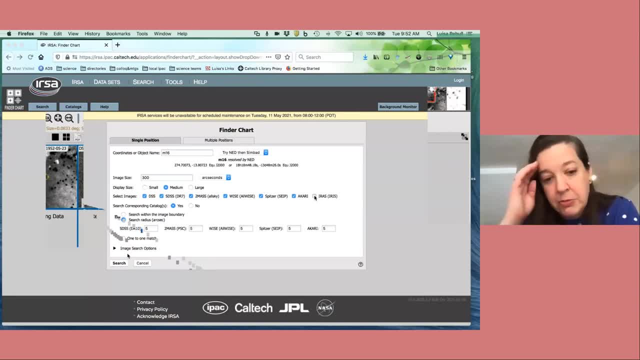 because that's how most astronomers are used to interacting with images. So things that are bright are black and things that are dark are white. So you can see that, those talons of the eagle you can see even in the photographic plates, And by the time you get out to the infrared. 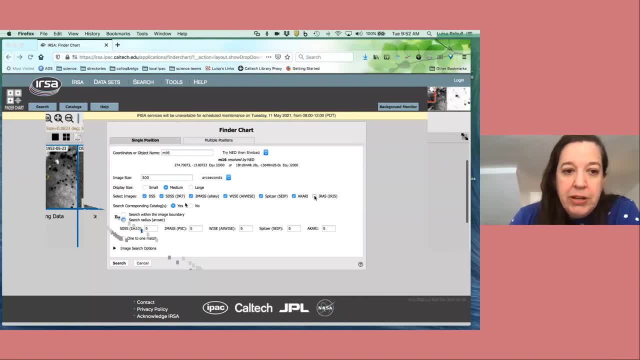 those talons can be quite prominent. But if you want to change the color table, you can. You can change it to be whatever you want. There's lots to choose from here- And then you can also change the color stretch. Here's a histogram of the values found in the image. 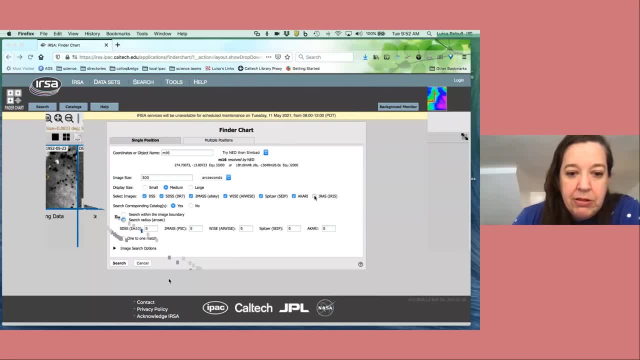 that's selected, which is this one, because it's outlined in orange. Let me pick a different one. Let me go there So that one is outlined in orange. So there's a histogram of all. Yeah, So I don't see this. 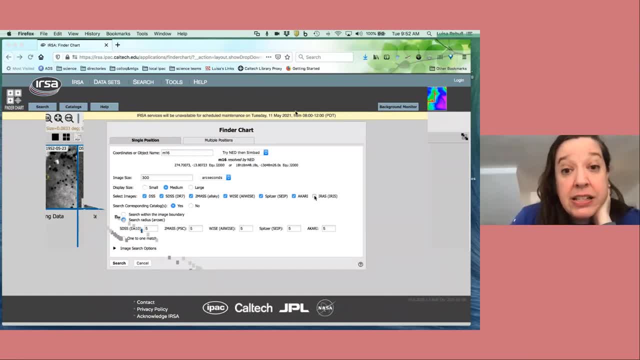 I don't see the histogram. I don't know if other people can I see it- with the coordinates of objects and things. Take it, But I don't see the graphs that you're sort of predicting Interesting. OK, yeah, I haven't worked with the big marker interface. 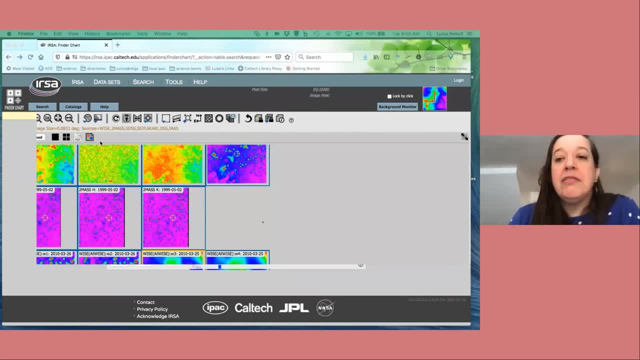 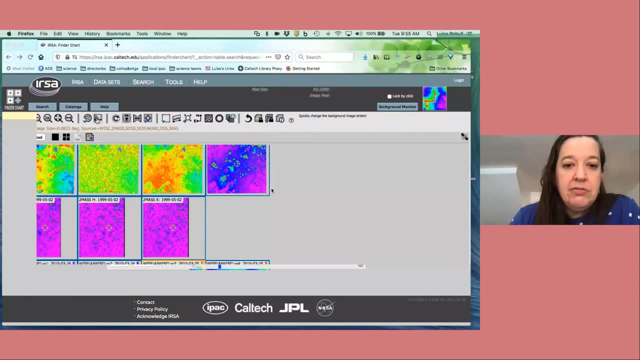 before. Zoom will show it to you. Now it's showing up. Now it's showing up. OK, It's just How bizarre. OK, can you see it now? Did it work now? Yeah, OK, So you can pick different stretches. 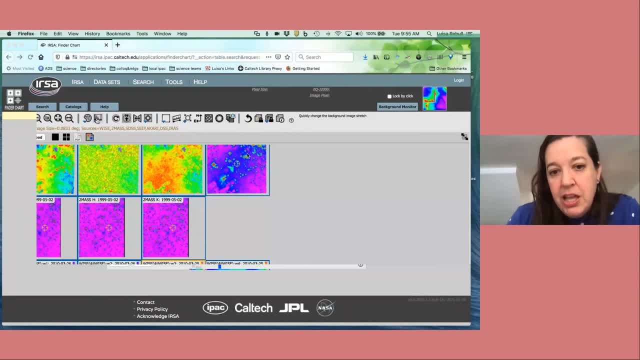 And it'll show you the histogram of the values And, given the color table that you've picked, it'll show you which value is which color, And you can, in this case, the default is showing you everything between 1% and 99% of the data. 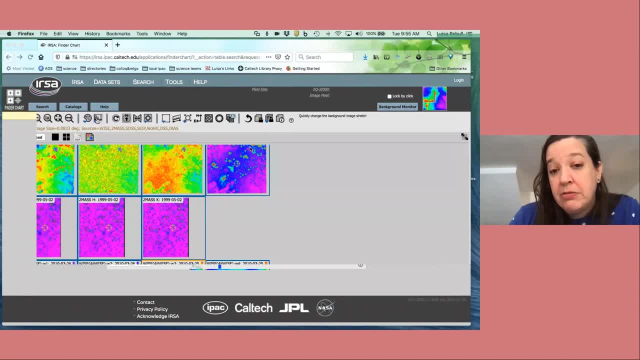 But you can change that depending on what details you want to bring out in the image. Let's see, Oh, let me put this back to reverse grayscale. Now this button right here, it's got a color, It's got a red, green and blue dot. 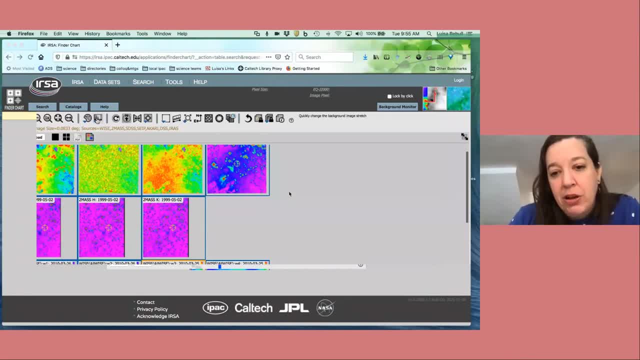 If you click on that, it will add at the end of each row a three-color image assembled from the data in that row, so that you can quickly and easily see what a color image might look like when you combine some of the data from that row. 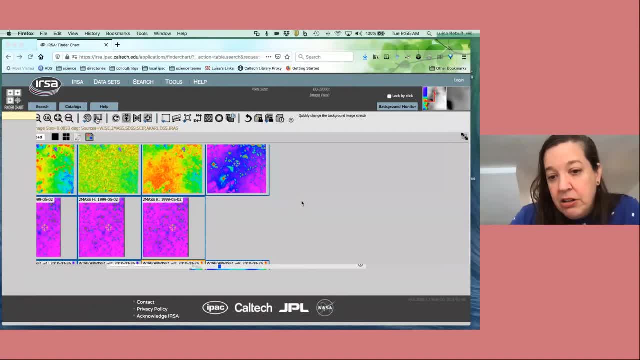 The crosshairs, there are the colors that you can see. OK, OK, OK, OK, OK. That is the target that we asked for. To download the data, you click on Prepare download And then you can say whether you'd like the FITS files. 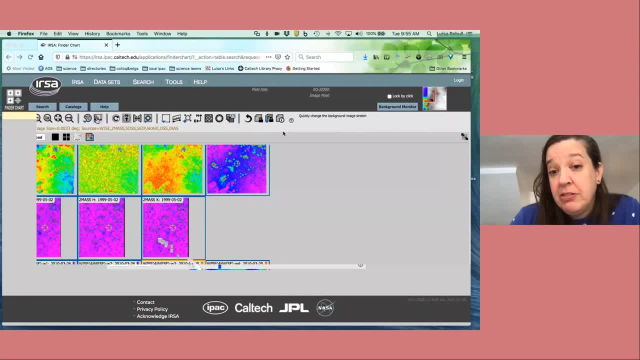 or you can save the HTML or a PDF version of it or PNGs. So the PNG is unlike GIFs or JPEGs. PNGs can be 8 bits deep, but you can also make them 16 bits deep, And so if you pick PNGs, it will try. 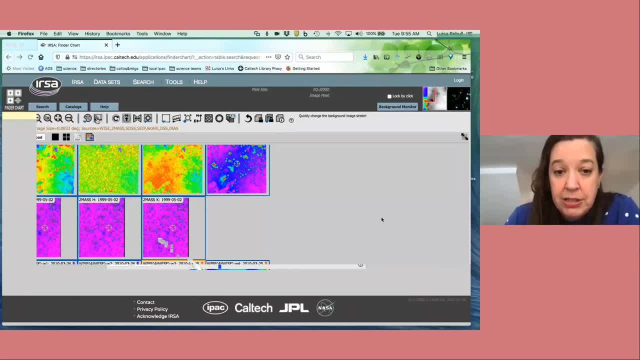 to preserve the things that you're looking at on the screen as you see them there, And you can save it to your local disk. And if you're downloading a lot of data, you may want an email notification and then it'll give you a script. 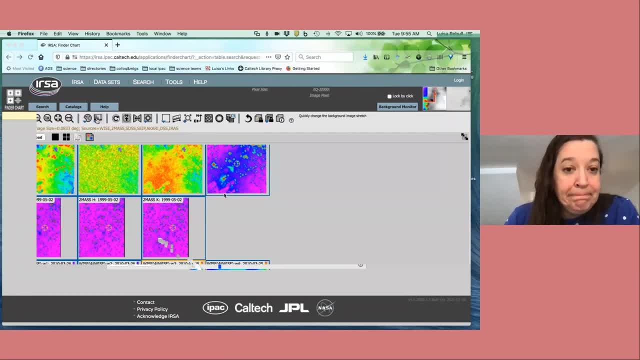 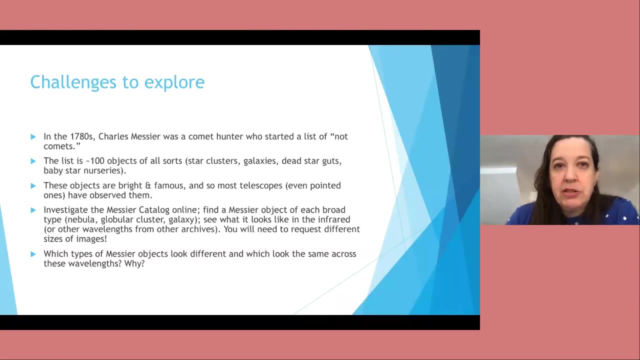 if you have many packages to download, What are the other? how are we doing on time? Let me step back to a couple of the slides and then we'll go back to doing some more demos and answer any questions you guys have. So here's a suggested challenge. So in the 1780s, a man by the name of Charles Messier- he was French, he was a comet hunter and he was tired of looking at things and getting excited that he might've found a comet, only to rediscover that no, that's not a comet. 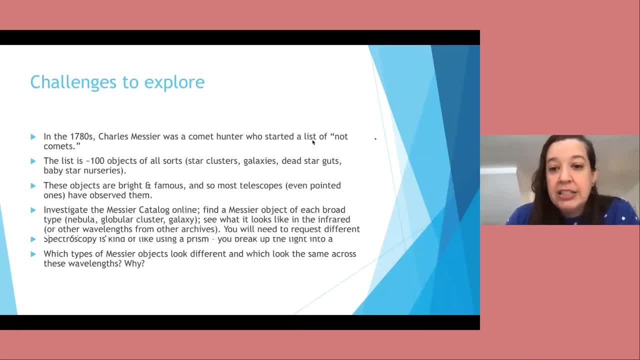 it's something else. So he made a catalog, a list- whoops, a list- of not comets, And he found some comets in the end. but what he's really famous for is this catalog, which is the list of not comets. 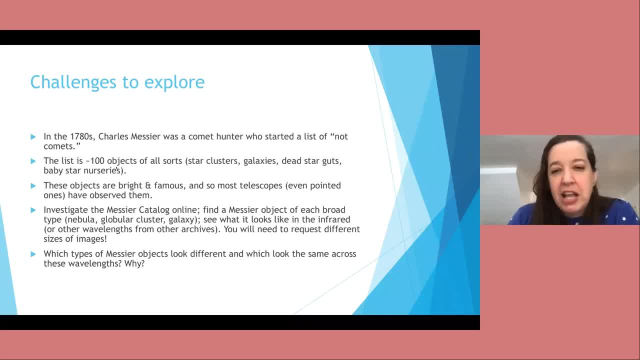 So the list is like 100, objects of all different sorts, clusters, galaxies, dying stars, star nurseries, all sorts of things, And these objects are all bright and famous. So most telescopes, even the ones that aren't, surveys. 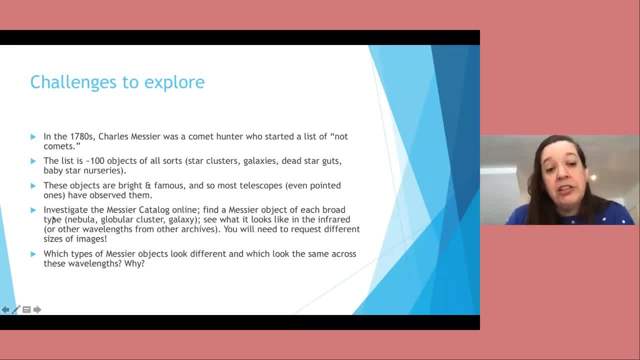 have observed them, And so one of the challenges that I'm suggesting that you do is go and do some research. find the Messier catalog Wikipedia page. find a Messier object of each type: a nebula, a globular cluster, a galaxy. 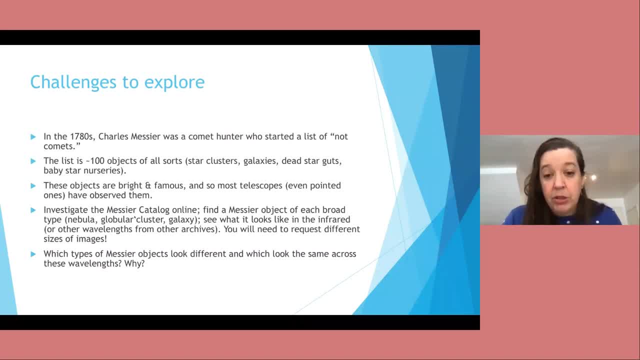 and then go and get the data in the infrared. You're gonna need to request objects of different or images of different sizes, because these objects are very different sizes, but you're gonna find that the Messier objects look different. Some objects are gonna look different. 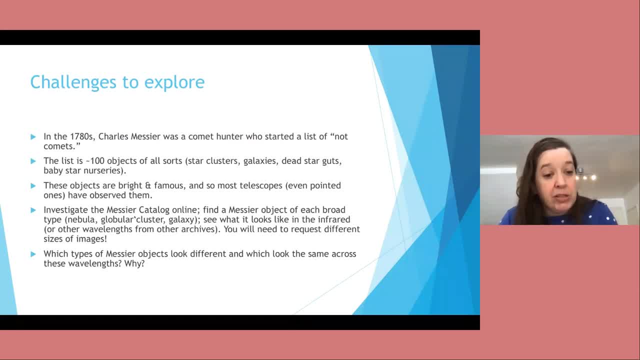 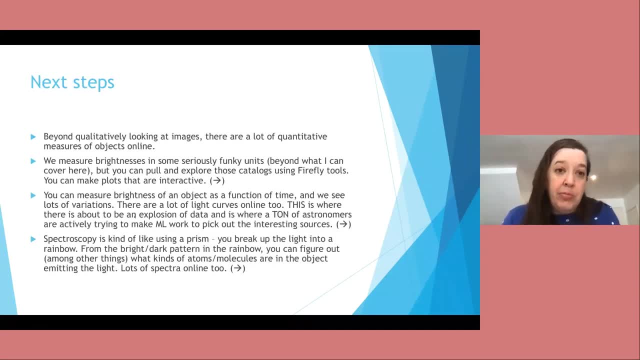 across many different wavelengths and some objects are gonna look the same across many different wavelengths. There's a lots of astrophysics in explaining why that is the case. So the next step: beyond qualitatively looking at images, there are a lot of quantitative measures of objects online. 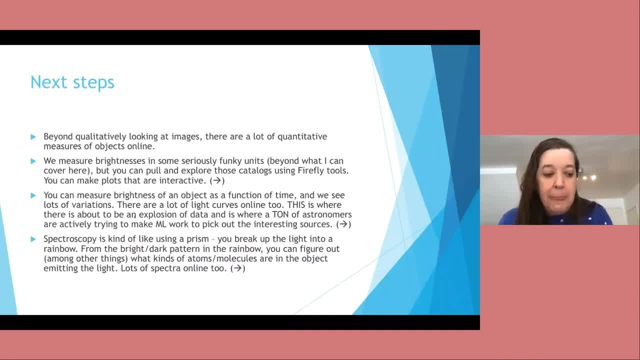 I don't have time to go through it in detail, So I just wanna give you some highlights. We measure brightnesses in astronomy in some very strange units, and that's beyond what I can cover here, but I've given you some links on that webpage. 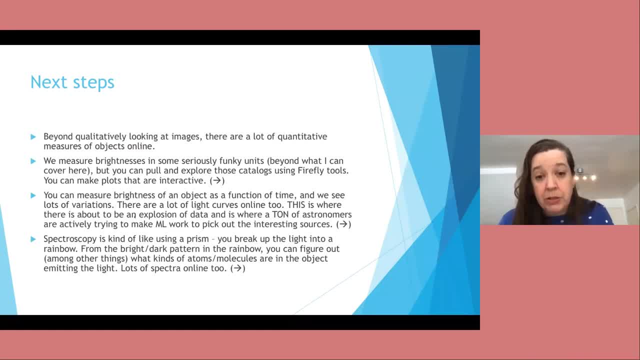 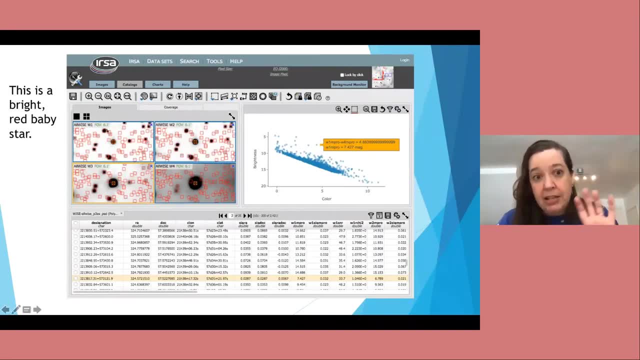 if you wanna get into more detail, But you can in fact pull and explore those catalogs using these Firefly tools and you can make interactive plots. So this is not finder chart, but you can see it has a lot of the same look and feel. 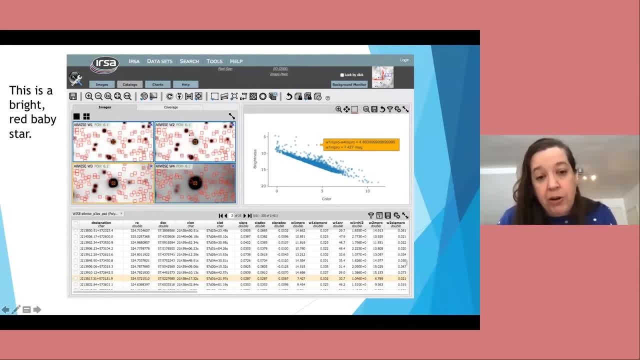 It's something called Ursa Viewer, And so I've loaded in four different infrared images here, I've loaded in the catalog and the catalog is over-plotted on the images here And I've made a plot which is brightness against color. 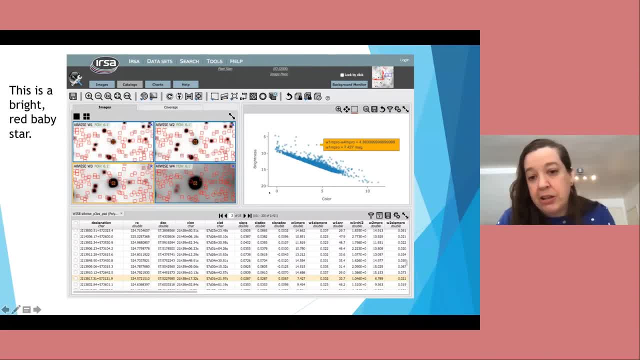 And so you notice I'm in some funky units here because the numbers are getting bigger towards the bottom, but it's the units that astronomers use. So this particular object, if I click on it in the plot, it's highlighted in the catalog and on the images. 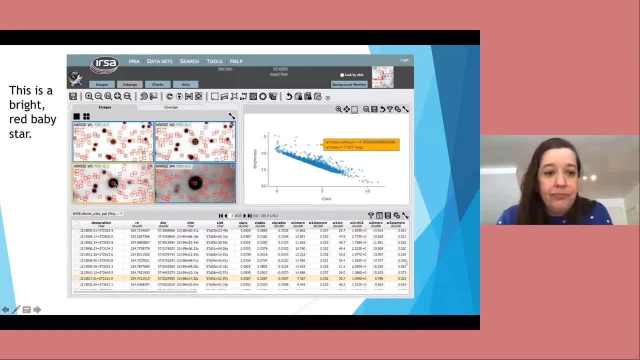 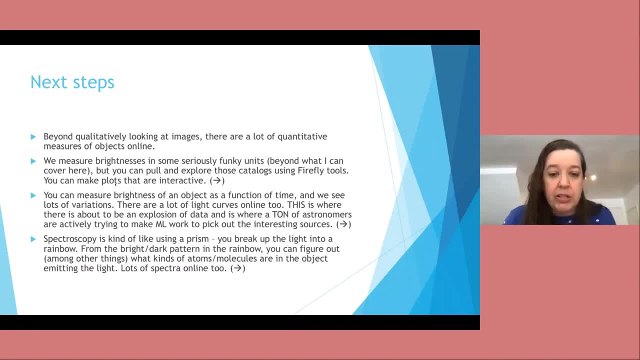 So this one in particular is a bright red baby star. You can measure brightness of an object as a function of time. Most people probably think of astronomical objects not changing very much as a function of time, but you can see lots and lots of variations. 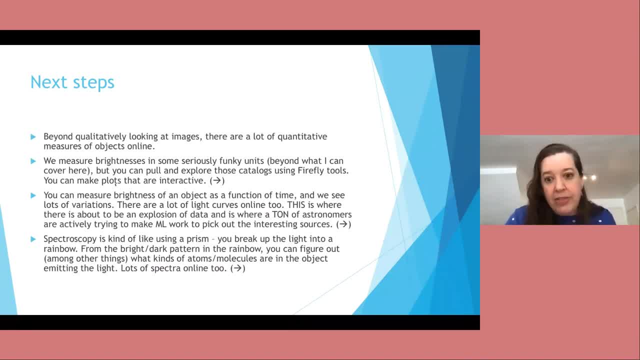 And this is where there's about to be a true explosion of data, And that is where astronomers are actively trying to make machine learning work, because there's gonna be so much data that there's no way that any person can put eyes on each set of data. 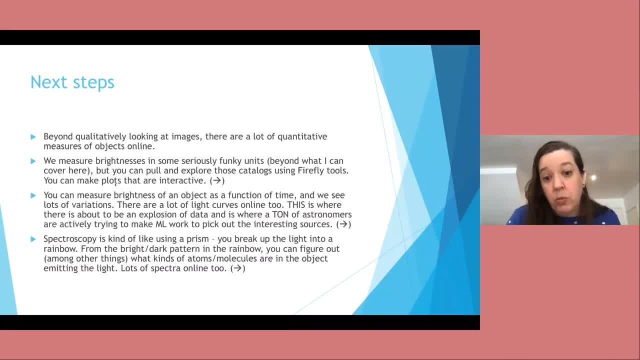 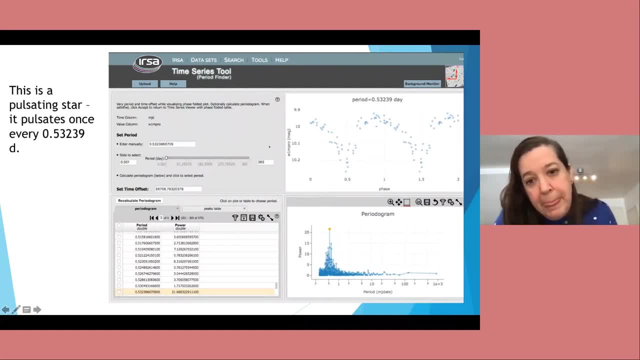 And so they are actively working, trying to make machine learning work, to find the interesting sources. So this is an example, again using the Ursa tools- This one is called Time Series Tool And this is brightness as a function of, in this case, phase or period. 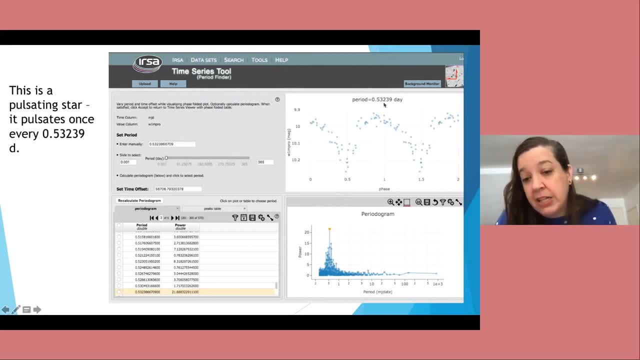 This particular thing is a pulsating star. It pulsates once every half a day And this is the time series analysis. If you're familiar, it's called Lohms-Gargel or it's an adaptation of Fourier analysis. It's looking for repeated patterns in the data. 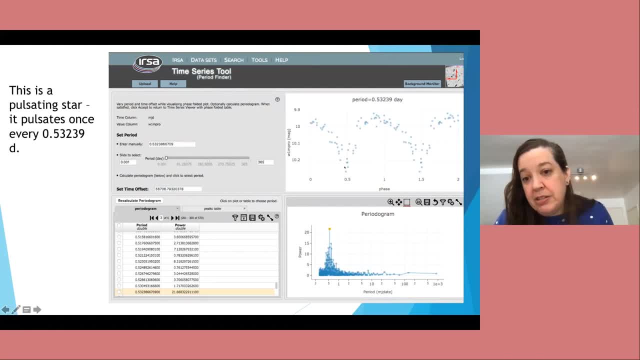 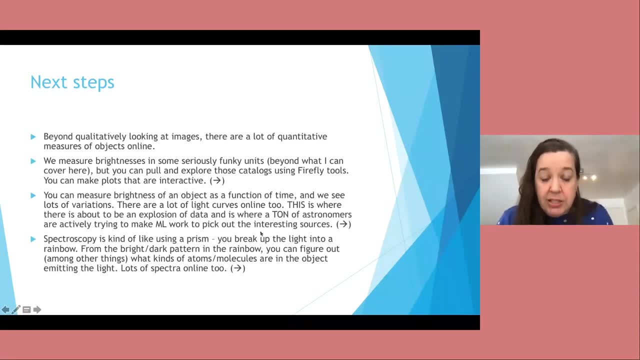 And so there's a repeated pattern at 5.3 days. that is coming from the fact that the star is pulsating And so it's changing brightness, And I swear retconoscopy is kind of like using a prism: You break up the light into a rainbow. 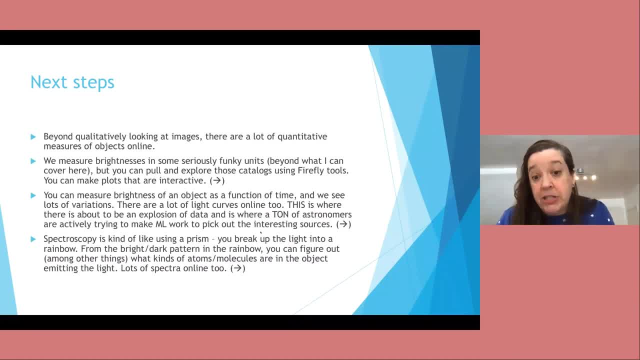 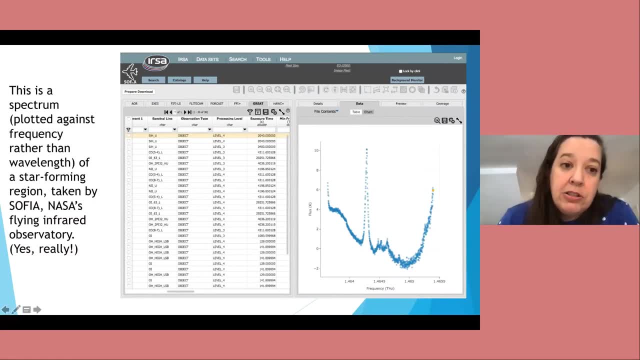 and from the bright and dark pattern in the rainbow you can figure out, among many other things, what the object is made of, And so there's lots of Spectra online too. This is again using Ursa tools. This particular archive is called SOFIA. 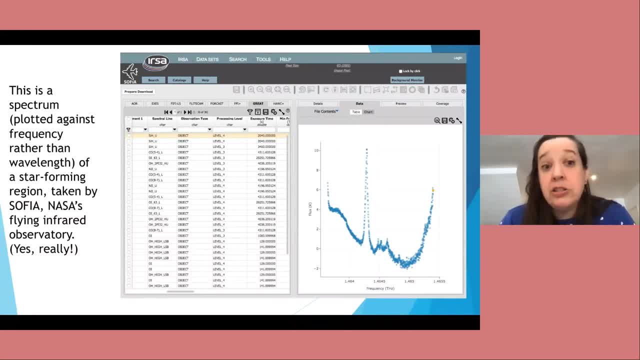 SOFIA is a NASA plane. It literally has a hole in the side that a telescope looks out from. I am not making this up. This is really a NASA facility. a telescope on a plane can look out, And this is a spectrum. There's brightness as a function, this time, of frequency. 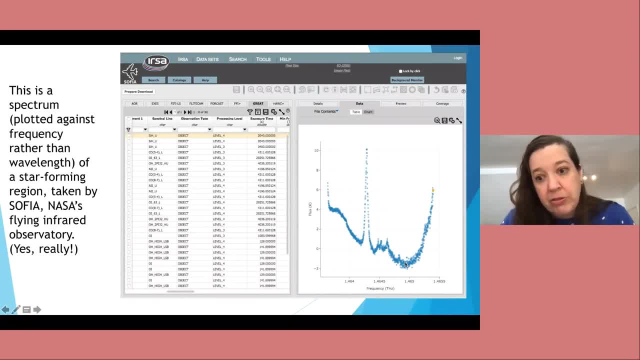 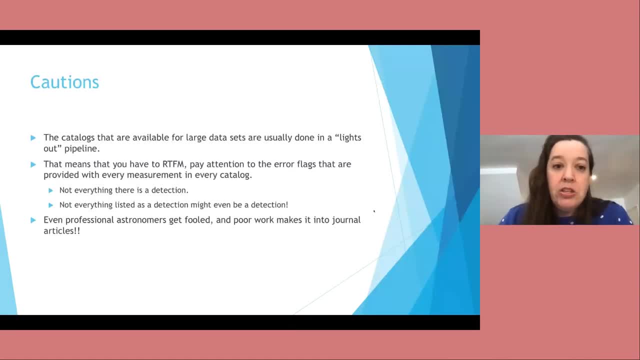 rather than wavelength, And it's a spectrum of a star forming region And this is an emission line that is being emitted by some of the hot dust that's in the star forming region. So the catalogs that are available that you're accessing through these tools are usually done. 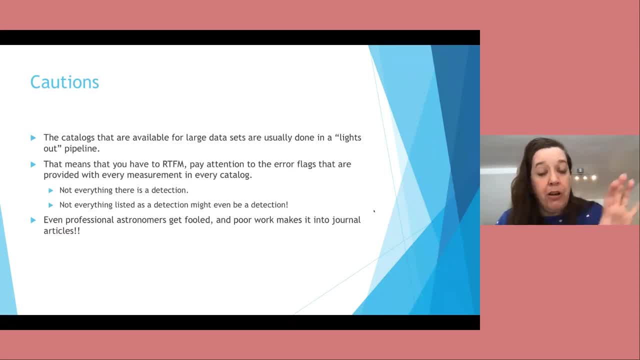 totally lights out pipelines. So in other words, there's no human involved, The pipeline just chews away. But that means that you really do have to read the documentation. You have to pay attention to the error flags that are provided, Because not everything there is a detection. 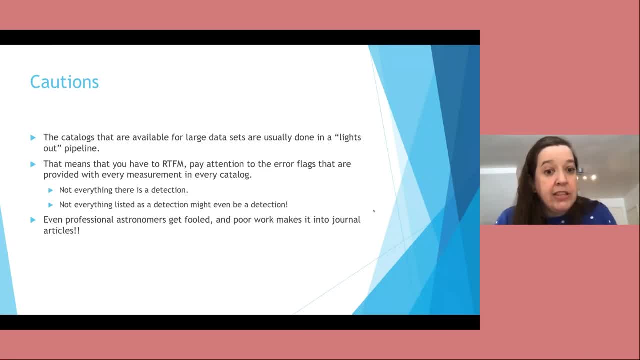 Even if it's in the catalog, not everything there is a detection And not everything that's listed as a detection might even be a detection, And even professional astronomers get fooled by this And wrong work makes it into journal articles. So this is finder chart, but for a normal point. 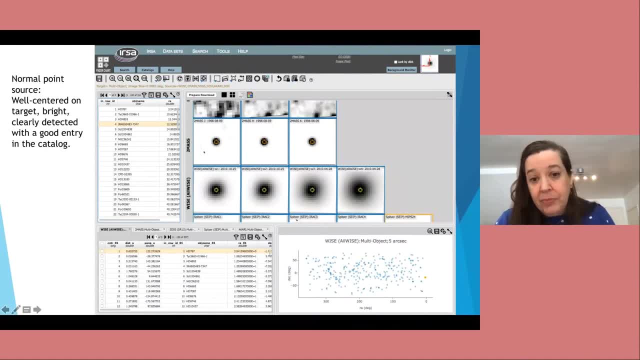 source. So I've got a list of sources here on the left And I've got this one individual source shown here And it's just a blob right. It's a point source. at all of these wavelengths, The reason the point source is looking like it's getting. 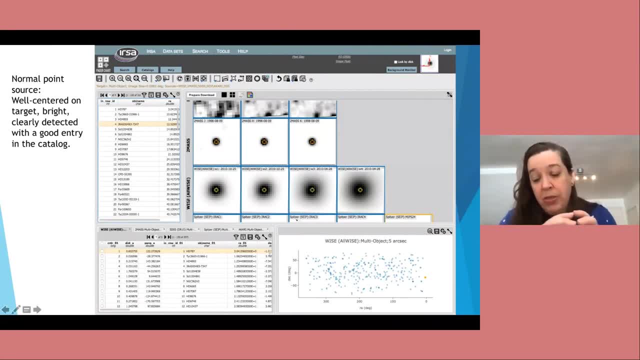 bigger is because the telescope is the same size on this row, but the wavelength is getting longer, So the blob gets bigger. It's just the way the physics works. So this is a bright point. source: Totally normal, Totally good detection, All makes sense. 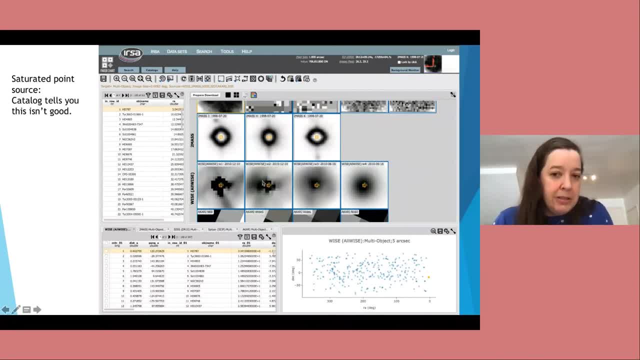 This one looks like a donut, But it's not a donut. The source is actually so bright that it's effectively temporarily damaging the pixels. You know how, like when someone takes a flash photo of you and you sort of get an afterglow, you get sort of spots in your eyes. 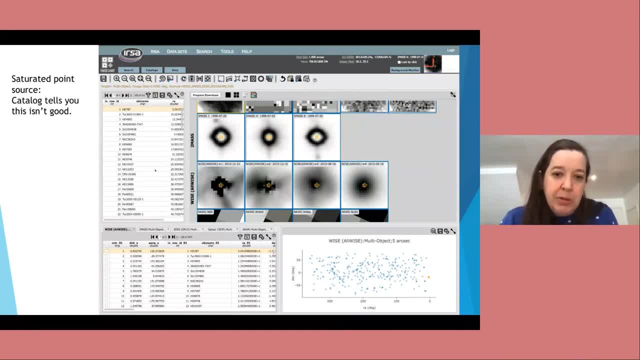 That's what's happening. The source is so bright that it's temporarily blinding the telescope at the core of the source. So I'm not going to name names, But there is a paper that's been published in a research journal talking about: oh, they found this new category of Y sources. No honey. 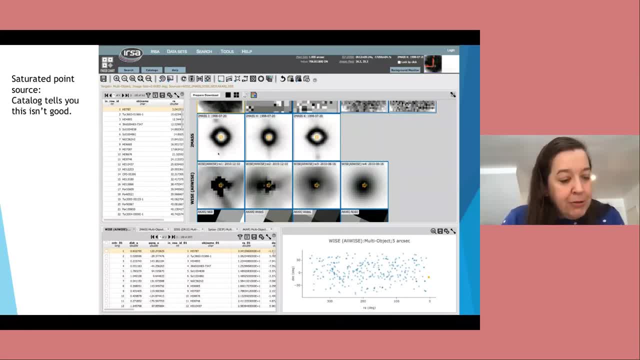 They're saturated. You know, this is what happens: if you just grab the catalogs and you don't look at the images, You can shoot yourself in the foot, Which these people did, Okay. So, even though it seems boring and counterintuitive to look at images by hand, as opposed to writing lots of Python code to pull the 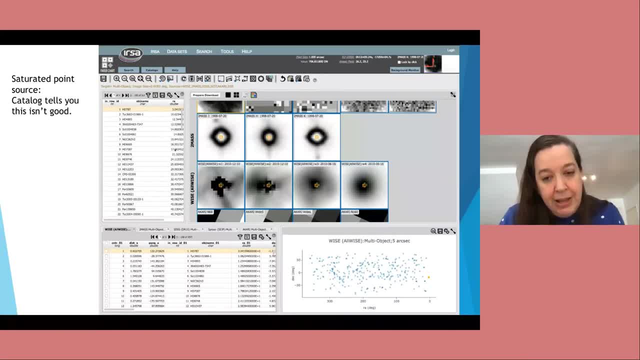 catalogs. please hear me when I say it's always useful to look at at least some of the images to make sure that you have not fooled yourself, Because the catalogs are going to be so good. And I want to show you this Because the catalog does actually tell you in the data that it's. 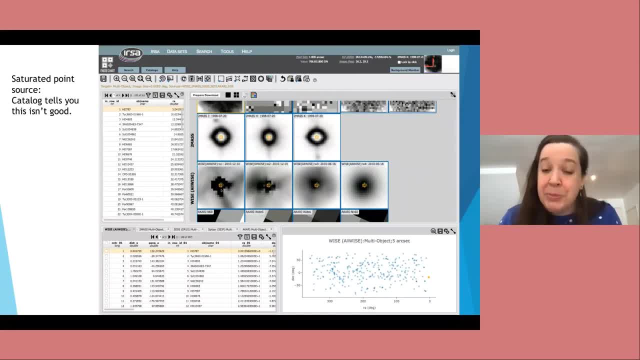 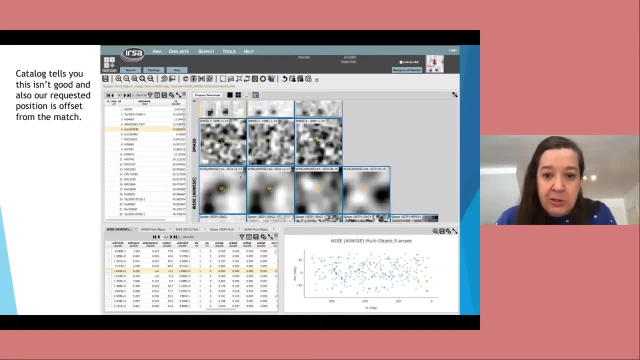 providing. in these columns down here, it is actually telling you that the source is saturated. But if you don't pay attention to those error flags then you don't know that they're saturated. Here is a source- Whoops. Here is a source where the catalog has told us that the measurement is 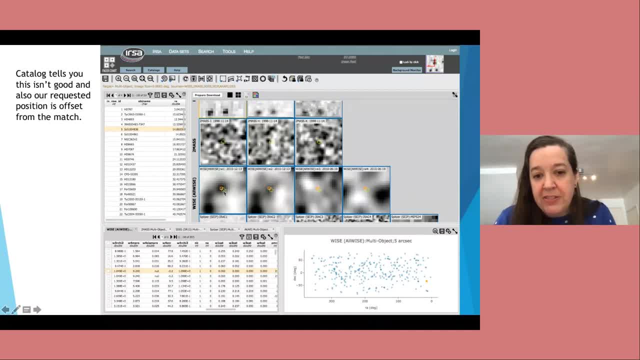 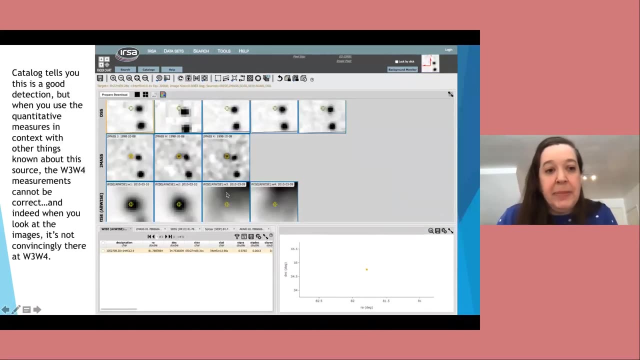 not very good, And you can kind of tell that because the source that it's returned is offset from the position that we asked for, And so it's very, very faint in the near-infrared, probably not even there there, and it's not the same as the source that you can see here, but it's offset. Here's another. 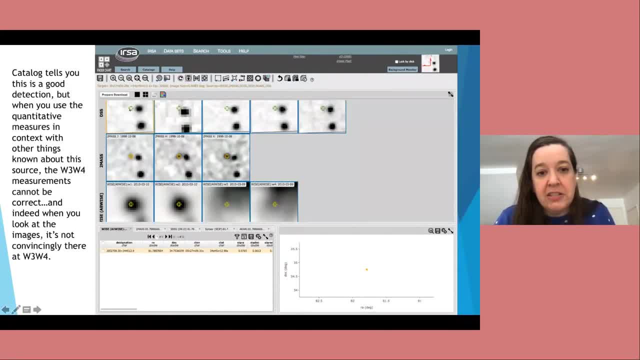 one where the catalog tells you it's a good detection because here's the source that crosshairs is the source that we asked for and it's barely visible in the optical. It's coming up fast, It's clearly there by k. It's barely there at j, which is one micron, and k is 2.2. 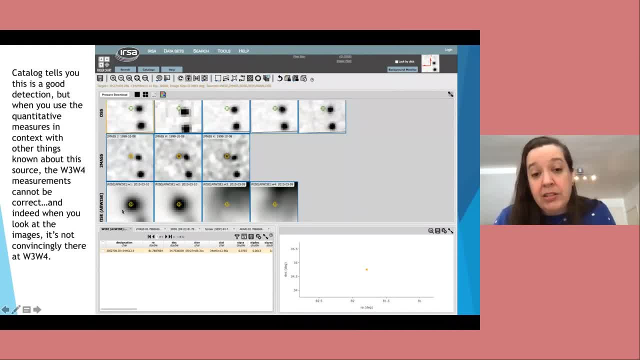 microns. so it's clearly there and at the shortest two wise bands. it's there and the catalog lists this as a detection at these two bands. but when you look at the actual quantitative measures that the catalog gives you for this source, the values that it tells you for, 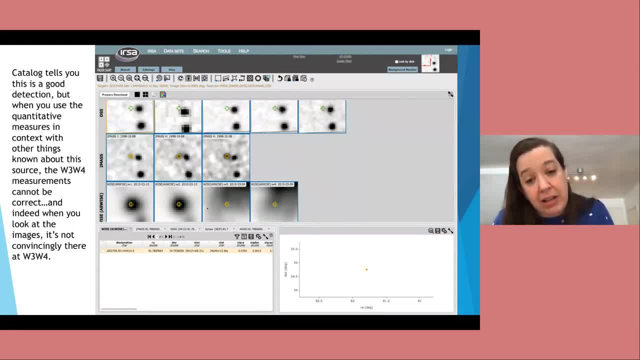 wise three and wise four cannot possibly be correct because they just look wrong. and when you actually go and look at the images, indeed, the source is clearly there, but when you look at the data, it's not there at wise one and two, but probably not really there at wise three and wise. 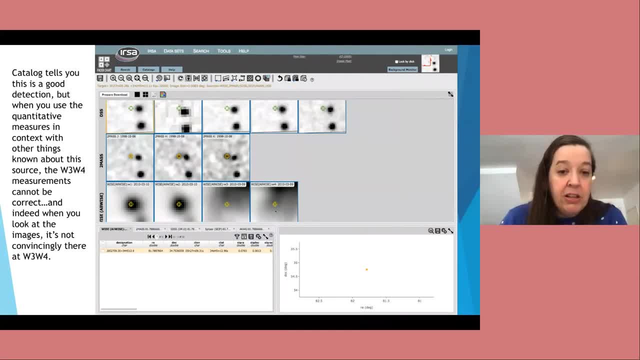 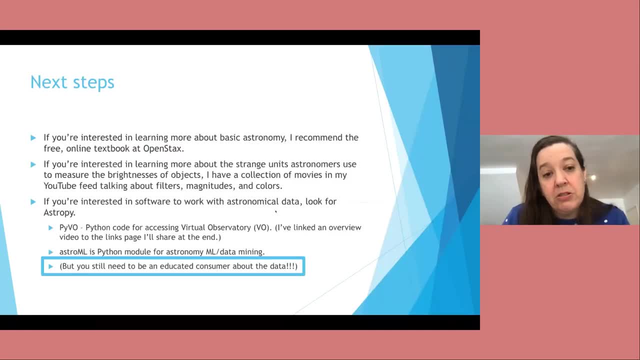 four. so I really want to emphasize that even though y'all are really experts at the pulling large quantities of data and doing lots of machine learning things, you do have to be careful because you can shoot yourself in the foot. so if you're interested in learning more about basic, 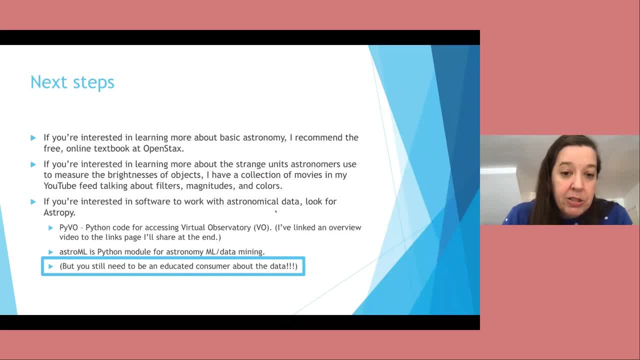 astronomy. there's a free online textbook at OpenStacks which is pretty good. If you're interested in learning more specifically about these funky units that astronomers use, I've got a collection of movies in my YouTube feed. If you're interested specifically in software to work with astronomical data, you should look for. 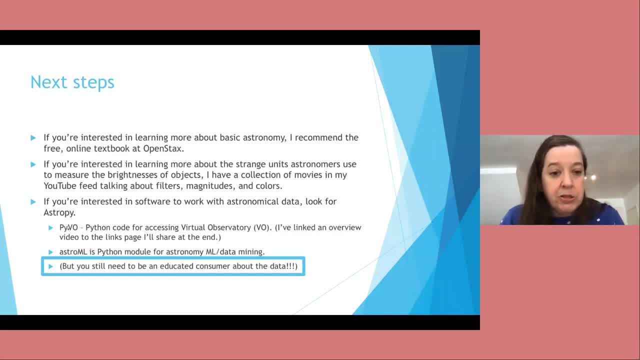 AstroPy for this huge library and community of astronomers using Python. It's enormous. PyVO is specifically Python code for accessing observatories through the virtual observatory protocol, so you can access different archives from many different telescopes using the same interface, and so I've included an overview video on the links page I'll share at the end. 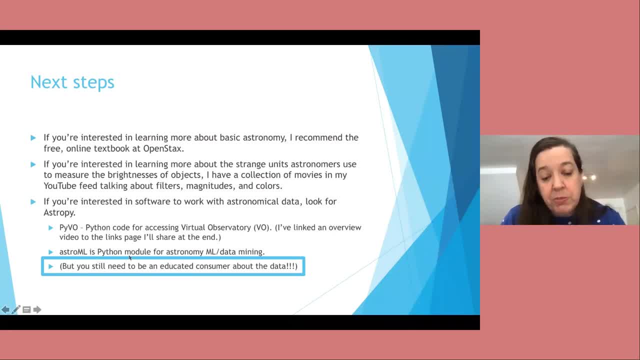 The machine learning. the AstroML is a Python module specifically for astronomy, machine learning and data mining, but I want to emphasize again, you still need to be an educated consumer about the data. You still need to read the documentation to understand what it's telling you about what you can believe and 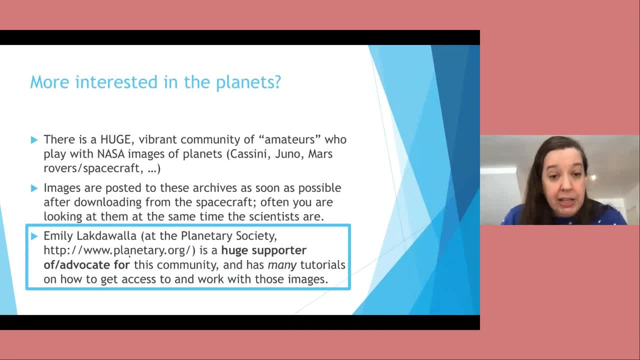 what you can't If you're more interested in doing planetary data. there's a huge, incredibly vibrant community of so-called amateurs who play with lots of NASA images of the planets. so we've got, NASA has and continues to have, several spacecraft that are in deep space, in other words, 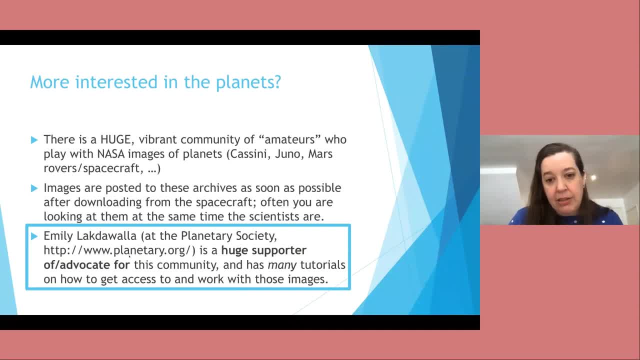 well away from Earth and they beam back data that, for a lot of these missions, are made public to you, the public, at the same time as they're made available to the scientists. So the Mars rovers that are up there right now download data every couple of days and they get. 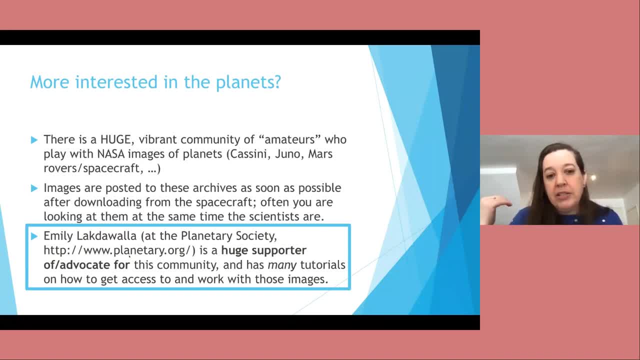 posted to the archives as soon as the data get processed, but you're looking at them at the same time as the scientists who requested those data. So if there's a Emily Lakdawalla who used to work at planetary society but her blog is still up, she's a huge supporter of this community. that. 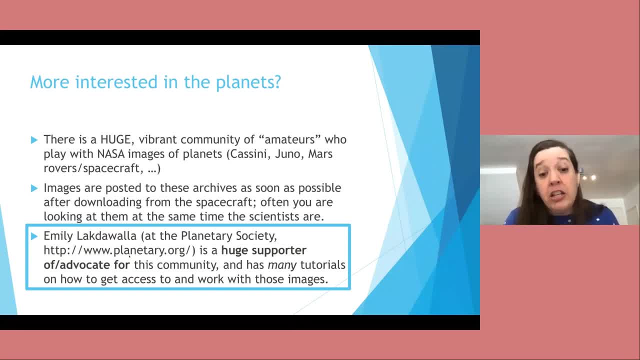 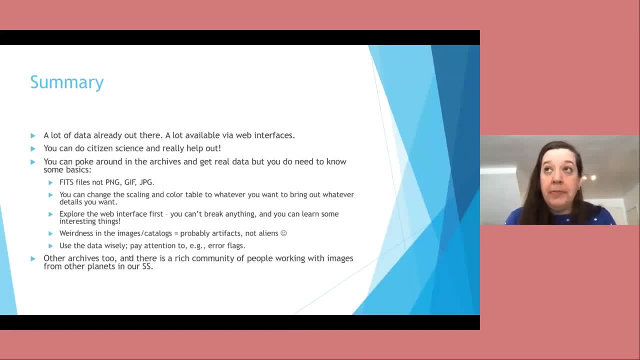 works with these nasa planetary data, and so she's got tons of tutorials of how to access those data, how to reduce those data, how to process those data. so, um, the summary of the main points that there's a lot of data already out there and there's a lot that's available via web interfaces and you can in. 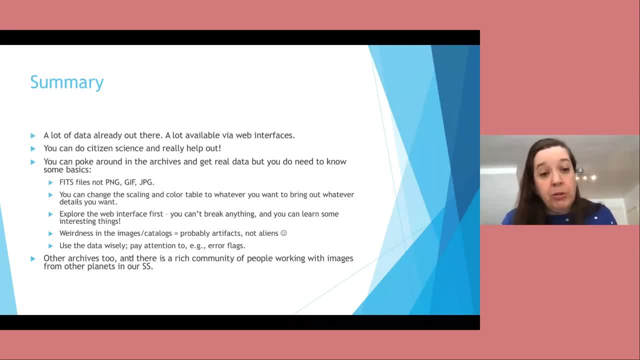 fact contribute to real science, these citizen science programs. you can poke around in the archives and get real data, but you do need to know some basics, like the fact that you're using fits files and you can't use gifs or jpegs. you can change the scaling and color table to whatever you 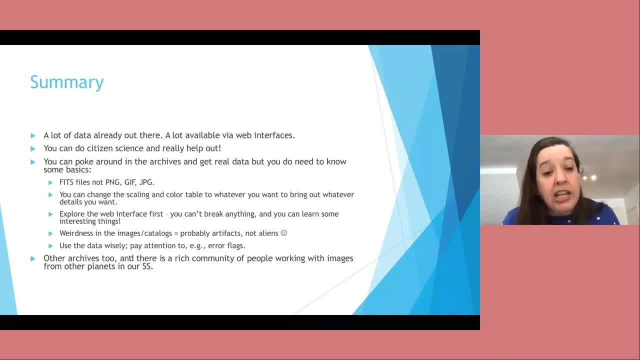 want to bring out whatever details you want to see in the image. i highly recommend that you explore the web interface first before jumping into code and get used to what sorts of weirdnesses you might see in the images and catalogs and the fact that they're not aliens. it's just artifacts of the 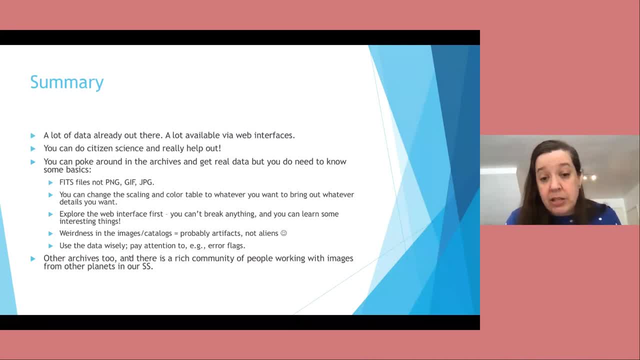 data collection and you need to use the data wisely. pay attention to what the catalogs are telling you about whether or not that data point is believable. there are tons of other archives and a rich community of people working with the images from other planets in our solar system, so i went through a lot and your brain is probably fried. 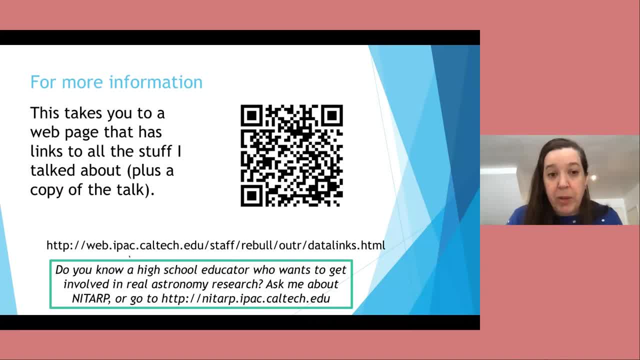 so i'm going to leave this up for at least a little bit before i go back to a live demonstration, because this is the link to a web page that has all of the stuff i talked about, all the links that i mentioned, all the videos i mentioned. all of that stuff is linkedin, and this qr code: 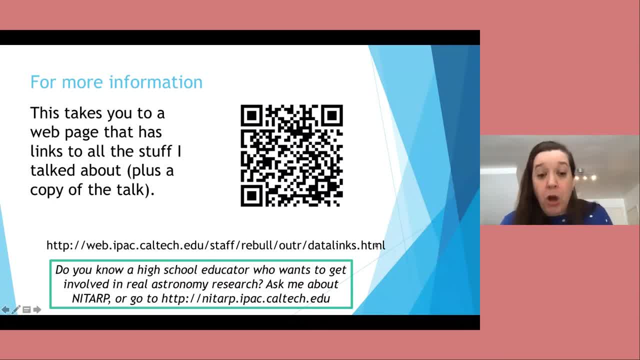 takes you to that website and if you want to go to that website, you can go to that website. and if you are or you know a us based high school educator who wants to be involved in real astronomy research, i want a program called night harp, which is the nasa ipac teacher archive research program. 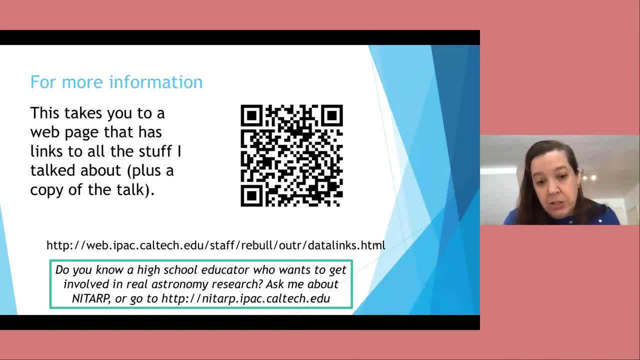 and that we work with high school- largely high school teachers to do real astronomy using real data. it's a year-long program and we're about to put out the application for 2022.. so i'm going to leave this up for a couple more seconds for people to take screenshots or write down the link. 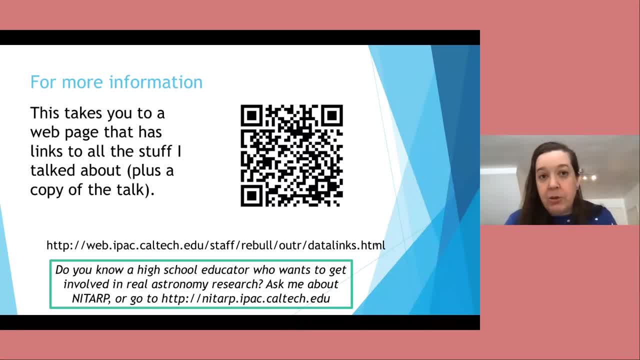 or whatever you need, and then i will take any questions you have. but i'll also go back to doing a live demonstration for as long as you guys want to listen. let me- hopefully everyone's got that link. you know what? i can probably put it in the chat. let me copy it and put it in the chat window. 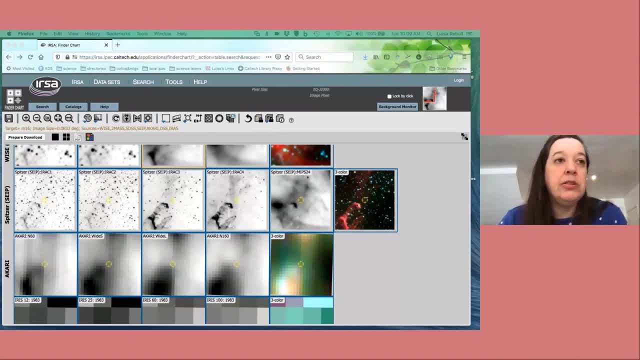 okay, so there's the link that i've put in the chat window. are there questions that you guys have now, or do you want me to just go back to showing you some of the other cool things that these tools can do? i have put everyone to sleep, sorry, go ahead. i don't see any questions yet. so if you want to do, 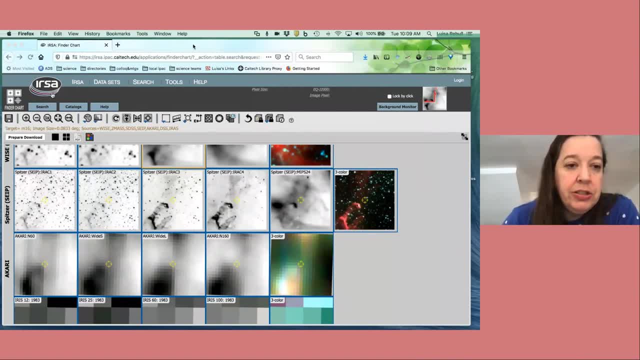 um, you know another demonstration, sure, sure, okay, so on the main ursa front page, if you put in um the, you know the name of an object that you like, m101 is messier 101, so it's from that catalog that i mentioned, where the guy was assembling the list of things that aren't. 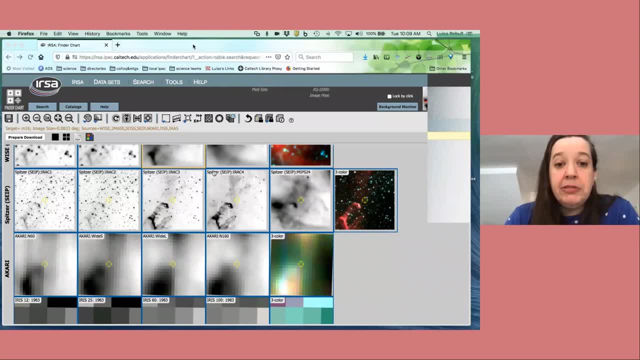 comets and 101 is a beautiful spiral galaxy, and so its images are quite, can be, quite pretty. it's the kind of thing that you see everywhere, because it's a beautiful something called the grand design spiral, so it has beautiful spiral arms- this particular image that's in the background here. 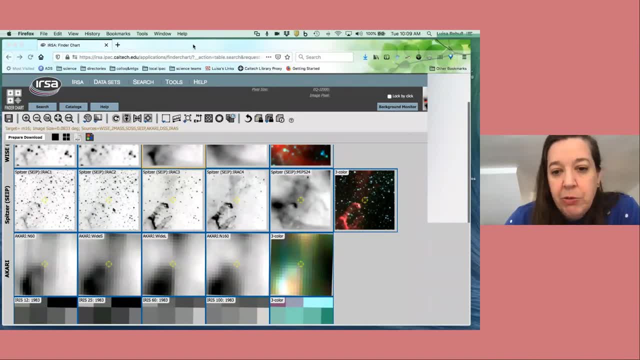 is not very pretty, but it's trying to give you an idea of where you are in the sky with respect to other objects. this is giving you an overview of the image that you're looking at, so i'm going to show just a little bit of a preview here of the property that it's all set on now. 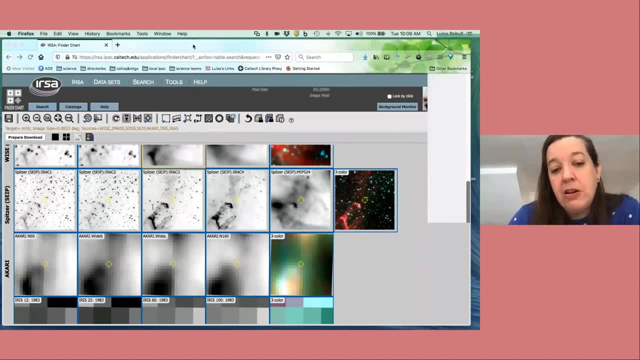 i'm going to show a little bit of an overview of brightness, basically as a function of wavelength, but what i want to really emphasize to you is this is all the data sets that it found that overlap, that position so wise, for example, goes: uh, because it is an all-sky survey. it's. 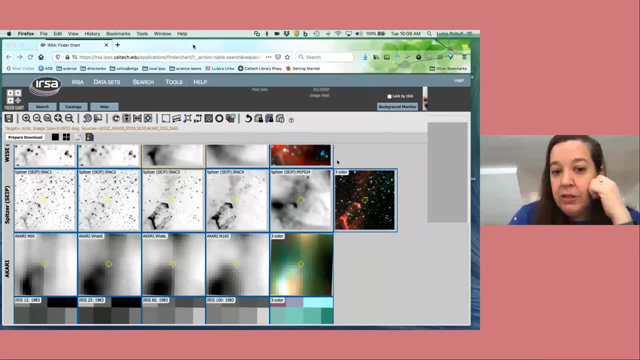 going to come back with almost every, every position you can put in. if you click on to ursa viewer, then so it found one source at that location and it's going to pull an image. so there, if you can, you can drag the boundaries between these panes so you can see it's pulled just a tiny chunk of sky and 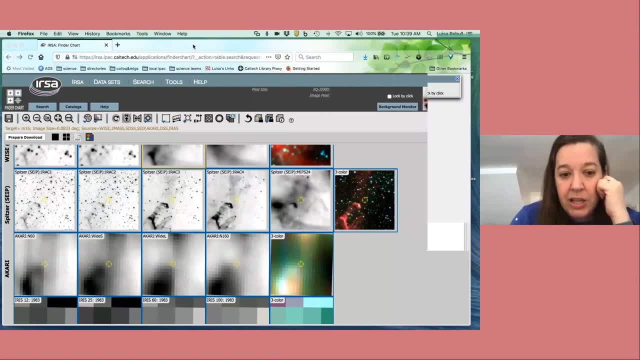 it's not terribly dramatic. you can kind of see the spiral arms. let's pick um instead of catalogs. let's filter this down. so we're just looking at images filter. so now we just have images. so let's go to the two mass large galaxy atlas here and let's go down and say: okay, i'd like to get the. 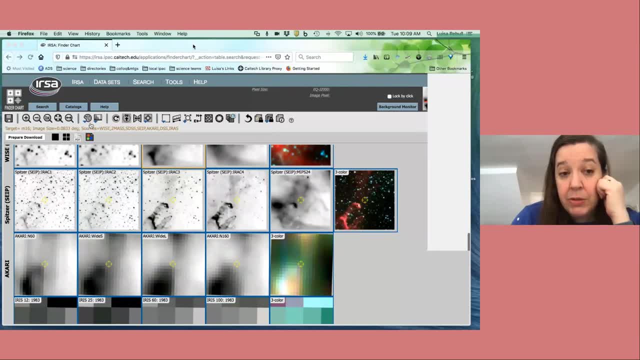 k-band image. if i click on this it'll download to disk, but i'm going to click on this, which will load it into the ursa viewer over here. okay, that's not terribly impressive. i don't know what's going on with that. um, fascinating something. something's not right. 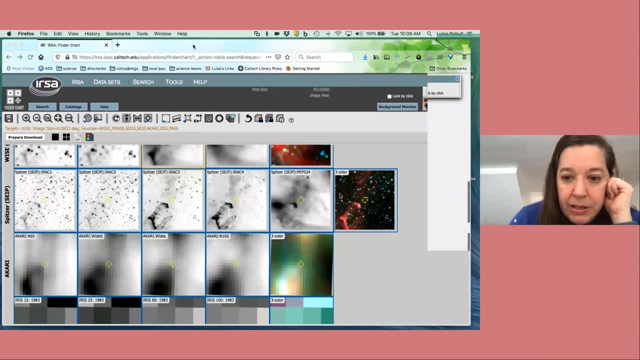 okay, let's go back over here. um, let's pick, uh, wise images. so this one is technically a wise specific archive, and so it's pulling the same little chunk of sky in just the four wise bands, and so you can see there's lots of background stars at the shorter wavelengths and fewer of them at the longer wavelengths. that's. 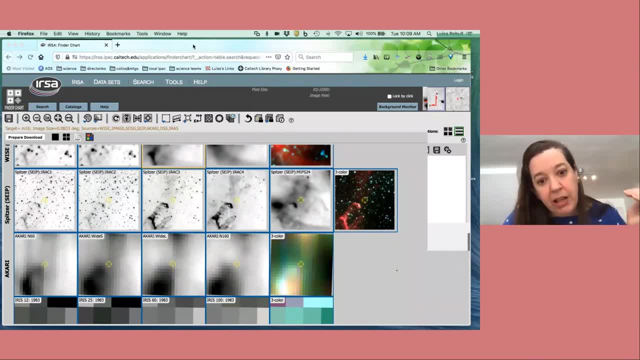 real astrophysics, because the stars will be brighter at shorter wavelengths than longer wavelengths and the dust will come up. so that's a pretty nice thing to have. so let's go back over here So you can start to see there's more texture in the galaxy core there. 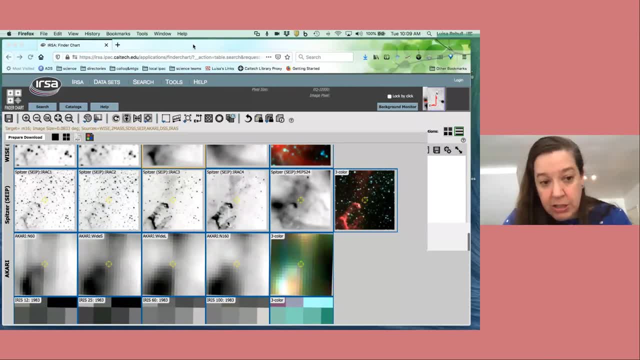 than there is at the shorter wavelengths when you go to the longer wavelengths, cause you're looking at more dust, Let's look at, let's see. I think crucial should give us some cool results, Let's see. So let's get, let's get, yeah. 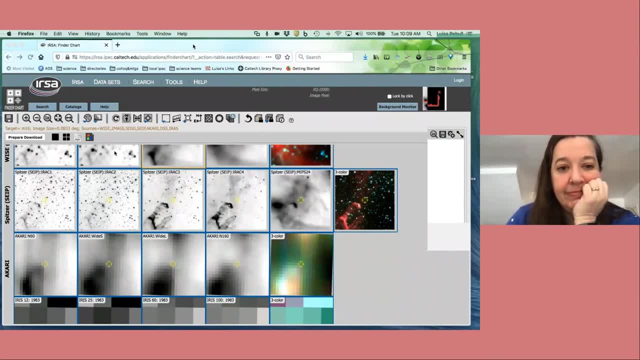 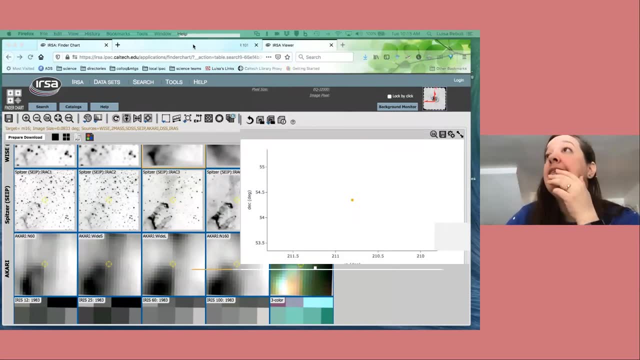 One thing is: I wonder, if you turn this camera off, there's still a delay on the screen. I'm just wondering if I can see a little bit faster. We can give it a try. Oh yeah, yeah, Maybe we can do that. 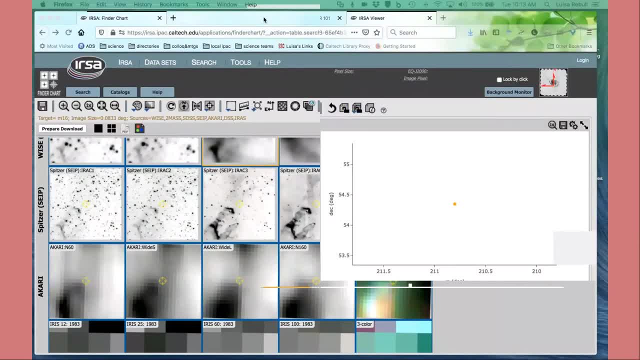 Just turn the camera off. Yes, let me do that. Okay, And there's one question that somebody had: which programs, ideally free, can handle the fixed images? Sorry, I lost you at the end of that. Which programs are what? I'm sorry. 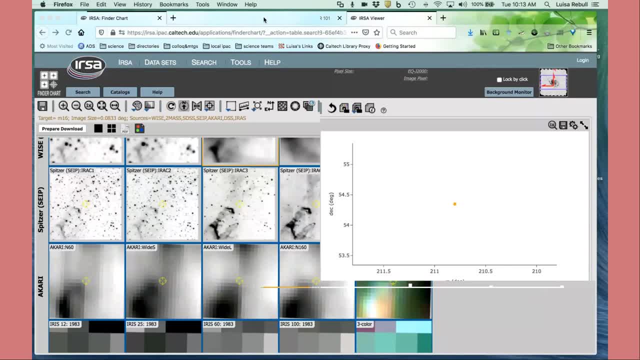 Which programs, ideally free, that can handle the fixed images. So there's lots of modules in AstroPie that can handle the images. These tools, these URSA tools that I'm showing you, that are all based in Firefly, can also handle the fixed images. 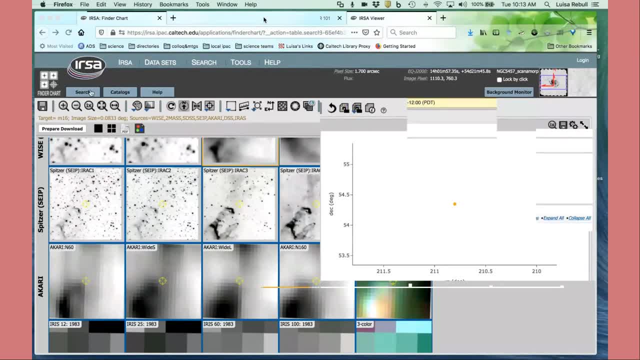 so you can load them in right. So if you wanna, if you click on image, one of the choices that you can load is an image from your disc, or you can pull an image from elsewhere on the web right, Or you can search within URSA's holdings to get more images. 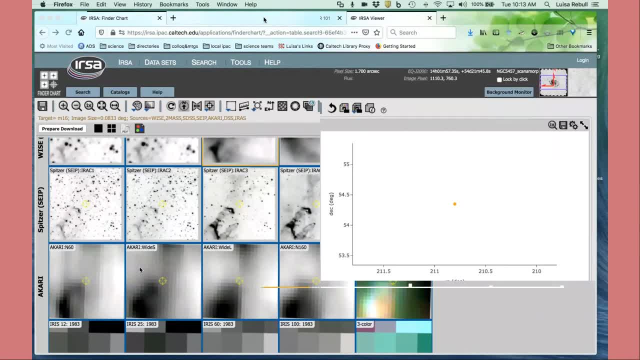 So the URSA. URSA tools can handle fixed images and so can a lot of the AstroPie modules. There's also a tool called DS9, which is it's written by Harvard and it will allow you to load in images. The URSA tools give you more interactivity. 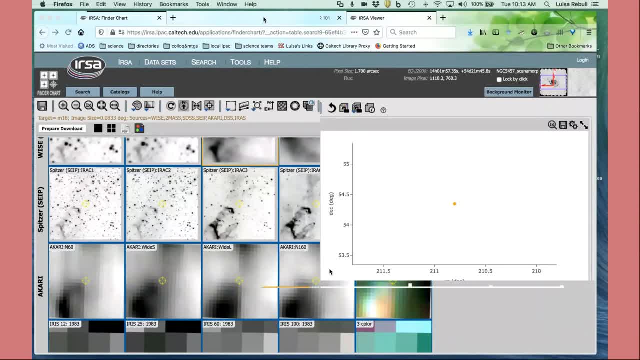 with the catalogs and the plots. DS9 is focused just on the fixed images, Anyway. so here this is a 70 mic, no 100 micron image, And so you can see lots of the the clouds of dust and gas in this spiral galaxy. 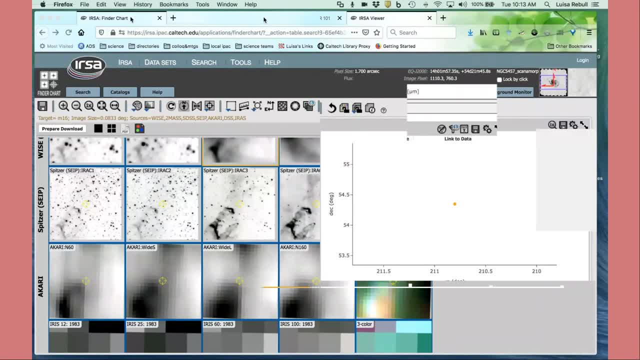 I'm sorry, the lag is making it difficult. Let's go back over here. If I pull up, let me do something a little different. So if I go to the back to the URSA homepage, if I go to catalogs- which is one of the best tools- and let's see what the differences are, 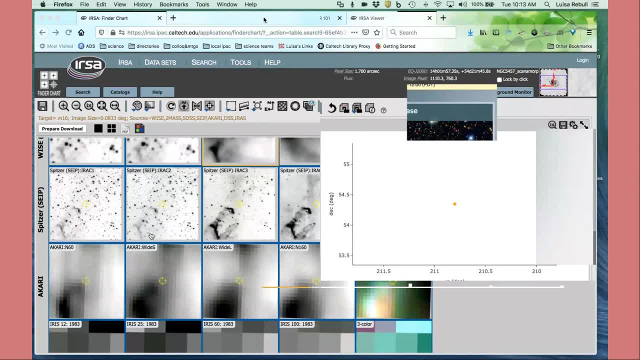 Let's go to catalogs, which is one of the best tools, and let's see what the differences are: big red buttons on the front page That'll give you access to a ton of catalogs. First you have to pick sort of the project that it's. that is part that you know whose catalog you want and 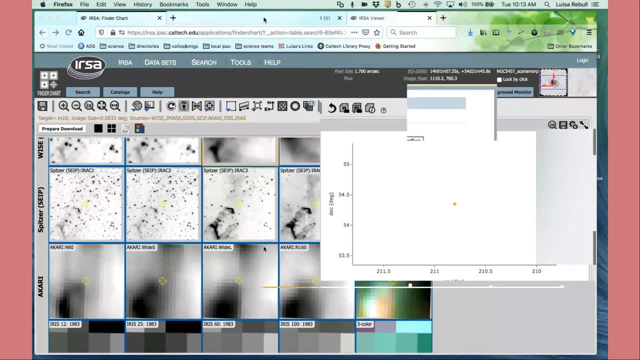 then you have many, many, many different catalogs, usually in each of these projects, to choose from. In this case, I'm going to choose something called the multi-epoch photometry table where it's going to use, because the the spacecraft observed the same chunk of sky. 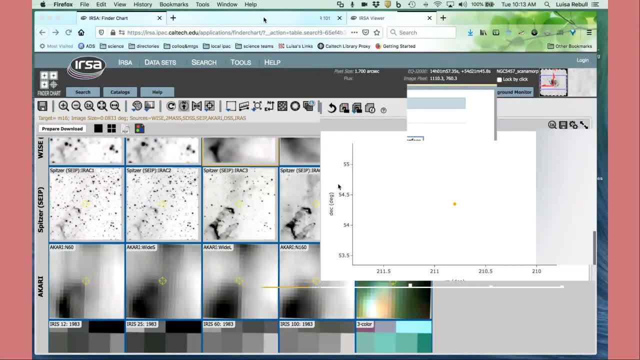 many times, and this is going to give us the individual brightnesses from each of those exposures. So our Lyra is a known pulsator and so I'm going to go let it pull the data. Come on. There's a block time on right now, but this: 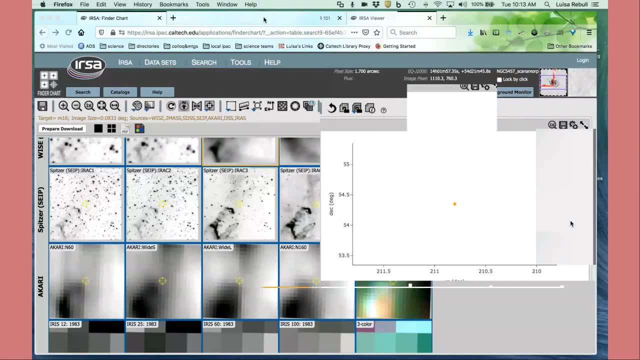 should still be working. There we go. So it found 49 individual observations of this star. Now there's a button here that's shown up that didn't show up on the other searches. This is two time series tool. If I click on the time series tool then it gives me an opportunity to 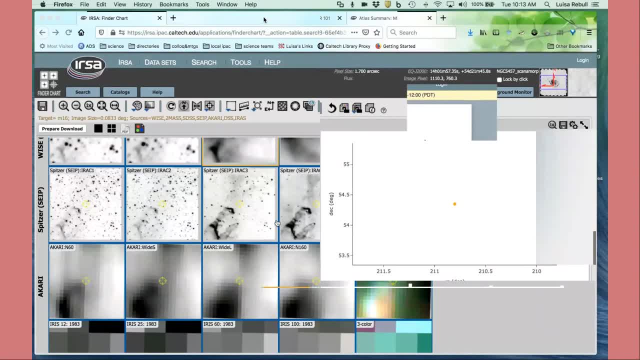 click on the source and then it's going to load it. It should load it. It doesn't look like it, but it's going to load it. Let's try it again. Let me get rid of this. Get rid of that. Try it again. 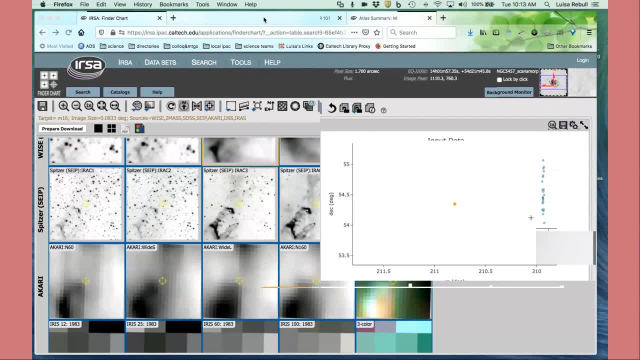 Okay, so it. the spacecraft visited this part of the sky in two different chunks, separated by six months, and if I go to this tool here that says period finder, that's doing that, looking for repeated patterns in the data. So if I can interactively come on, 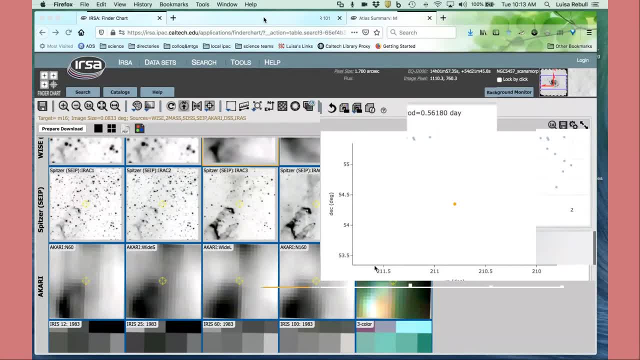 play with different peaks in this, and this star is pulsating at around half a day and I can choose different peaks and have it phase up the data. So what it's doing? let me use the peak again. Let me go back over here. So this is the original light curve, where this is brightness as a function. 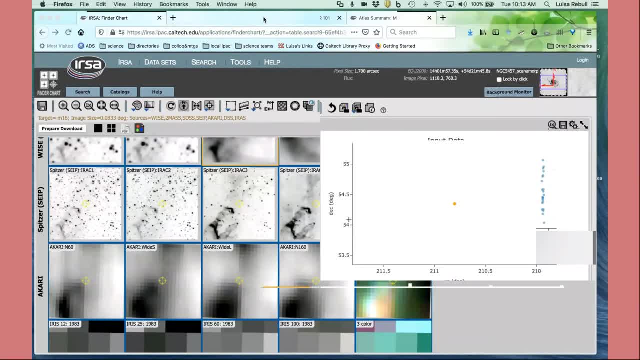 of time and the spacecraft visited it twice, six months apart. so I can, you know, zoom in on just a piece of the plot and start to see that there's more variations there. but what i've, what i did when i clicked on period finder, is i went and looked for repeated patterns and this is the strongest repeated. 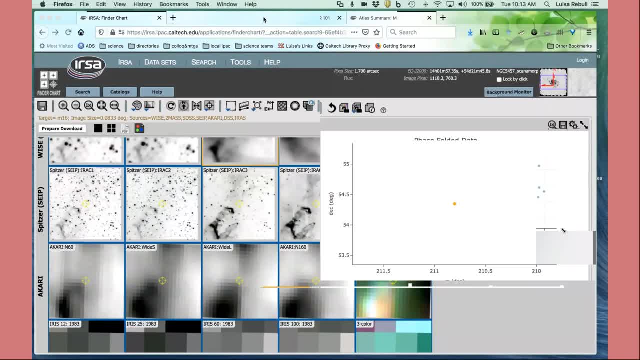 pattern. so now it's got brightness as a function of rotation phase or pulsation phase, basically repeated pattern phase. so between zero and one is one period and between one and two is the same period repeated, so that you can look at the overall shape. and so what this is is brightness. 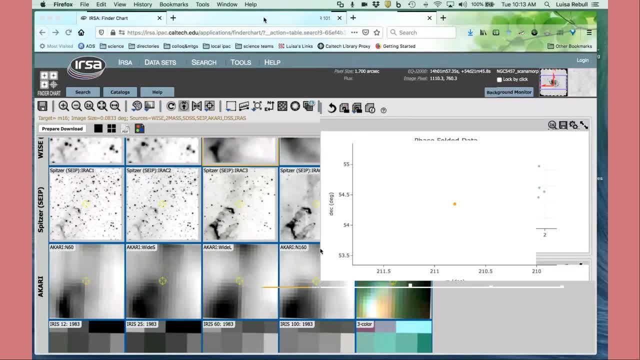 as a function of repeated pattern phase. that's why it's called phase folded um. and so when we go over here, what this is doing is saying, okay, i can represent this light curve, this, this brightness, as a function of time by a collection of sinusoids, and the most, the strongest sinusoid is the one. 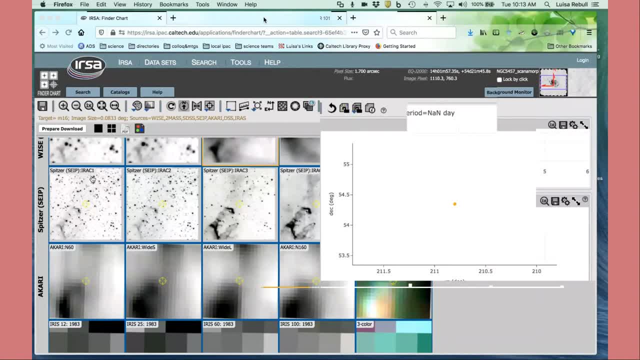 that's at point five, six, one days, so that when i go back over here here, that's the period it's going to use to phase fold the data. um, what else can i show you? um, here's the archive for sophia, which is the plane with a hole in the side. um, 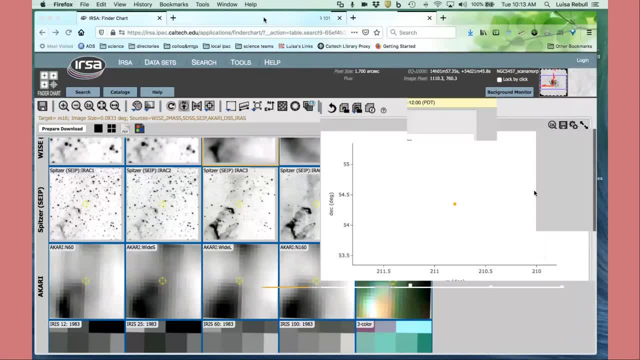 they, too, have, uh, lots of resources online to get up to speed on what, what they're observing and how they observe, but they have several different instruments. they have um, one, two, three, four, five, six, seven different instruments, um, and so i'm going to ask it to search for m17- any instrument, and it will come back eventually. 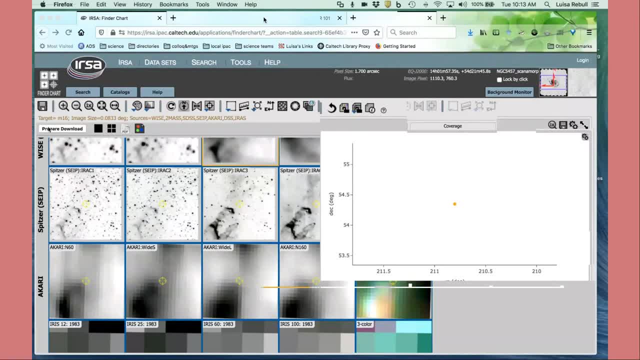 okay, so the aor tab, which is on the foreground here, this one right here. this is a list of all the observations. aor is astronomical observation request. okay, so then these are all the observations that we're going to look at, and then we're going to look at the. 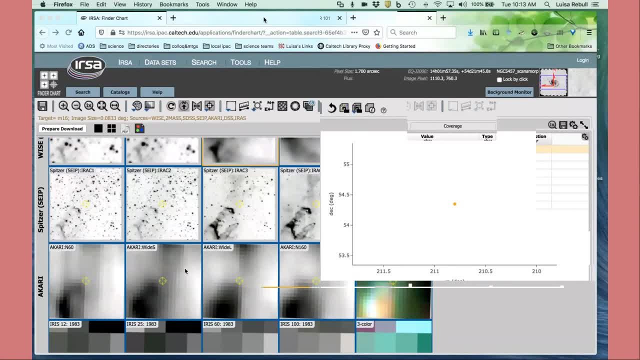 observations that it found of this region using four different instruments. and if i go to see forecast as an imager, if i go there and go to the data tab over here, that's the individual image that goes with that observation. but there's lots of spectroscopy here too. these are different views. 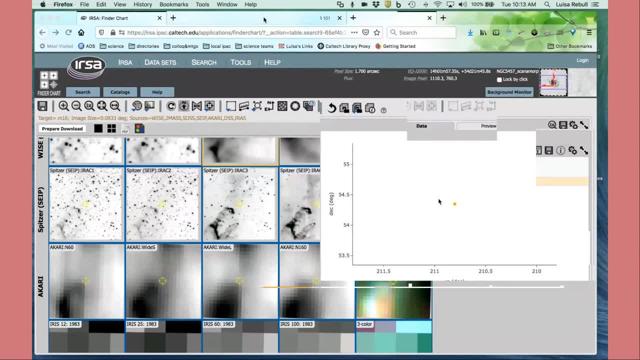 on the um, on the uh. that's not what i want. there's lots of views out on the right and that's why you're seeing stuff on the right there and everything's locked up to things. i see, and i think that's what it was um at the sixth grade. 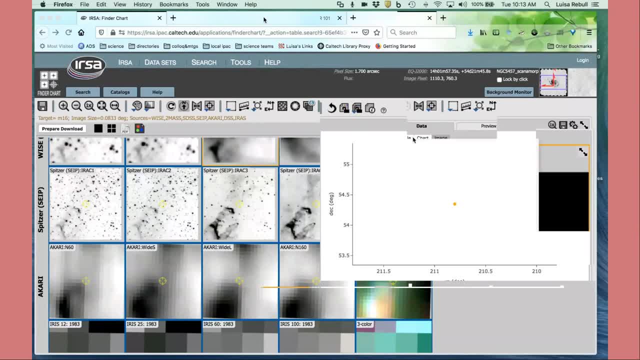 was last week i dag routine came out and that's where it's at right. so um nineton and then these are some of my favorite sources on this, but them are really useful. we all need to. um take a look: there is a lot of useless data. this is. 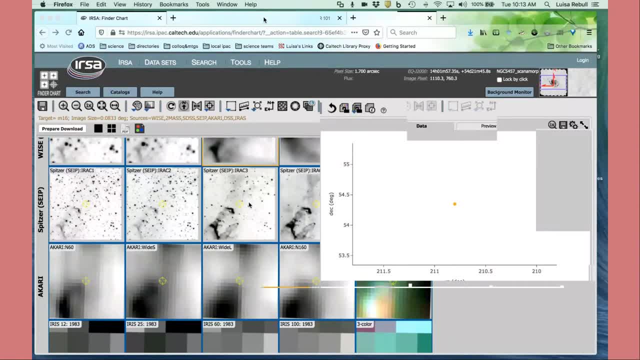 Um, the great data is sometimes very complicated. So is the Hawk plus data, Um, so it's going to try to give us the data there. There's a lot of different member. I mentioned that fits images have many different planes. This one has a thousand planes. 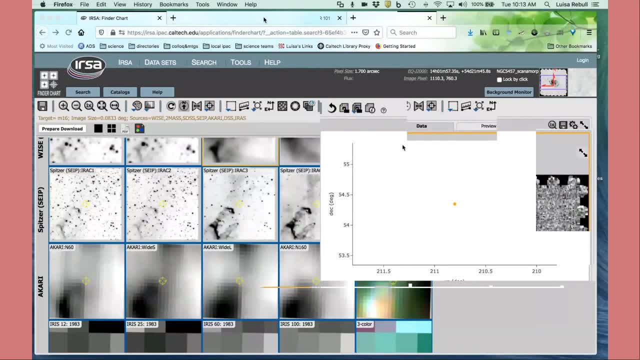 So if I type in 500, I can jump to the 500th. It's playing out of a thousand and you can start to see texture that it's seeing there. in this case, in the oxygen, one line basically singly ionized oxygen, um, and see Hawk plus has um a polarimeter. 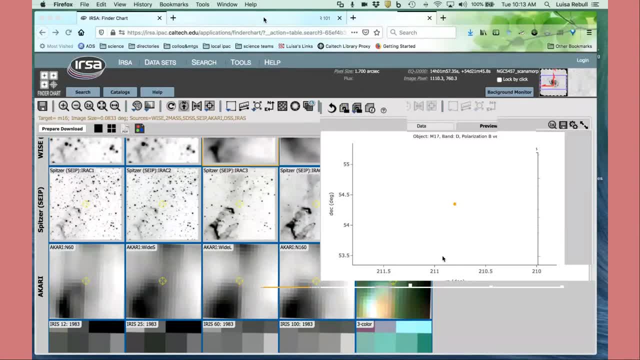 So it. it measures magnetic fields in space, And so the these data, all of those little black hash marks which you can probably barely see, are the magnetic field strength and direction On the sky, And the the background is the total flux that it's measured in this particular band. 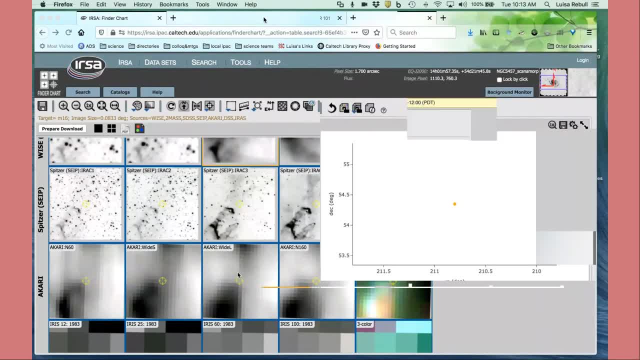 So, yeah, the data get really complicated really quickly, which is why I was recommending that you guys start with binder chart, because it's pretty straightforward and it gets you many different observations at many different wavelengths. So I put an M 17 there and turn off the catalogs. 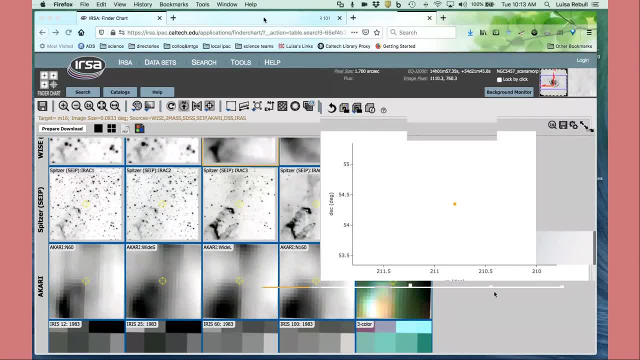 You can get the same chunk of sky at many different wavelengths. Let's ask for a bigger region than that. Let's do instead of ah, come back, Let's do a degree, Come on, All right. So the two mass image tiles are fairly small, but here at least you can get a sense of how big the star forming region is and how bright it is. 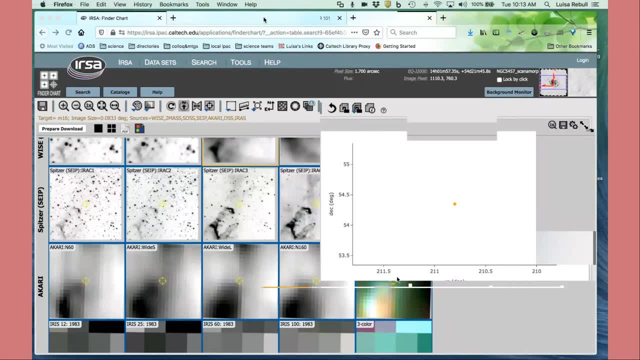 You can see it's saturated down there So it's too bright for the telescope there, but you can see it's sort of V shaped. Let's do one image at a time and zoom in. Oops, You can see it's sort of V shaped. 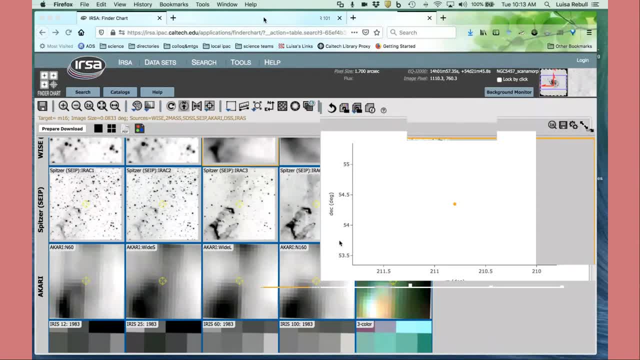 It's a star farming region that. uh, there's lots of baby stars in there. Okay, Um? are there more questions? or have I put y'all to sleep? Um, so if anybody has any more questions, now is the time to ask. 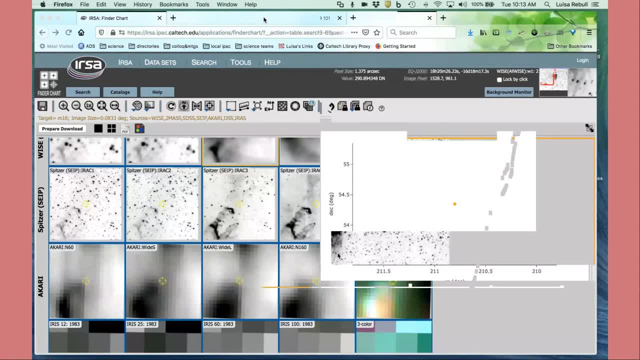 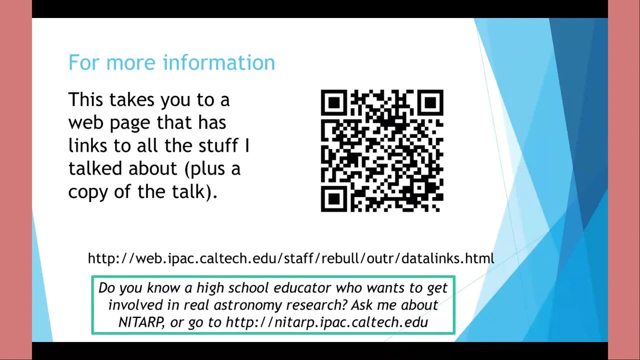 Um, and then can? we can? um- I am sorry that the lag is not cooperating- Um, let me, let me put up the slide again that had the um the webpage. that webpage has links to, among other things, the YouTube feed for Ursa, which has lots of screen capture videos, all of which are well, most of which are very short, so that you can see a demonstration of just how to read in images. 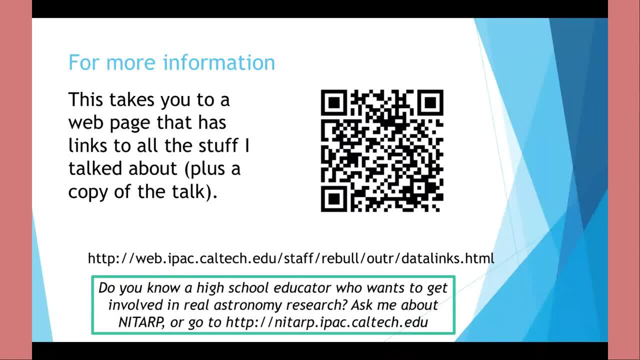 Or just how to work with catalogs And, um so those that, because there's, you know, because those videos were recorded locally on my computer, there's no lag, So I am sorry that the lag is prohibitively difficult for following what I was doing for the demonstration. 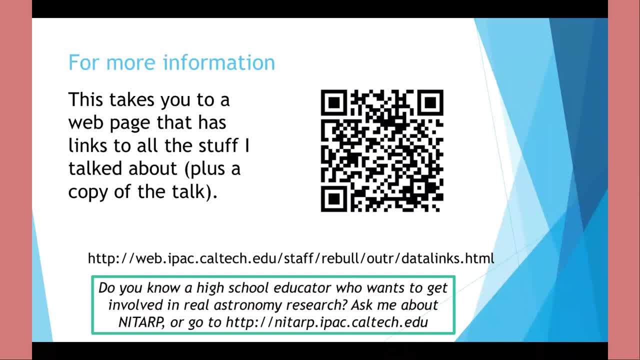 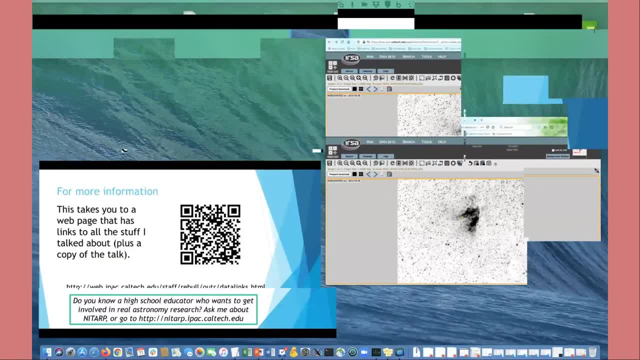 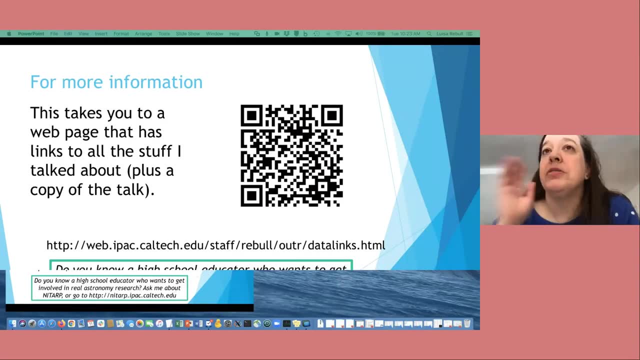 You can turn your camera on now if you want. Let me, if I put, let's see, uh, come on, Okay, so okay, Um, I don't see any more questions. So, um, yeah, maybe give it a couple of minutes if anybody has any other questions. 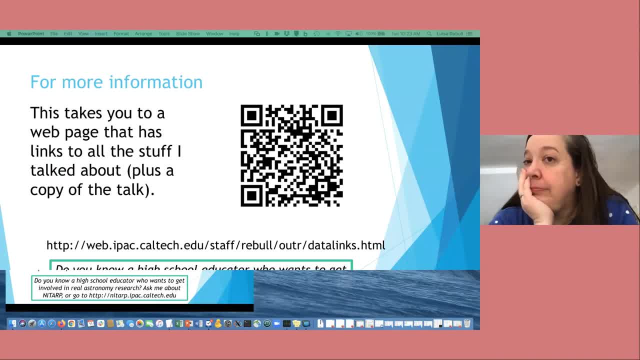 Um, but yeah, this was um. this was a great presentation and I guess we can see some of those images on the um link that you have there. Yeah, So I um, there's different, I don't know if it. yeah, I, looking at the screen that looks like it hasn't even on. 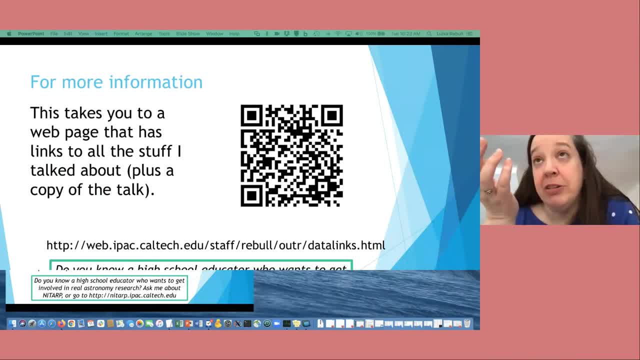 Okay, Okay. I don't know if it's the screen in the big marker interface. It doesn't even look like it's completely rendered. the image that I'm looking at right now No, And I so I'm. is it because it's the images are so large, or is it the platform?